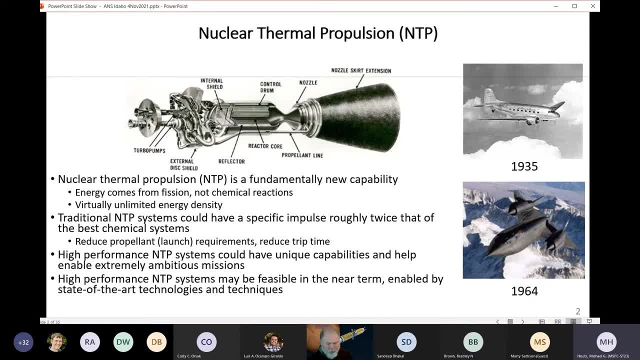 the efficiency, basically the exhaust velocity that we can get with the propellant, goes with the square root of the temperature divided by the molecular weight. So you have a strong incentive to to increase temperature and decrease molecular weight And so hydrogen, you being the lowest. 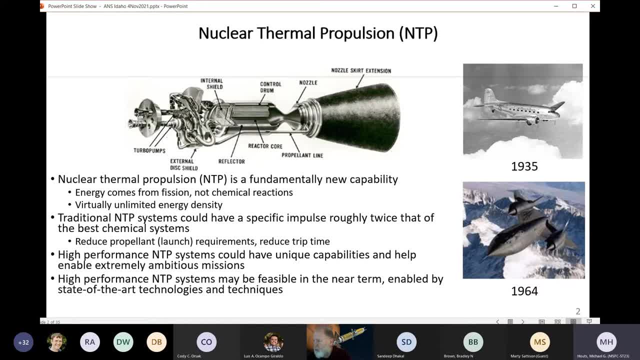 molecular weight ends up being the propellant of choice, especially for a given temperature that the engine, the nuclear fuels, are able to heat that propellant to. And then also, of course, with fission, we have essentially unlimited energy density. We do actually bump up against. 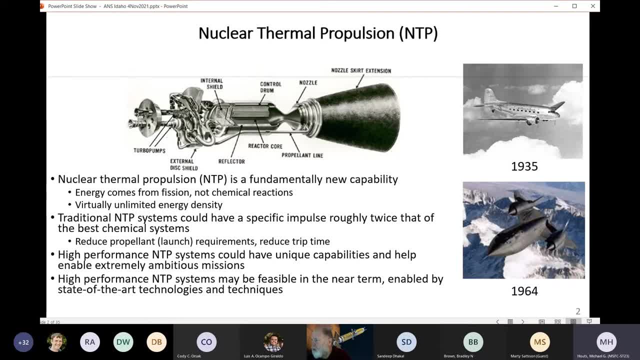 some energy density limits in chemical rockets. With fission I mean, you're millions of times the energy density of chemicals, So that really removes that particular constraint. And so again, talking about, as Mark mentioned, the traditional NTP systems that we've been working, 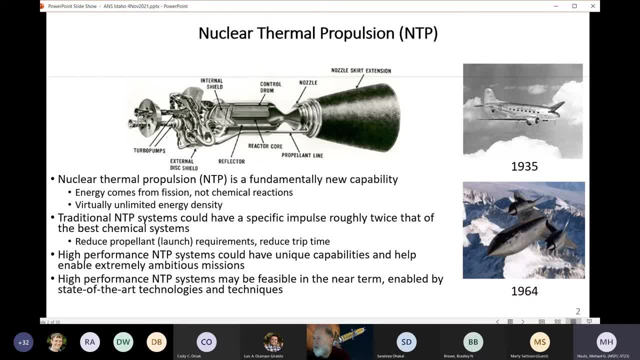 on And of course Doug Burns is leading the effort really for DOE and certainly NASA's interface with the DOE. The traditional NTP systems have a specific impulse. pretty good, It's about twice that of the best chemical systems. So rather than going maybe 460 seconds, 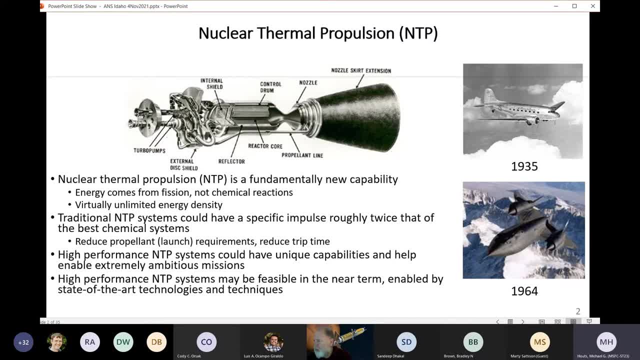 which is our best? liquid oxygen. liquid hydrogen engines probably can get over a 900 second specific Impulse, or at least around 900 second specific impulse with your traditional- you know, I guess, say it's just solid fuel, nuclear rockets. But if you go the next step beyond that, because again, 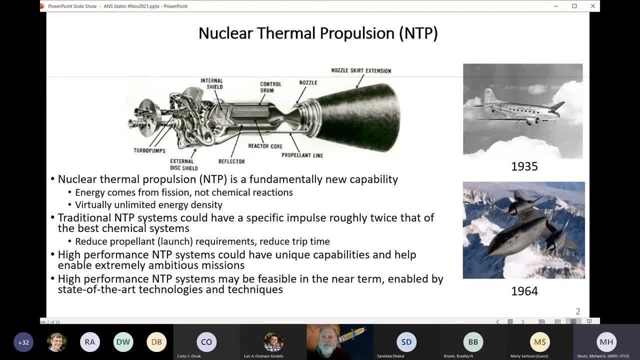 we don't have a, we don't need chemical reactions and we have essentially unlimited energy density. It's pretty, you know again, impressive what you might be able to do with fission systems. So we'll talk about that in a couple of slides or start talking about it. But did want to give 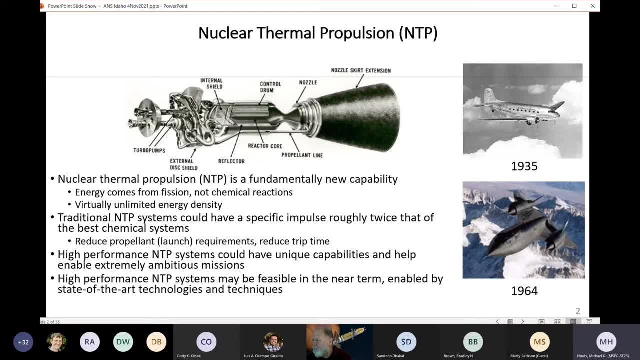 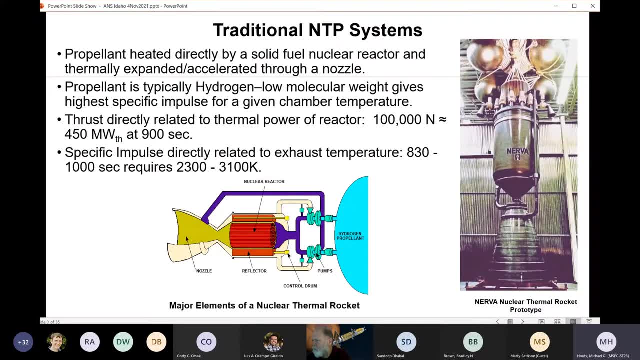 one more slide, just again, just the fundamentals. With a traditional nuclear thermal rocket- you see the hydrogen propellant tank on the right- And a lot of times for a human Mars mission, we'll be talking about hundreds of metric tons of propellant or more, And so it's a lot of propellant. And again, in the case that we have, 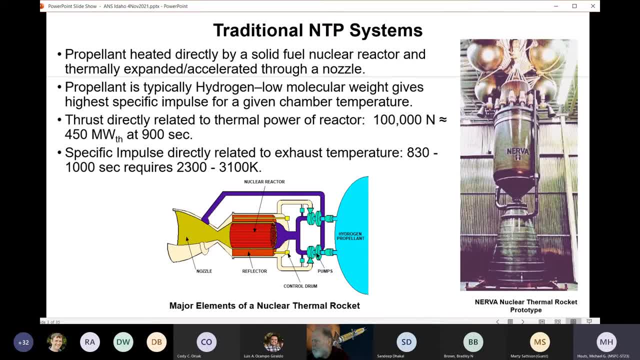 hydrogen, and with hydrogen being a low density, those hydrogen tanks also become extremely large. And so two challenges using hydrogen. One is we have to keep it cold. Even in space, it's hard to maintain 25. Degree Kelvin temperatures, which is about what we need for liquid hydrogen in that propellant tank. 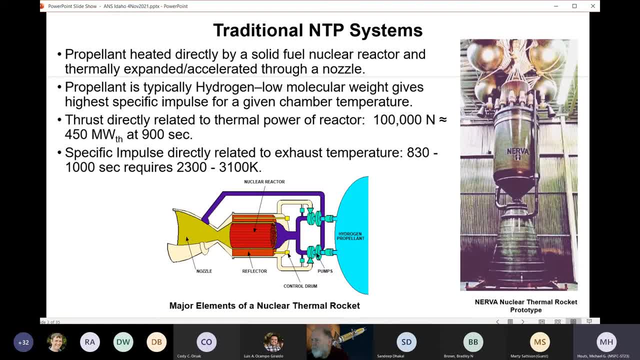 And even though when it's liquid it's a, it's a low density, And so those are two constraints that will come into play, because a lot of our, a lot of the commercial launch vehicles, a lot of the launch vehicles that we potentially might have available, they're actually volume limited instead. 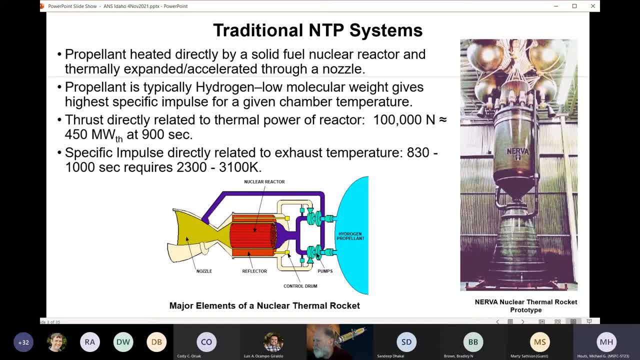 of mass limited. So in other words, we're limited by the volume within the payload shroud, how much hydrogen we can get into orbit versus the actual mass. And so we're limited by the volume within the mass limit of the reactor. But again, essentially, with the solid core rocket you have the hydrogen. 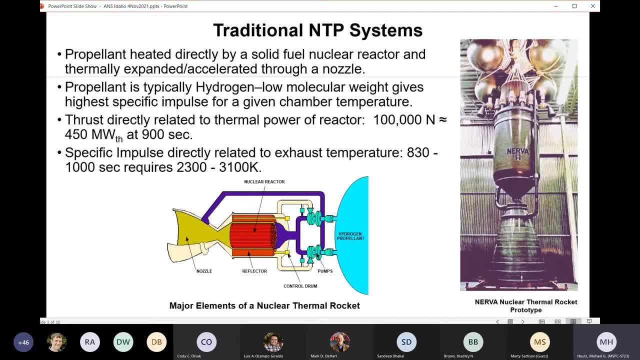 from the tank. We basically use it to cool the nozzle. We regeneratively cool the nozzle. We'll have temperatures- you know, propellant temperatures- ideally up around 2700 Kelvin, going through that nozzle. So we have to cool the nozzle walls. We cool the neutron reflector, We cool the. 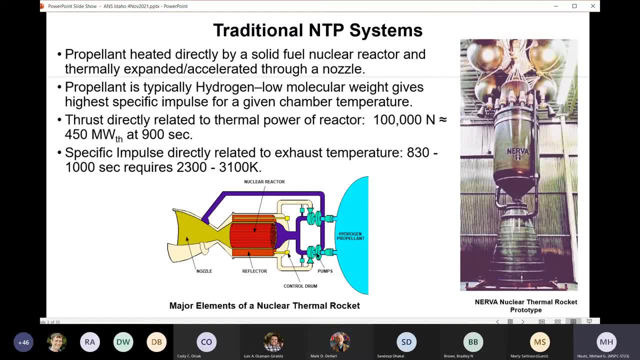 neutron moderator. Then we use that energy to actually be powering the turbopump which is, you know, pumping the hydrogen, So basically bootstraps itself. And then that hydrogen, after it's cooled all of the structural and moderator components, it goes through the fuel and is exhausted again. Right now we're 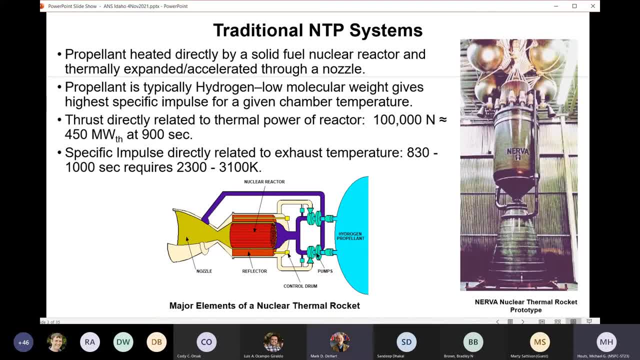 looking at trying to get to temperatures about 2700 Kelvin so that we can have the 900 second specific impulse exhaust. Now, if we want to talk about high performance nuclear thermal propulsion systems, what we're really looking at is, well, what you know. what would be the next step up? What would 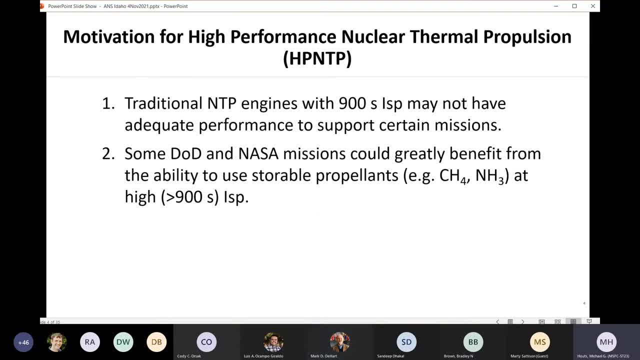 really get people excited about, And so one of the things we start to run into a little bit is the 900 second ISP might not quite be adequate to support certain missions, And one of those is of course very quick round trips to. 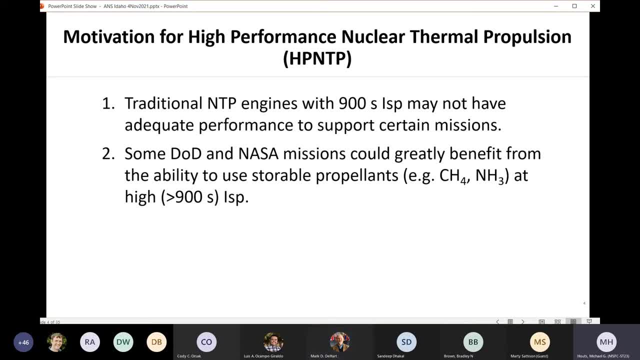 Mars. when people start talking about trying to get human Mars missions down close to a year, You really need a much higher specific impulse. And the reason for that close to a year is that's our experience on the space station. In other words, we've shown we can keep. 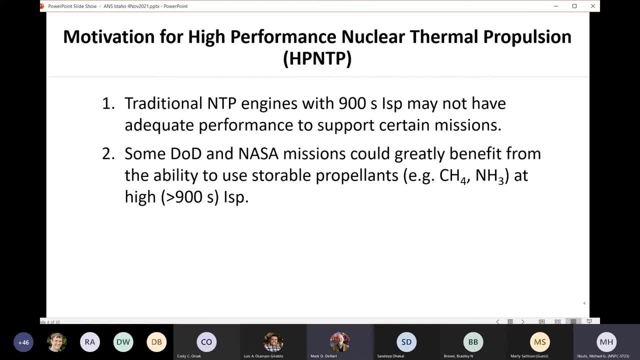 astronauts alive and reasonably healthy on the space station for about a year, And so people are generally comfortable, or more comfortable, at least, if we have a mission where those again the astronauts, will only be away from Earth for about that period of time, And so 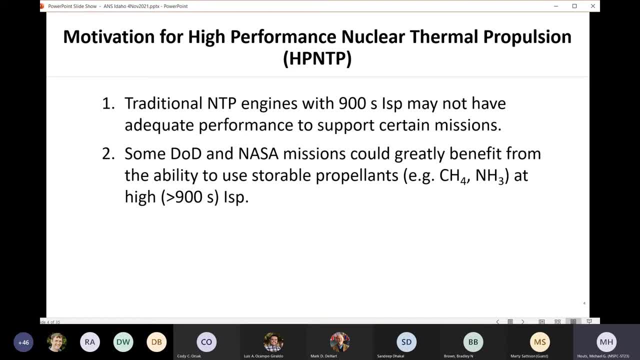 that's the push. If we could get close to a one-year round trip, would that generate enough interest or enough confidence in that human Mars mission that the US would actually commit to that mission? Right now, with the 900-second ISP engines, we're unfortunately up closer to two-year. 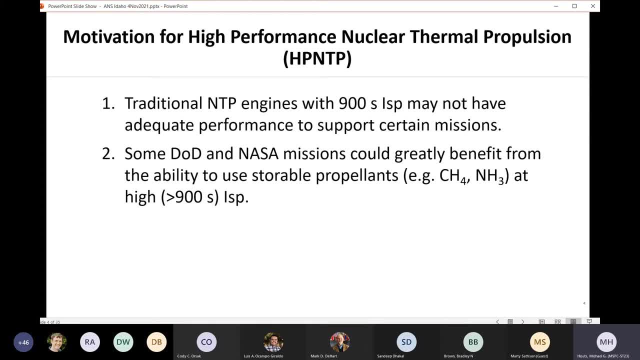 round trip missions. We have a recent study saying that if everything worked perfectly we could get down to maybe 670-day round trip And then probably that was a pretty hard opportunity. So there's probably some architectures. we could go even faster than that, But we're still. 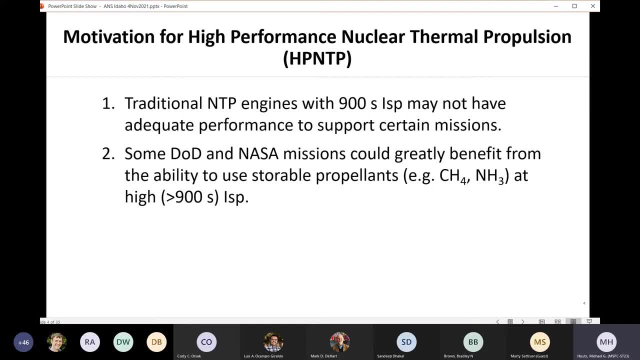 quite a ways above that. one year- that might be a threshold for some people- And the other one. this goes back to what we're doing in the space station. We're doing a lot of work on the space station. So we're doing a lot of work on the space station. We're doing a lot of work on the space station. 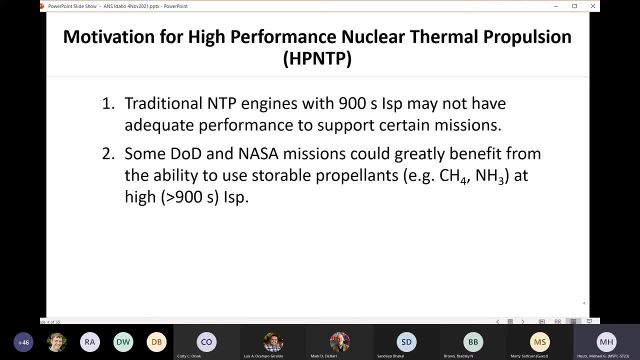 We were talking about with DOD, you know, NASA missions just associated with using hydrogen. Hydrogen is, again, it's hard to hold on to, It likes to leak, It needs to be kept very cold And then also it has a. you know it takes up a lot of volume. 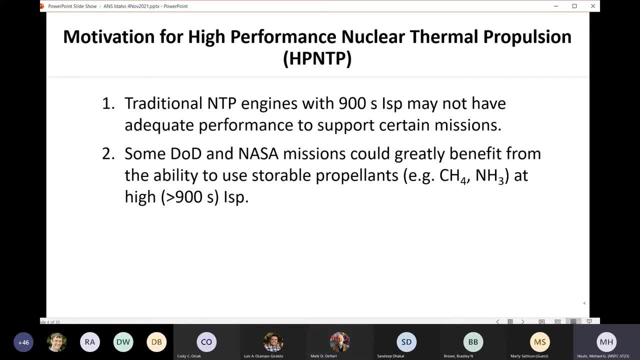 So the idea would: be well, could you devise a system that might let us use more storable propellants, you know, say, methane or ammonia or two that come up a lot Methane, of course, SpaceX, Elon Musk, he's talking about having liquid oxygen. 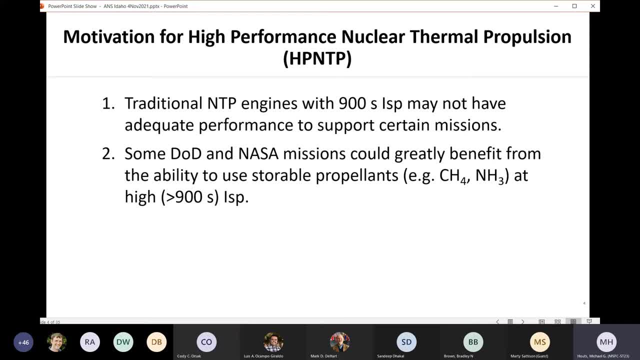 You know, methane, liquid methane, actually propellant depots in orbit. Ammonia turns out to be just incredibly storable in space. It doesn't freeze, It doesn't boil, And so it's really in a kind of a sweet spot with ammonia. 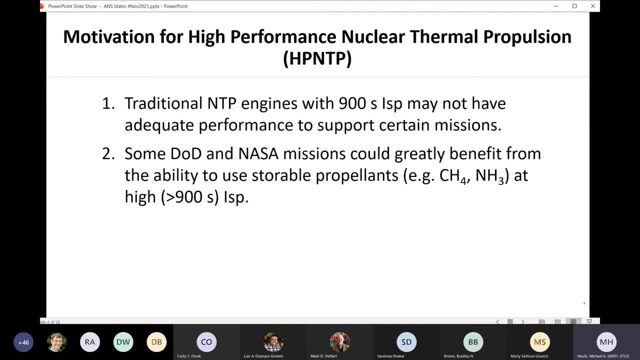 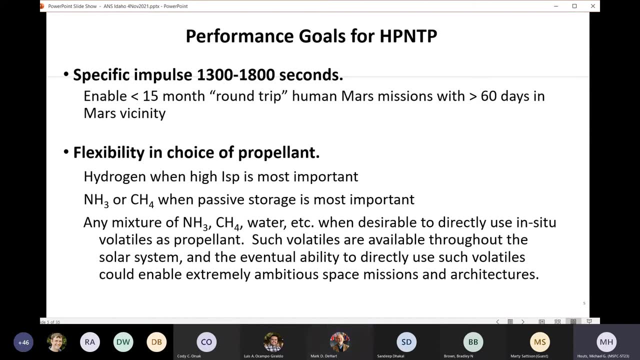 So those are two that are often mentioned in conjunction with NTP, or, you know, methane, of course, also storable for chemical systems as well. So when we're setting these performance goals, what we came up with was saying, OK, you know what are possible, you know reasonable performances that would still 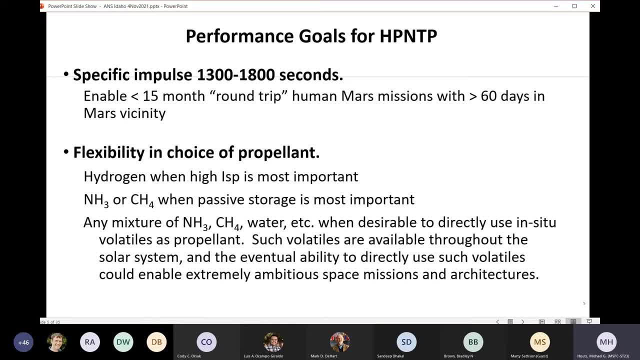 enable these types of missions, And so the, you know, a year. of course, we immediately said, OK, less than 15 months. we should be able to get people interested, And then some of the feedback we got was that people really wanted about 60 days in Mars. 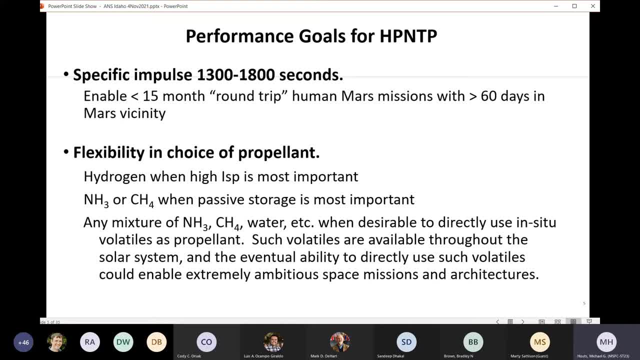 vicinity. In other words, that would make sure that we had time in Mars vicinity to you. know, essentially, you know we're in orbit and you know, have time to make sure we can get down on the surface. You know people can spend time on the surface, have time to get back up on the surface and get 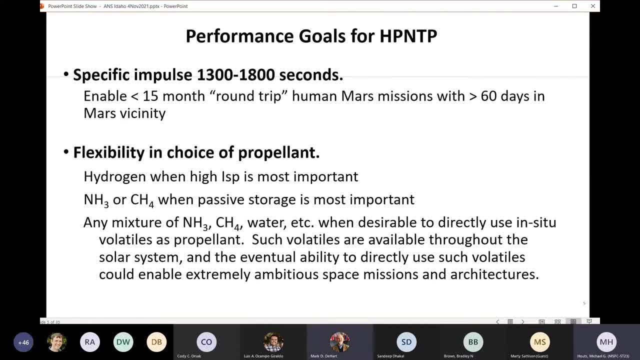 you know and start the trip home And so, and you know and have adequate time for exploration on the surface. So that was kind of a one performance goal. And then the flexibility and choice of propellant. you know hydrogen when the specific impulse is. 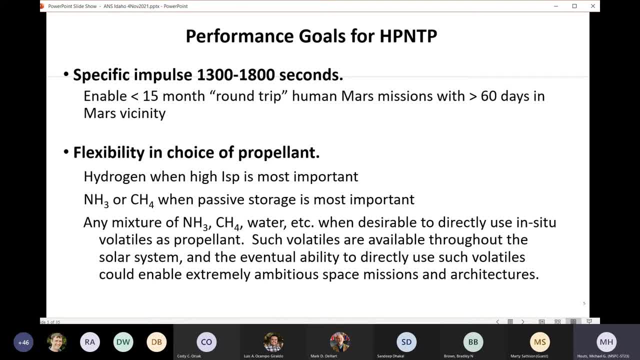 most important, ammonia or methane, when passive storage is most important. And then, if you really want to look futuristically, there are a lot of volatiles around the solar system, But usually it's going to be this: you know, say, some kind of a body like a Kuiper belt object or another. 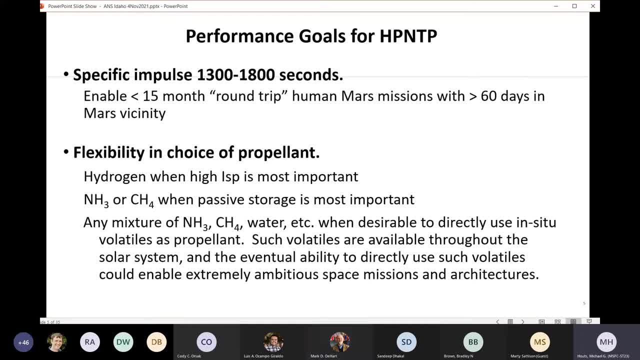 object that really has it's going to be. usually it's a mixture of ammonia, methane, water, you know, maybe a few other volatiles. So the idea would be: is there a simple way to use those volatiles as a you know? basically? 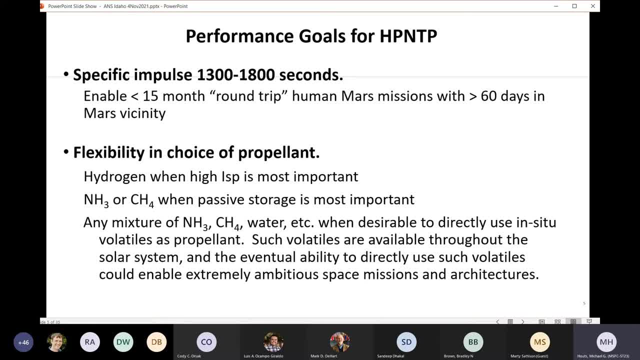 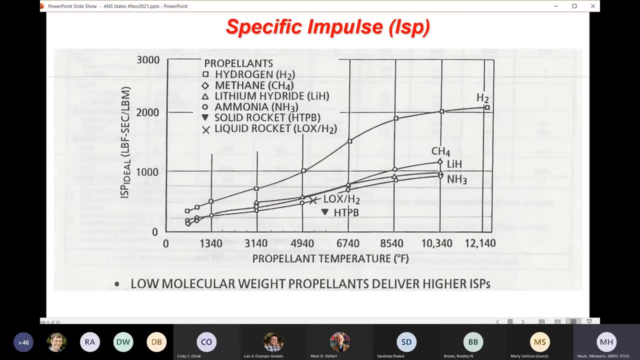 just simple way to use those propellant too. And so that's, you know, another, I guess, goal of this type of system, which is again kind of a more advanced version of a nuclear thermal propulsion system. Okay, So to get to that specific impulse, and that's in this, you know again, 1300, 1800 second. 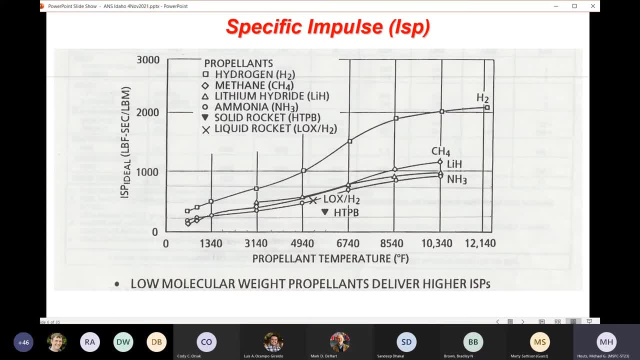 range. what we really need to do is first get the temperature up And then also, in the process of increasing the temperature, well, we can take advantage of dissociation. So you see, on this curve it's in Fahrenheit, but basically like 4940, I think is 3000 Kelvin. 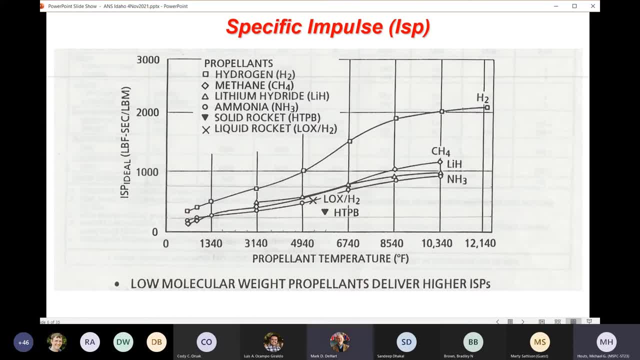 8540 is 5000 Kelvin, And so the during in that range you notice that the curve goes non-linear. and what's happening there? for example, the upper curve, hydrogen- well, it's actually dissociating, And so you're going from H2, when you're down around 3000 Kelvin, basically up to monatomic. 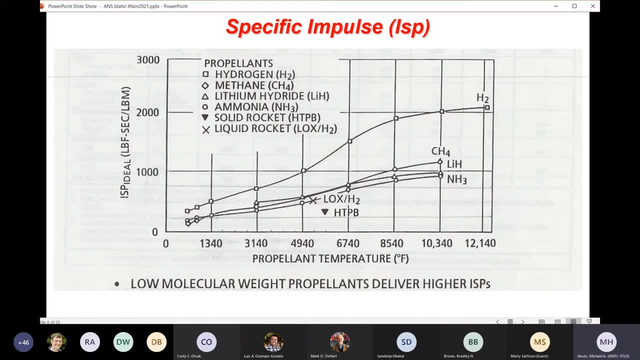 hydrogen when you get close to 5000 Kelvin. So it gives you the a boost in a specific impulse And that's of course in that range. you're getting up a little over 1800. second specific impulse with hydrogen. 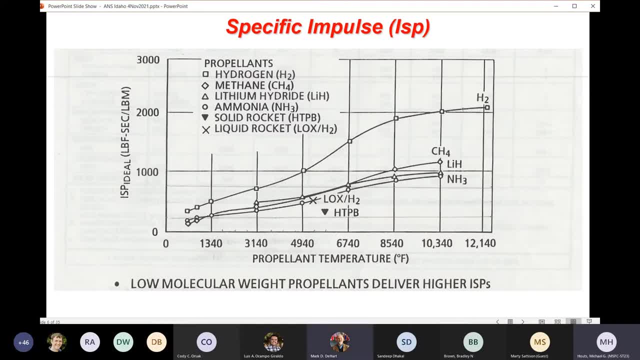 And then with methane. Again, you see it's. it also dissociates. And so, instead of having CH4, you would end up having it dissociated into a carbon and four hydrogens. And again, the advantage of dissociation is it's reducing the molecular weight. 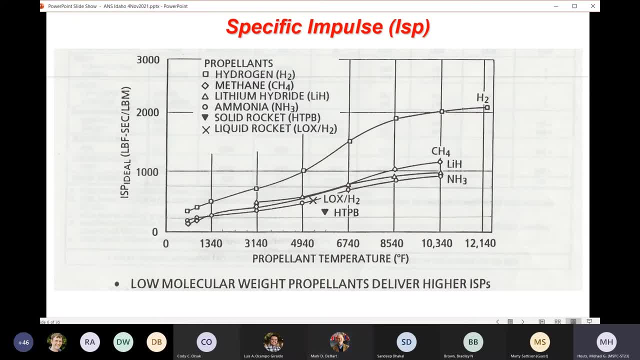 So for you'll get. in the case of methane, your effective molecular weight goes from 16 down to 3.2.. In the case of hydrogen, your effective molecular weight goes from two down to one. And so that's what the you know, that's that's kind of the you know the incentive another. 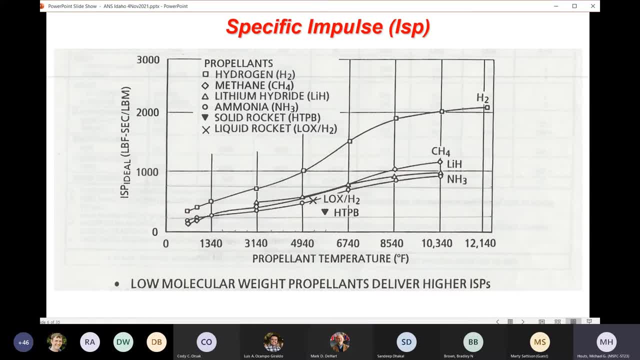 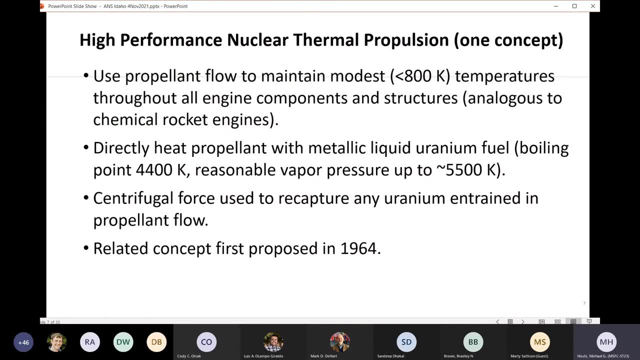 incentive to go to high temperatures. So then of course the question is: okay, if so, that's obviously way above any kind of reasonable temperature to run a solid fueled system. you know you can't. I mean you're not. 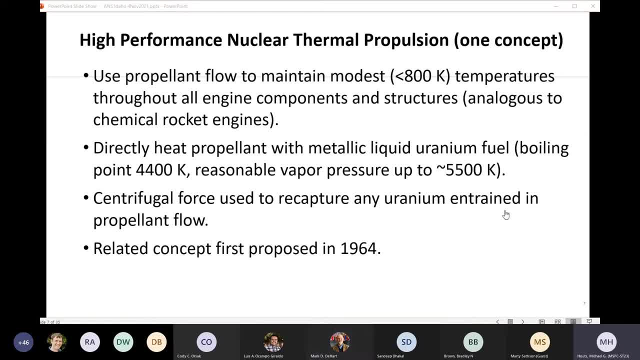 sure how else to phrase it other than that's just, you're obviously not going to keep any solid at those temperatures because you're looking at needing, needing to be close to you know again, close to 5000 Kelvin. And so what one concept is- and that's what we've been talking about today is is basically to go ahead and use the propellant flow to maintain modest temperatures throughout the engine components and the structures. 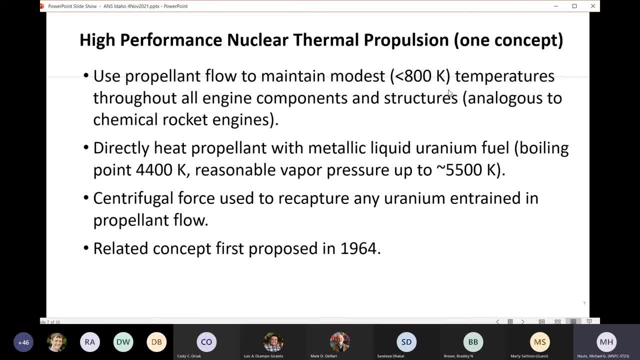 And so that's very analogous to chemical rocket engines. If we look at a typical liquid hydrogen, liquid oxygen engine, the temperature is actually in the- you know 3600 Kelvin range when you get into the combustion chamber. So you actually have a very, you know, very, very hot gas in there. 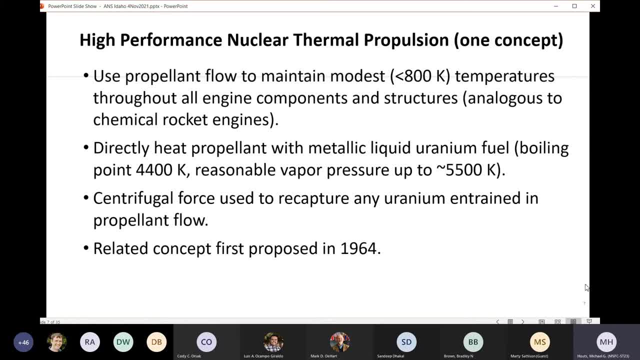 But you're able to. You're able to keep. your walls are actually very, I guess you'd say, the walls of that chamber. you can actually use some pretty low temperature materials on them because of the way you use a transpiration cooling film, cooling just by how the propellant is plumbed. 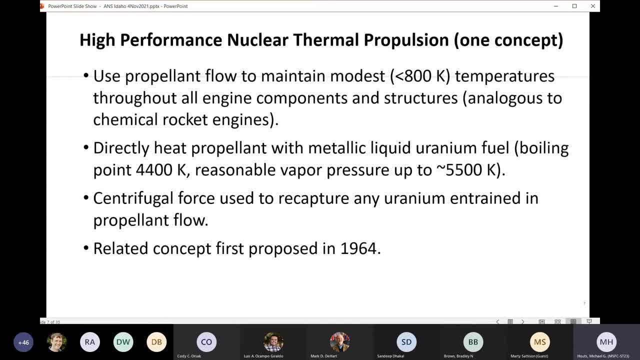 And so we would do kind of the same thing in a in the nuclear rocket And then the on the then to get the propellant hot, what we'll be doing is direct, basically directly, The heating propellant with the metallic liquid uranium fuel, the. the boiling point of that metallic uranium is about 4400 Kelvin. 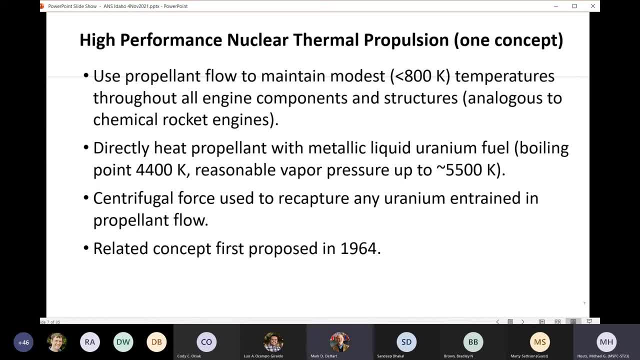 You do keep a reasonable vapor pressure up to about 5500 Kelvin And you're, of course, you're melting points down around- I think it's 1404 Kelvin And so the go back. So you're, you're boiling points down around the 1404 Kelvin. 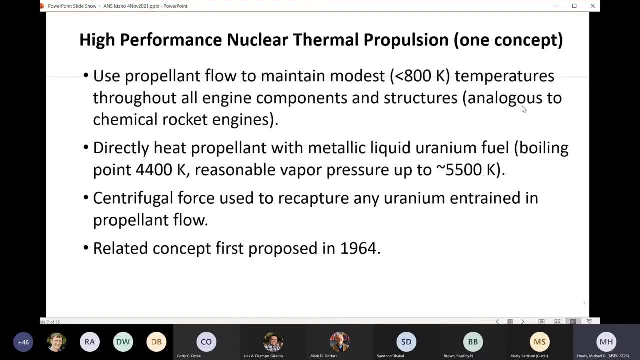 So I mean, I'm sorry you're melting points 1404 Kelvin So you can run it liquid. It can melt at reasonable temperatures And of course You know just from our experience working with molten uranium metal. you know one material is zirconium carbide is very compatible with those temperatures and there might be others. 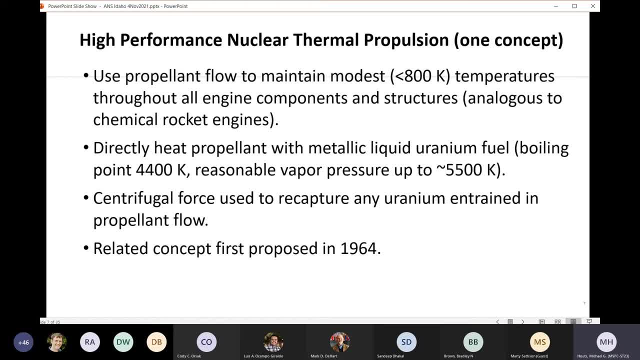 So you have a way to melt it, And then again the boiling point stays reasonable or the vapor pressure stays reasonable up to a fairly high temperature. Now the key is then to contain it. Different ways have been proposed for containing it. It seems like most people have kind of settled on trying to use centrifugal. 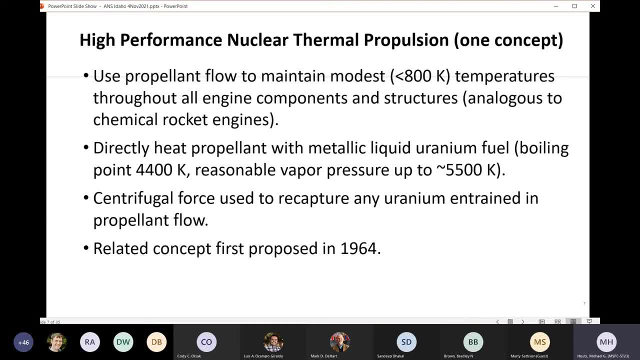 Force, at least for the initial systems, And so that centrifugal force both helps with the containment of the fuel as well as is recapturing any uranium that's entrained in the propellant flow. And these are first started being talked about. probably about 1964 was the first time this particular ideas appears in the literature is actually I think it was the first. I think it was like volume one of the Journal of Spacecraft and Rockets. 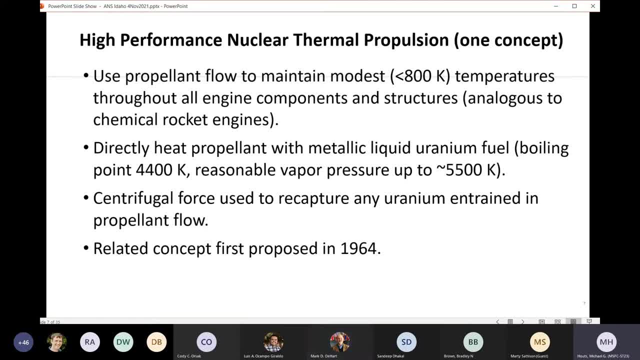 So it's actually one of the you know kind of right when we were really starting to do a lot of Papers, a lot of research related advanced propulsion systems, It was one of the first papers. There's a lot of really good work done it over at Princeton. 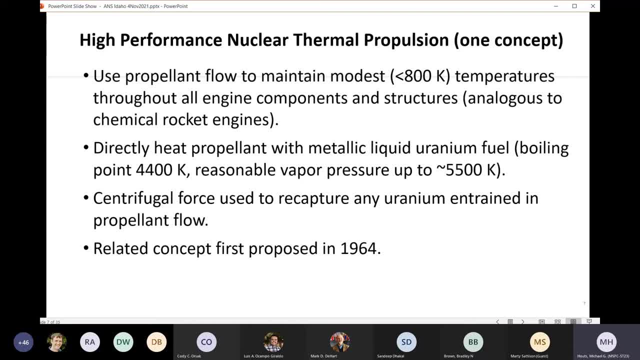 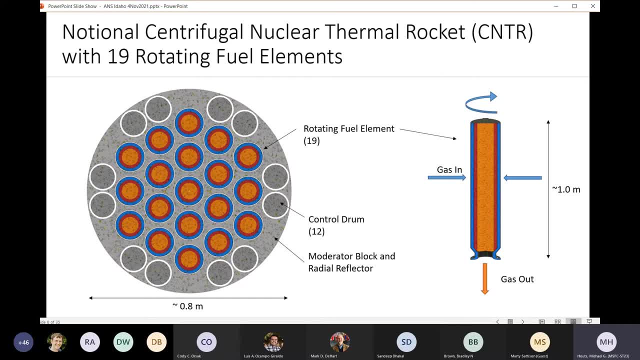 So, in a nutshell, the way it works. I'll pause after this slide just to make sure Well, a, that I'm not on mute and B, that this is making sense. But but basically, in a nutshell, the way it works is: you just picture those kind of the orange elements with the, and I think I think on zoom the pointer works. 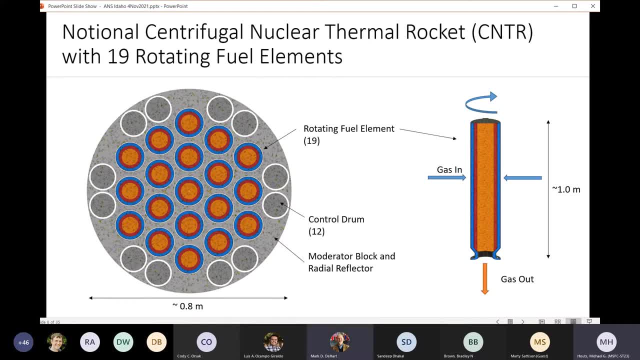 So you picture this is the. These are each fuel cylinders and in this you know again just a very you know first cut non optimized MC and P analysis. This is just a about 10 centimeters across the cylinder, the blue region, I think in this model it's a silicon carbide wall with a zirconium carbide layer. 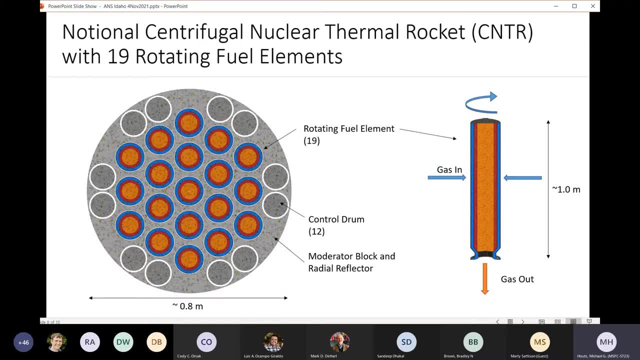 Now we could certainly make the wall out of a different material, but of course, the silicon carbide being pretty much transparent to neutrons, If we can use that as a Structural material, it's good. It would be running about 800 degrees Kelvin, so it's a reasonable temperature for silicon carbide. and then you have a zirconium carbide inner layer and that's for the compatibility with the uranium. 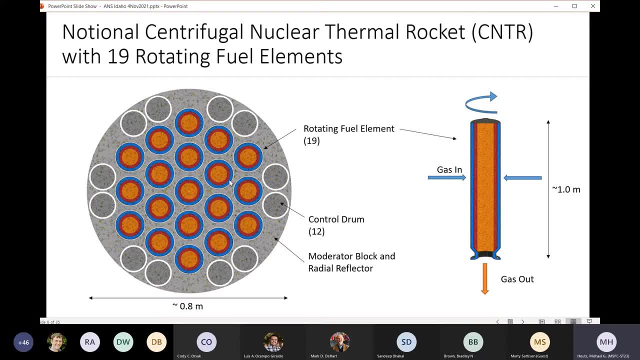 Then that red region is where the liquid uranium fuel would be, and so the so that's the region literally, where it's going from about 1400 Kelvin to maybe 5000 Kelvin on that inner surface And then the Kind of orangish layer on the inside. that's the mix of at that point. hopefully it's mostly propellant, but it could also- there probably will be some uranium entrained in there. so we've got about six universities working on this right now. 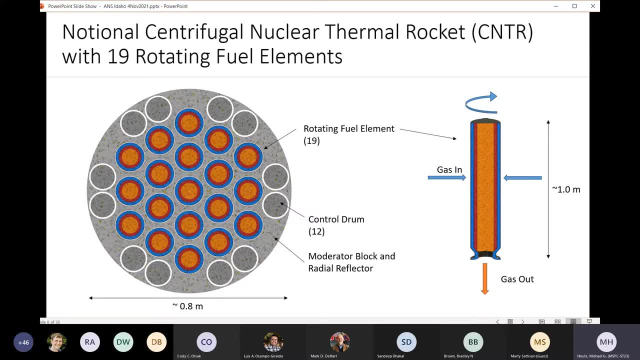 No real industry effort yet, but so one of the so University, Alabama, Huntsville, you know, right here next to Marshall, they've been looking a lot at the bubble heat transfer and so that's basically this propellant going through the metallic. 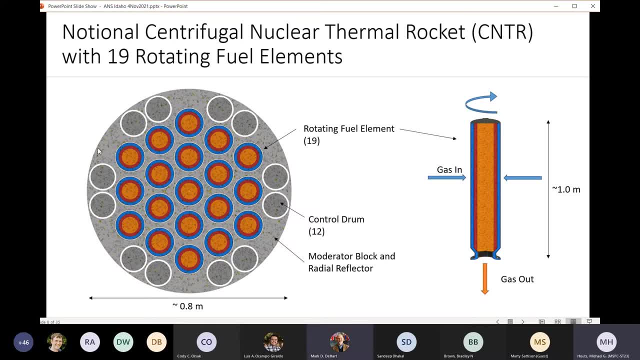 Liquid uranium. So the heat transfer is really good. That part looks promising, It's. we're going to have to, you know, basically optimize the propellant flow channels, you know, radio in the wall to make sure that we can keep the wall cool enough, because of course the metallic uranium does have a very high thermal conductivity. but the 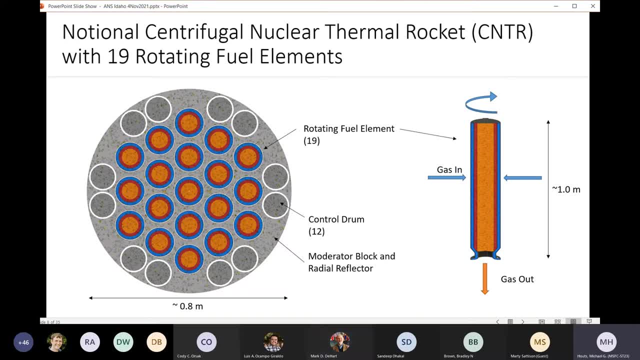 Yeah, but but again it's you know, overall you'll get excellent heat transfer between the Uh, your Uranium- and the propellant, and so we can actually keep the propellant pretty close to the- you know, pretty close to the temperature of the metallic uranium fuel. and then over here on the right- this is just a schematic. again, it's this picture: 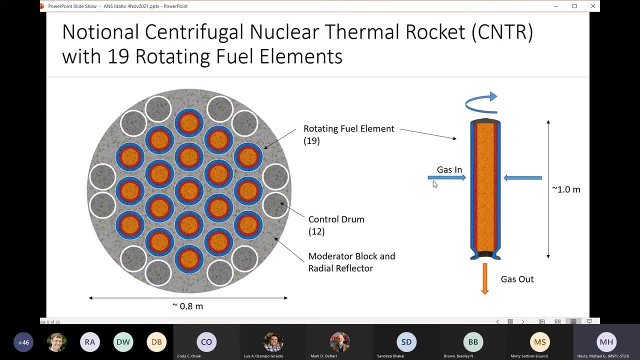 If any of you are familiar with timber wind and the old space nuclear thermal propulsion concept, there's a basically a particle bed reactor. It's pretty much the same flow path as that, but instead of in this cylinder cylindrical region, here, instead of having a packed bed of particles and a cold frit and a hot, 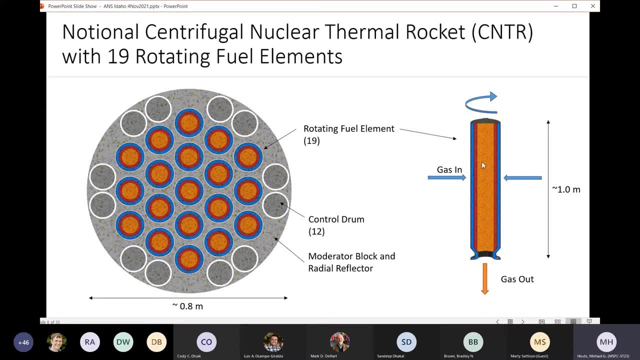 Frit because of the really high temperatures. again, trying to get our propellant up, say, 5000 Kelvin, we end up having to rotate it instead. We can't have a hot for it, and so it's a and. so that's the. the big complexity of this is having to rotate these cylinders right now. 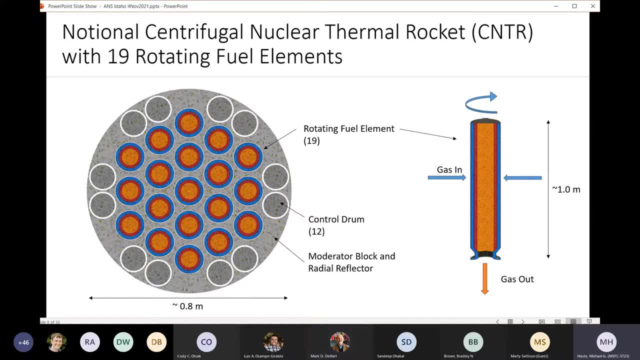 It looks like it's going to end up between 1000 and 5000 RPM, and so it's you know, it's it's you know. we can obviously rotate things much faster than that. I mean turbo pumps run over 50000 RPM. 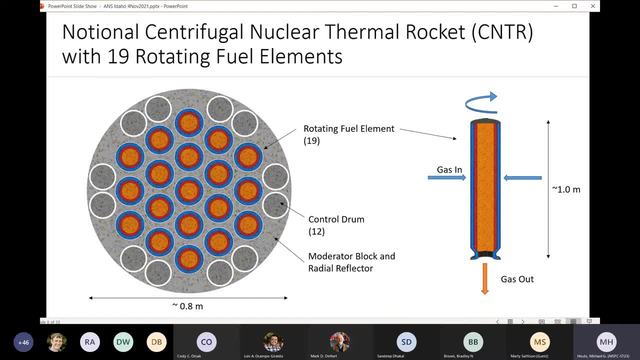 But this is also. this can be about a 10 to 20 kilogram cylinder and you know, and get a lot of other constraints. So it's so that's. that's definitely a non trivial engineering challenge. So any any questions at this point? 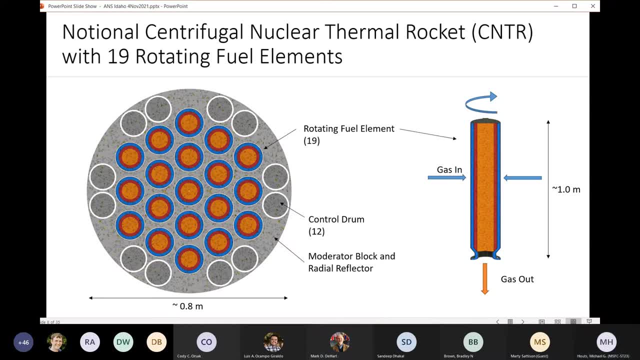 Yeah, Mike, yeah, good question for you. This is a Gilles. Thank you How you doing Good and you Good thanks, Good. What? what is the power source that is used to make the cylinders spin? Is it electrical or is it directly from the the? 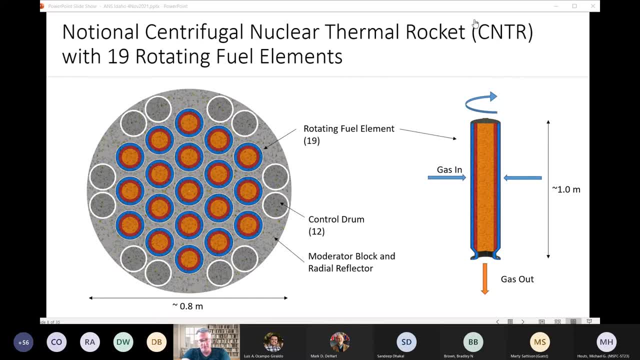 The coolant flow. yet so from the coolant flow, let me So this is the general idea. what we would have is- And again, these are all 100% notional and so exactly the you have this, this picture, in this diagram. 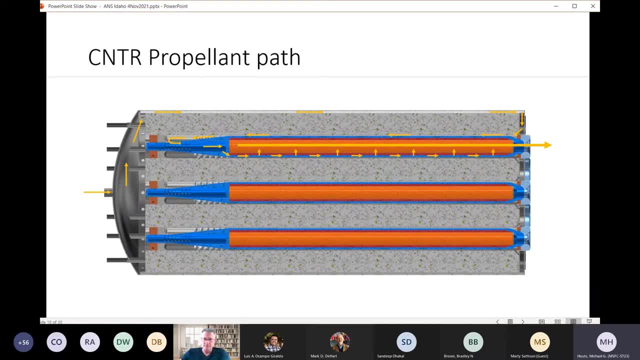 The propellant tank would be off here to the left And so we do the standard. you know, turbo pumps, everything from the traditional NTP and all of the gray is basically the same as a traditional NTP. Have your structure, your moderator and then not shown here would be like control drum. 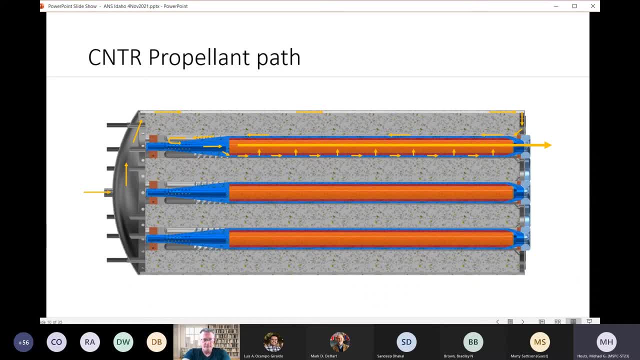 So everything's the same as the solid core NTP, But then the propellant. a couple key areas will have bearings down here again, Remembering that this, this area- here We're trying to keep it about 5000 Kelvin and these areas here. 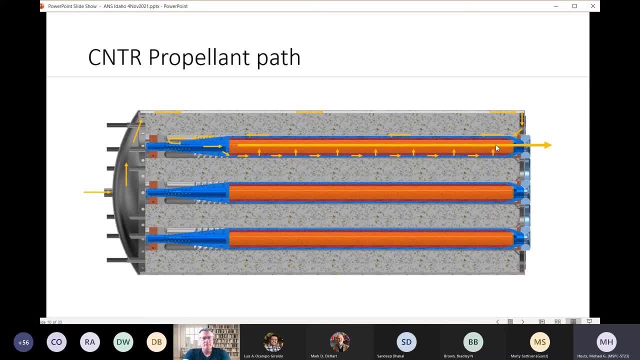 We've got to basically have enough cooling to keep those walls at a reasonable temperature, And so we'll probably even might even need to be bleeding some propellant through those walls. But anyway you have. the propellant comes up along the side in this particular one. 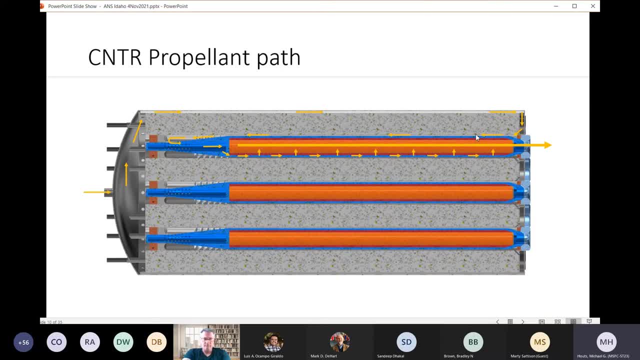 It would enter the cylinder at the top and then, you know, spin it via these veins and then comes down radially along the side of the spinning cylinder. So this gray is stationary. The blue is your inlet plenum. That's where your propellant is flowing. 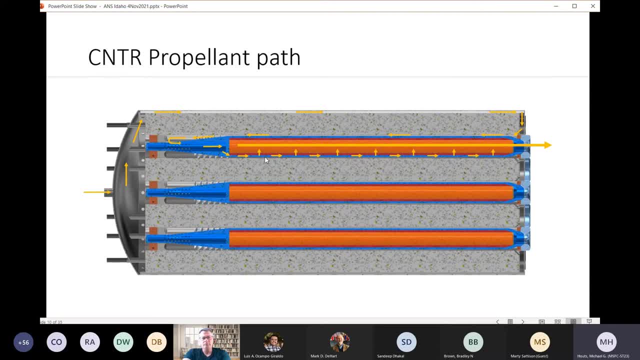 And so, and then the red is: is, you know, on the inside Again, these are definitely, obviously aren't engineering drawings, but that's- but in inward of that is where everything is spinning, And then the propellant again flows a radially through the fueling out. 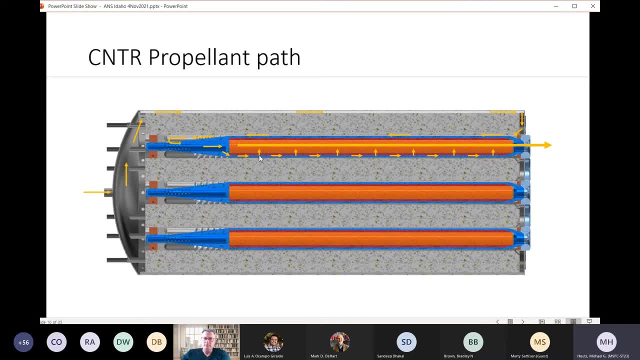 But, but yeah, for so we're talking about using the hydrogen, the propellant, basically to spin the cylinders Now during startup, the. You know we can get to that, We can get to that. We can get to the point where the uranium is melt, molten. 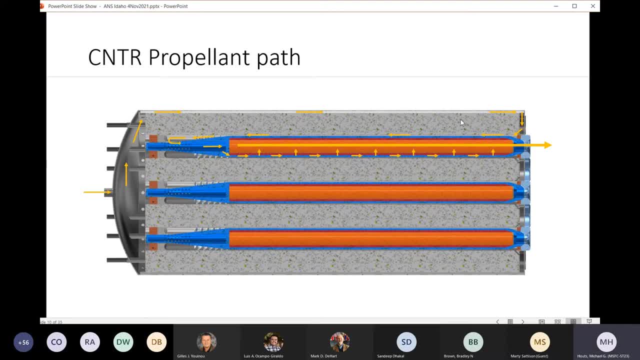 You know, because, again, if this is zirconium carbide and silicon carbide on the side, we can use those at above the melting point of uranium metal. But probably before we melt we're going to want to start spinning these cylinders. 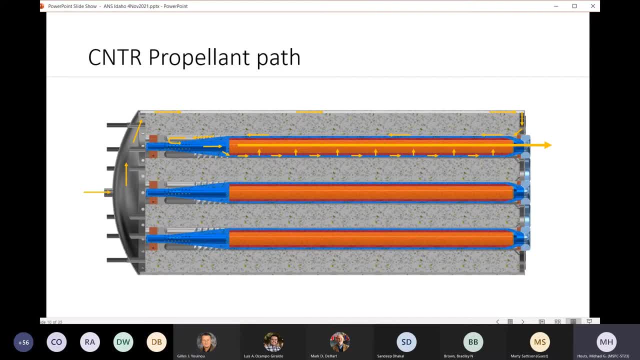 Yeah, really just to hang on to the liquid And so that's so. that's one where we could go to a electrical drive, and the electrical drive gives you some benefits too. I mean it gives you a lot more control than just having to use the gas pressure coming out of the tank. 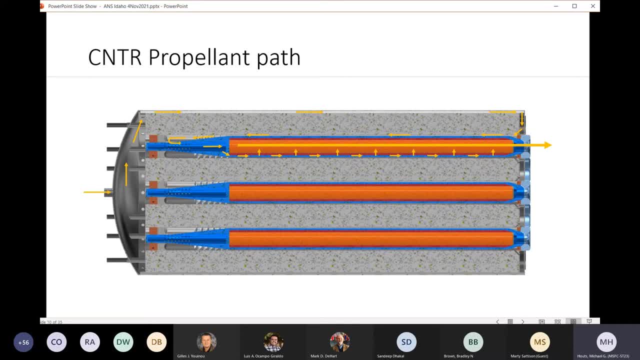 And so that's definitely something we're looking at also, But we're not really. I think one of the- I think it's University of Rhode Island. Maybe they have a team that's looking at you know, maybe how would you, how would you have a combination of the gas drive? 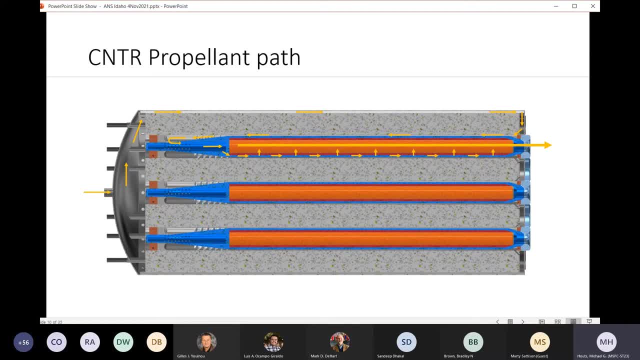 You know the? basically the turbine drive and the electrical drive. Okay, And using the propellant to spin the cylinders, that doesn't add too much pressure. drop too much constraint on the pumps. No, we'll have plenty of plenty of energy and plenty of the pumps. 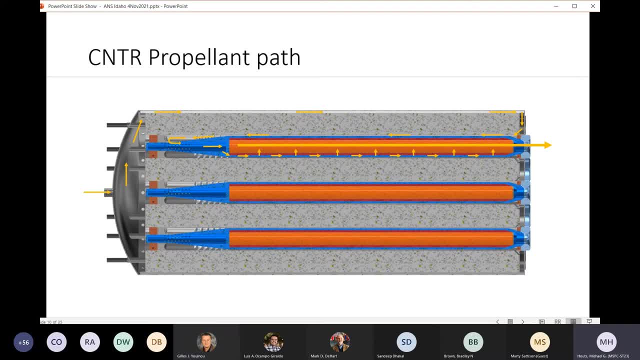 It's pretty low pressure system We're looking at. I mean, I'm sorry, compared to chemical rocket engines. You know, it's really fun working with the chemical rocket guys because, like we say, we want a 30 second start. They're just like: how could it possibly take that long? 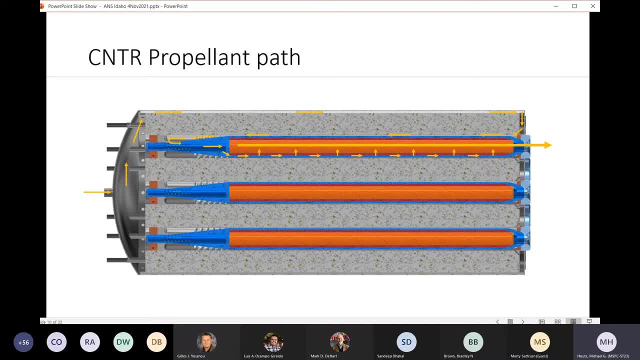 You know what I mean. It's a. It's kind of the same thing. when we talk about, you know, 500 psi, They say like, why so low of pressure? or 1000 psi, I mean they run in thousands of psi now. 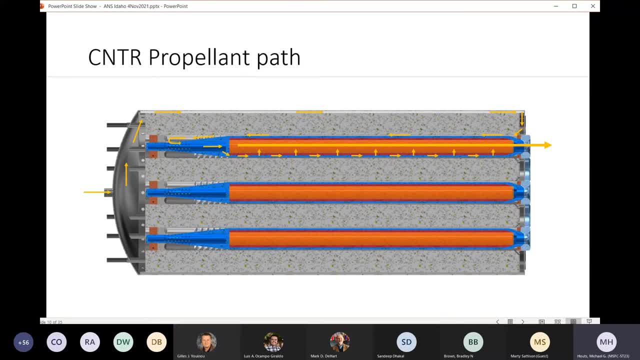 So, yeah, we will have, and we have enough energy from the rest of the system to be able to drive that. But again, lots and lots of really good engineering remains, And so so when I make statements like that, that's the you know. we saw it still needs a lot of engineering. 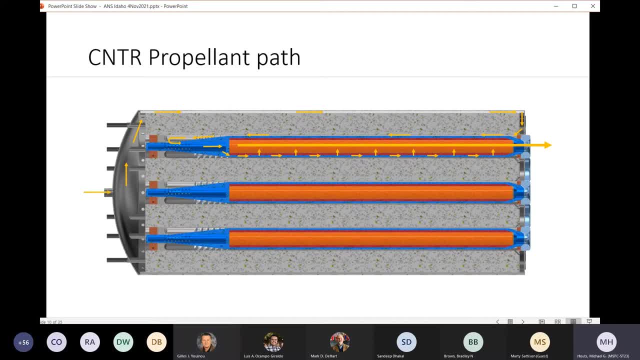 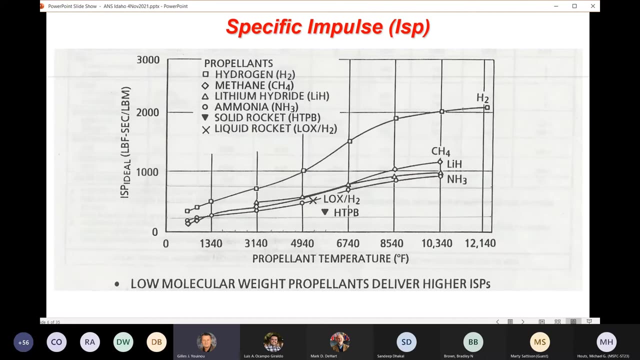 Okay, And just one more question. When you showed the, the dissociation Of the different propellant As a function of temperature, So this was for the same pressure? Yeah, So it's. So I'd have to go back. We've had. I think Aerojet Rocketdyne did this one and maybe- But I'd have to go back and check- It might have been done at 1000 psi. So I'm not So usually people are looking at either 500 psi or 1000 psi. 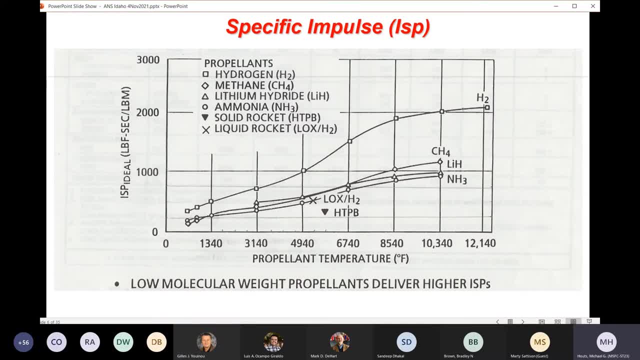 Yeah, So, so that's it. So, yeah, we need to go back and refine this, But the basic idea is, you know, if you can get up into that 5000 Kelvin range, you've had a huge boost just from the increased temperature. 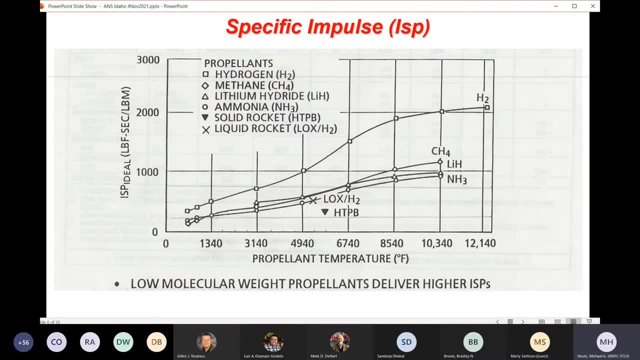 But again, you also- you know pretty much- have taken advantage of all the dissociation you can take advantage of. Okay, Thank you Mike. No, thank you Thanks. Yeah, It's. it's much more interesting when people ask questions. 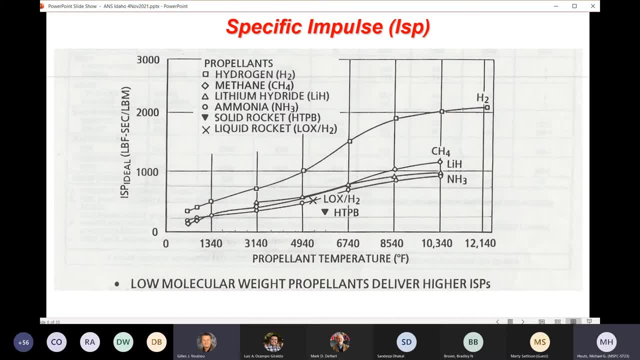 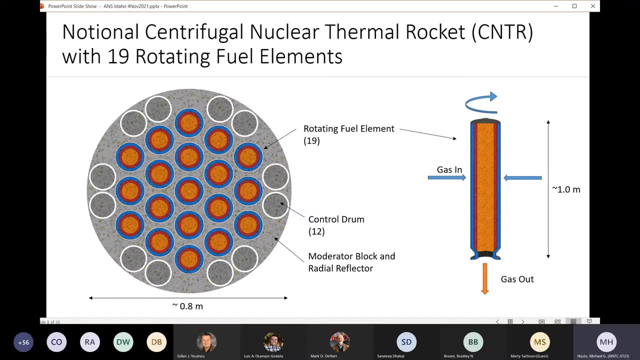 So so please, please, please, keep you know. Yeah, Anything else Is everything just the general operation. Is that sort of makes sense to anybody? or Yeah, it makes sense. It almost seems to be too good to be true. 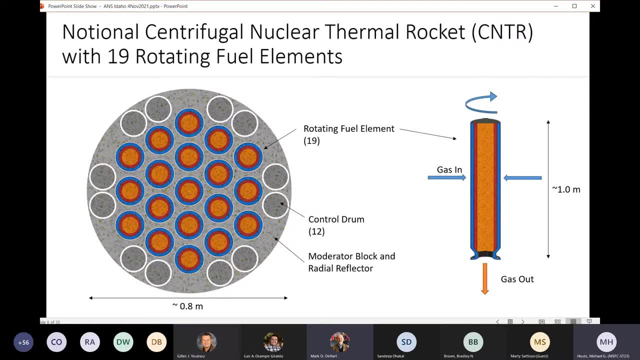 But I believe it. I just I need to get my hands dirty. Yeah, Hands are a little bit, Yeah, Yeah, The that's why we need good experiments and additional analysis. And you know, and you know because, because you're right. 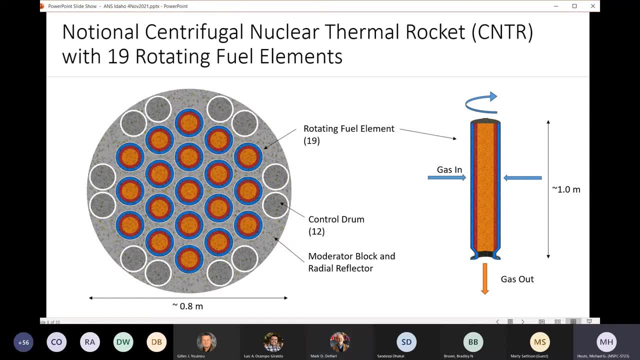 It's if it is you know, too good to be true. We want to find out as quick as possible. They call it the. I used to say we want to fail fast And then, but that always came across as too negative. So so now we look at the. I think we call it the AD squared: the advancement degree of difficulty. 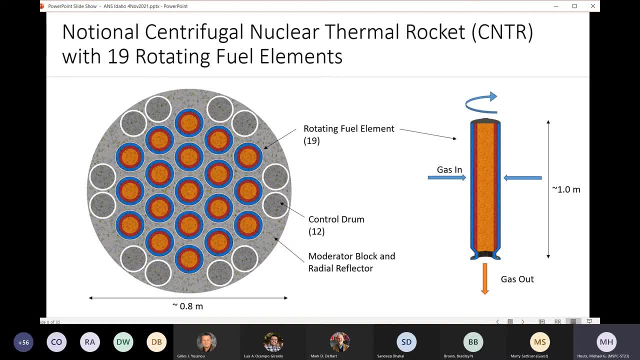 So you want to say it's the advancement degree of difficulty, It's at least acceptable, meaning you start doing like these, you know, spinning some cylinders and bleeding the gas through a liquid metal and everything just working perfectly, you know. So anyway, that's the positive spin. 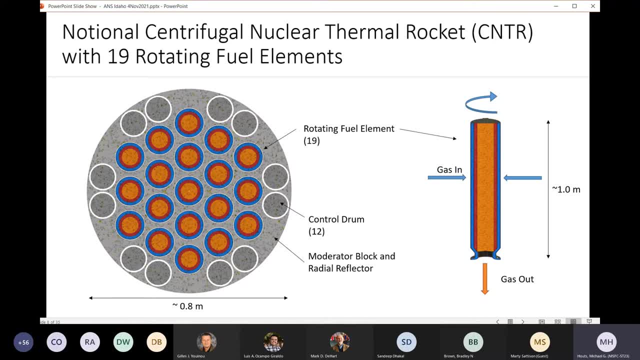 But the, the universities. right now, we're just. we got a lot of them. Well, they're doing experiments, but we also have them really looking for. Okay, Is there a? is there a fatal flaw here that that we're completely missing? 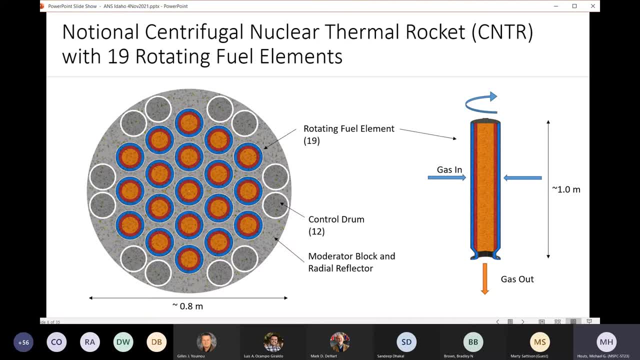 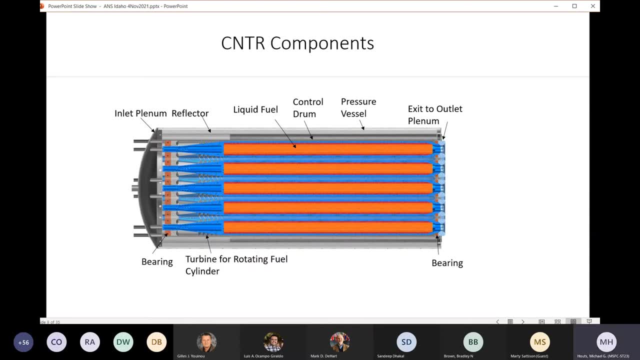 So this is just the Yeah, just a diagram. Again, just keep emphasizing: everything outside the rotating cylinders is quote-unquote normal. In other words, that's what we've been looking at for solid core, the ONTP, the materials, the beryllium reflectors, control drums, the moderator structure. 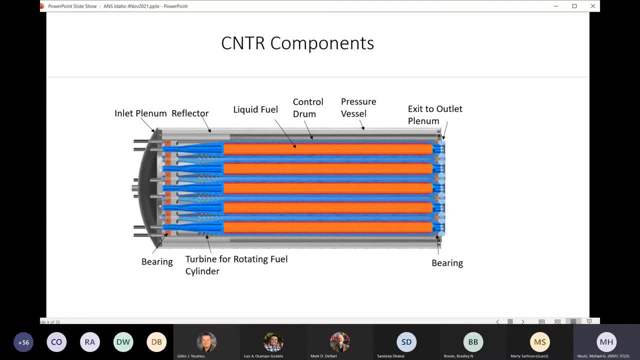 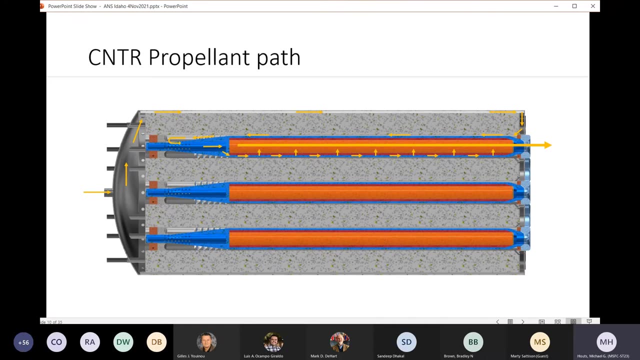 And then just where it gets completely different is when we get inside these, the fuel cylinders. And then I think we talked about this diagram a little bit. This is just again. these are all notional. So these are just some of the ideas, but just labeling some of the components. 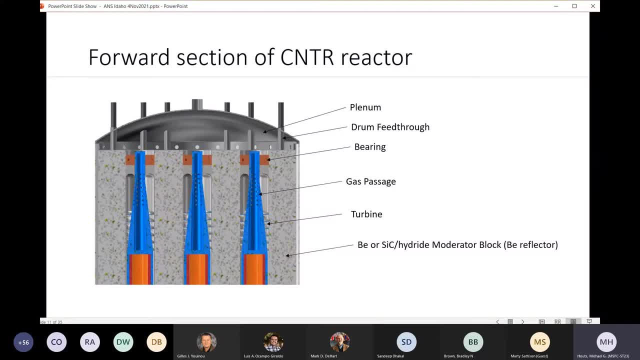 And I can send these charts, obviously, to anybody that's interested in them. But again, just very, very notional. I do want to acknowledge Tom Godfroy here at Marshall. Marshall did a tremendous amount of work just laying out the notional diagrams And he probably used the word notional 10 times more than I'm using it right now. 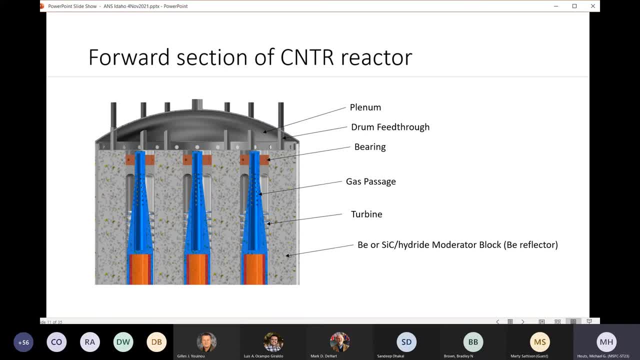 So he was just saying: don't again emphasizing these aren't engineering drawings, but just kind of communicates the basic approach And then at the end again just a little bit of the complexity. You have bearings on both ends that we'll need to keep cool. 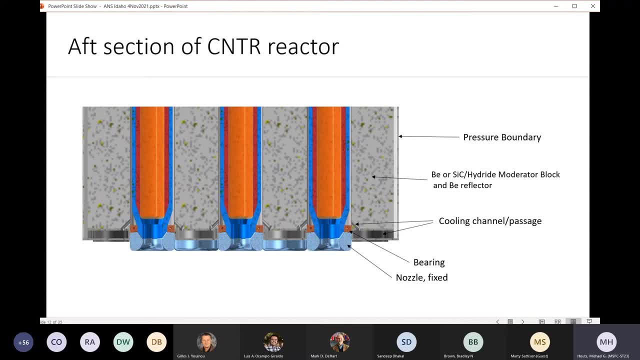 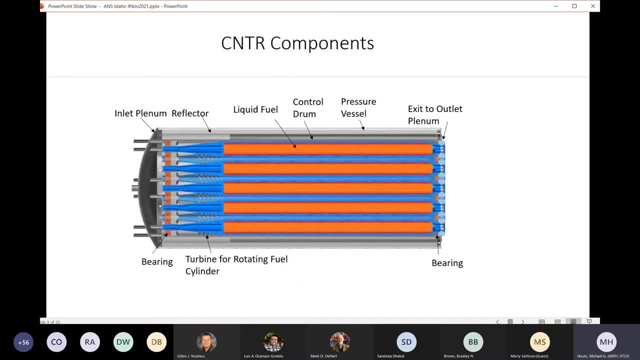 We'll have a nozzle. what we're thinking about, What we're thinking about doing right now, and this is all subject to- let's see if I got a better picture of it. Yeah, so we're thinking about each cylinder would basically exhaust into a common nozzle. 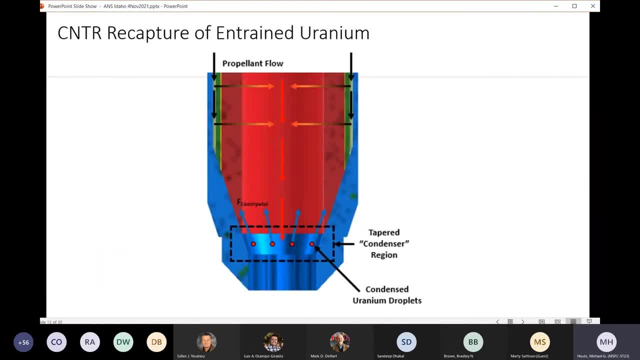 And then so you'd have a single nozzle on the engine, So the exhaust from each cylinder would then go into a nozzle. And then again we'd have to, just like we do with the chemical rockets. we'd need to use transpiration cooling, film cooling on the walls to keep that chamber cool enough. 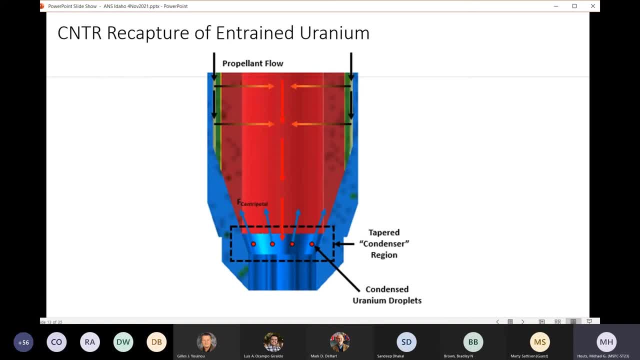 And then he'll expand out through. So it's a single nozzle per engine And then this is just a, again very notional. This was actually a let's see. I think it was an Auburn student that did a lot of this work initially. 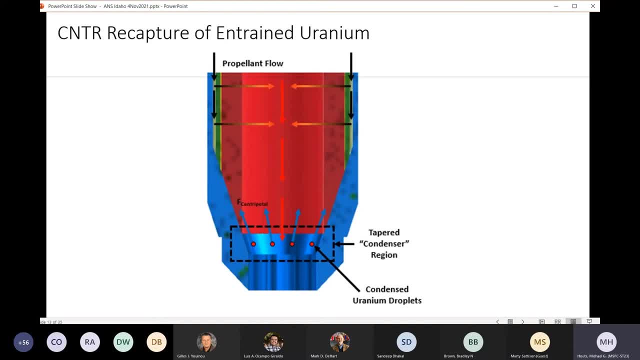 And then a few others are working on it now. It's just the idea that at the end of the cylinder you would start tapering in the wall. And so this is this region, here is the liquid fuel, and you would taper in the wall. 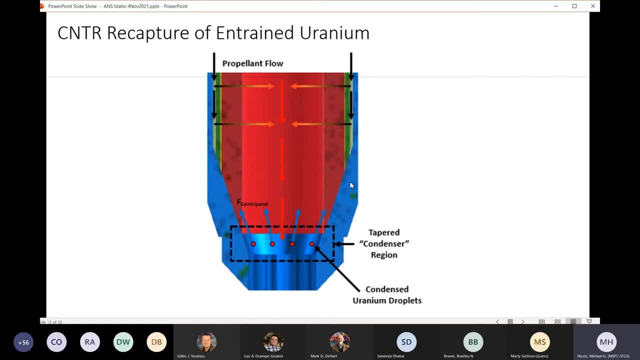 You know, and again you'd still have some cooling going through the wall to keep that wall temperature reasonable, And then this taper would probably continue, And so this is what we'd have to optimize: How much do we taper it down? But the idea would be any: make sure that any entrained uranium has enough opportunity to condense on that wall, which again is going to require wall cooling. 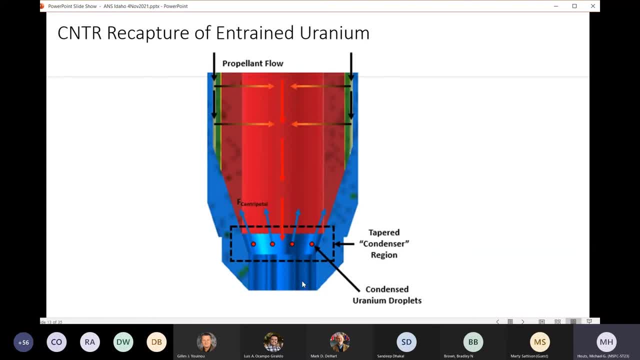 And then just the you know, the centripetal force would just, you know, naturally it's the uranium. Essentially, you think it would just be flowing back downhill into that liquid region. So very, very notional Again, a lot of additional. 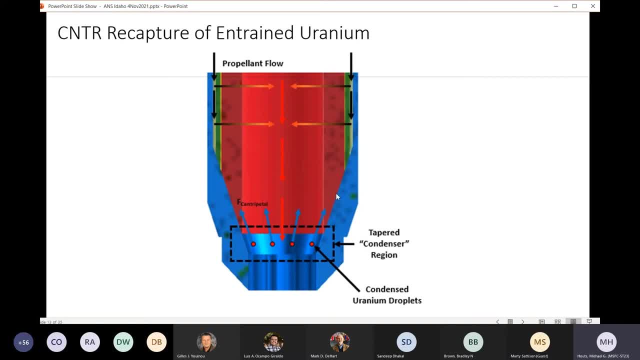 You know calculations need to be to be done on that, the- and I should mention we've got some really good work on MIT and Penn State and Michigan. We just got a group at the US Naval Academy, which is kind of fun because this is. you might've noticed, there are some subtle differences between this and a submarine reactor. 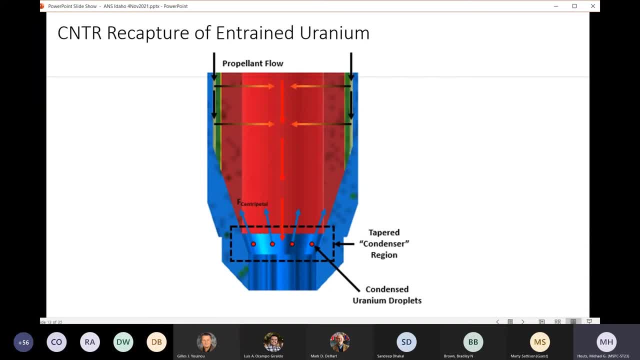 And so, but they're they're having a lot of fun with it. So again, but right now it's mostly just a university level efforts- Ohio State's doing some really good work for us. Okay, So I want to say so. here are the potential benefits. 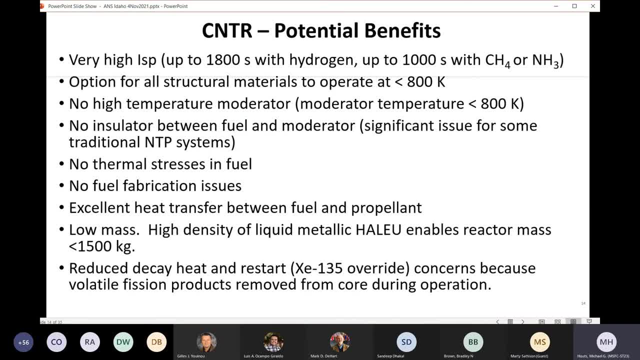 We had the, the ones that we mentioned up front, where with hydrogen it looks like you know, we should be able to get up to 1800 seconds specific impulse- If it all works, a lot of engineering and required- and then a thousand seconds with methane or ammonia. 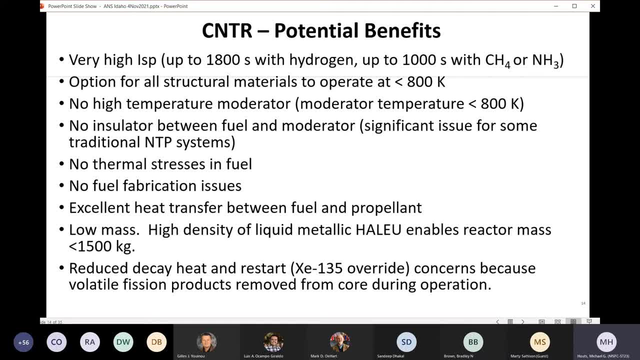 We should be able to keep all the structural materials- moderators, you know vessels- down below 800 Kelvin, The limit there really is. if we're, it's going to come down to how much of our energy Gets deposited in the structure, and the moderator, you know nozzle things like that. 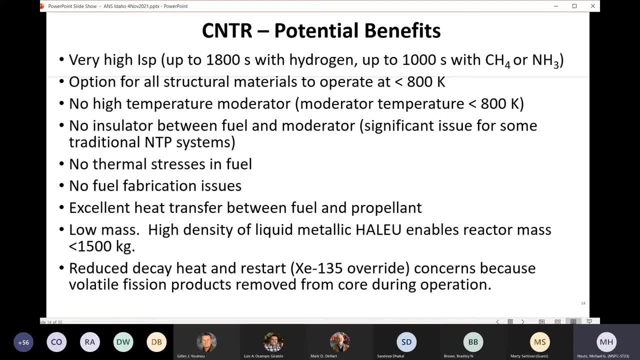 If we- yeah, so say we. if we assume, say, 10% of that energy gets the 7% of the reactor energy gets deposited in the, in the those materials, then it's, it just comes down to an energy balance. 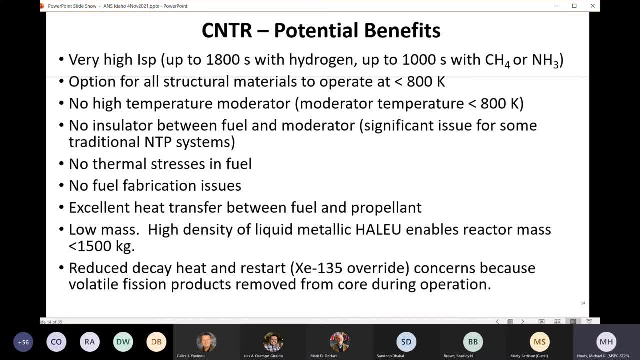 What would our inlet temperature of the cylinder be if you only have 90% of your energy left and you're trying to get to 5,000 Kelvin, but right now it looks. the energy balance looks good for staying quite a bit below. 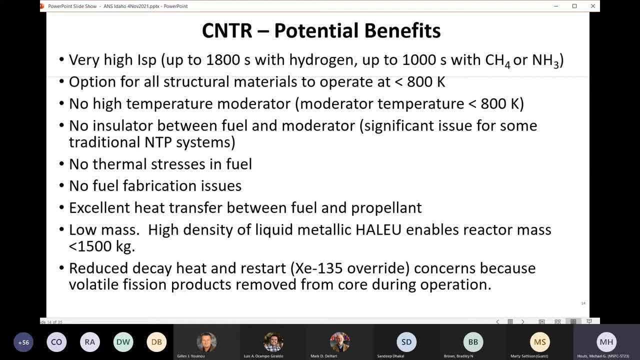 800 Kelvin, and so of course that gives us good moderator capability. We would probably use a zirconium hydride moderator, and there's some talk you know about using just just some low enriched uranium or even depleted uranium mixed in with that zirconium hydride, to keep our moderator temperature coefficients the way we want them. 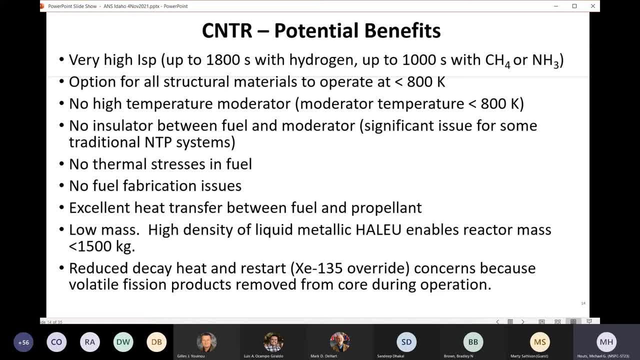 And that was some work Penn State had done, some neutronics and it's kind of like like any other Reactor, Where you have your moderators completely external to the fuel, you can end up with a positive moderator coefficient. So they were looking at some ways they can. it looks like we should be able to set the moderator coefficient. you know, you know where we want it. but again that goes back up to that top one. 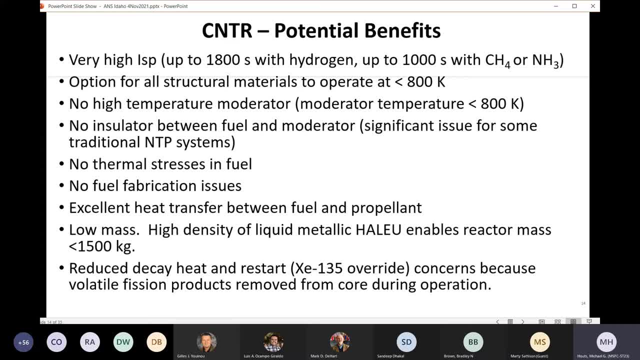 We can't, we can't give too much fissioning going on in our moderator, because that, might you know, then that makes our- you know, our overall structural temperatures higher. So that's the balance of it. So far. that looks really good. 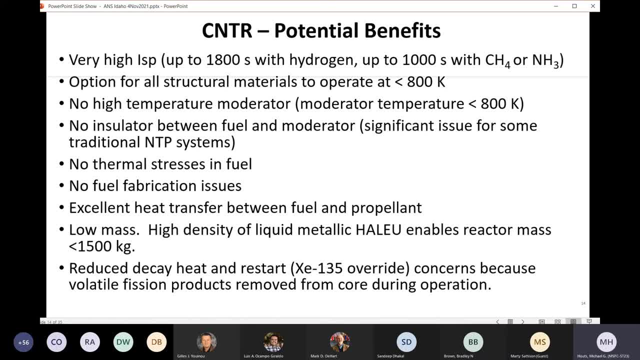 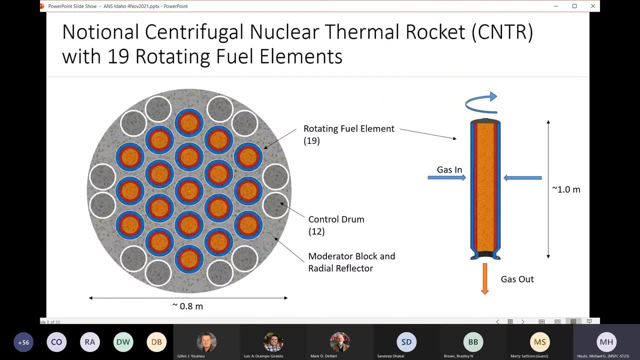 Now these next ones And these are so we don't have an insulator between the fuel and the moderator. and so if you can see how these, you know, the cylinders are set up because there's a gas. so this gas and this inlet plenum, this blue area, the moderator, which is going to be out in the gray region, it sees that same inlet plenum gas. you know that's also, you know, actually getting pushed into the rotating cylinder. 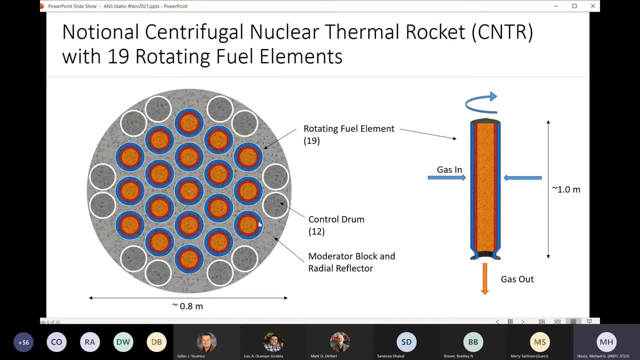 So essentially this is isothermic, So it's not going to be as thermal. In other words, this surface here is going to, you know, be very close to the same temperatures as this surface there, and both those temperatures again would be below 800 Kelvin. 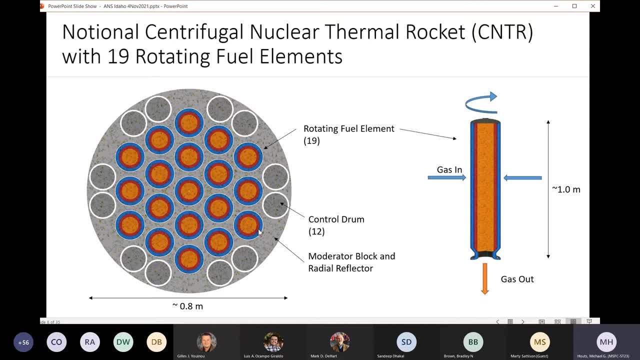 So we don't need to have an insulator between the fuel and the moderator, And that can be an issue with some solid core concepts. Now the trade is we are using up a little bit of core space, you know, because now you have to in your core, you've got your inlet plenum. 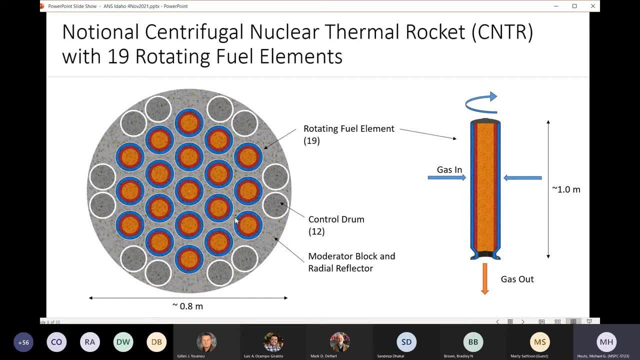 And so that's so. there is a trade, trade there, but that is a, you know, a potential advantage is just not needing to have an insulator between the fuel and the moderator And the uranium metal- liquid uranium metal, you're still. 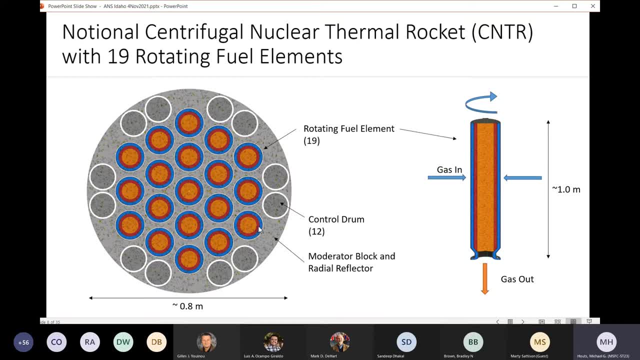 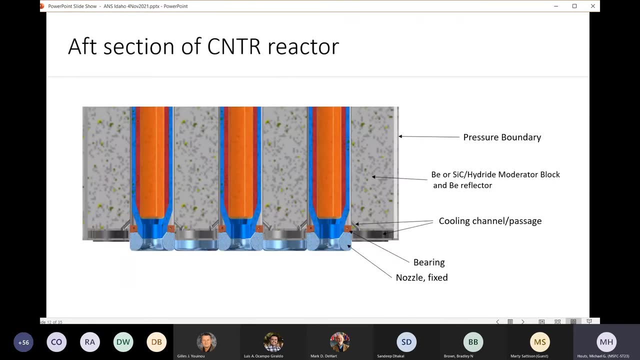 up around 15 grams per cubic centimeter density. so you still, you know, that kind of compensates for this little bit of extra void that you have in the core, And so I think I mentioned that down here some ways. There's a okay, this one's kind of tongue-in-cheek, but there's no thermal. 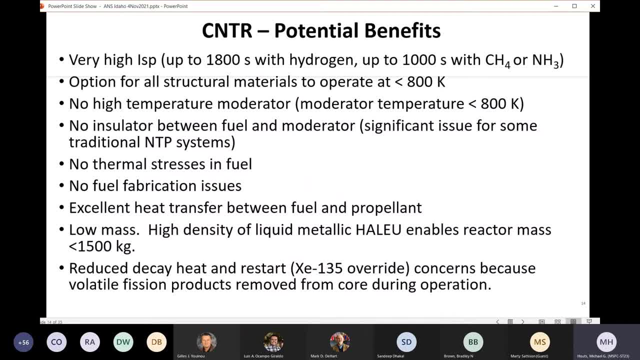 stresses in the fuel because you're a liquid, you know. so you don't have to worry about the thermal stress in the fuel. That's one issue. That's primarily a test issue. right now for the solid core systems We're looking at trying to run about five megawatts per liter and you can. 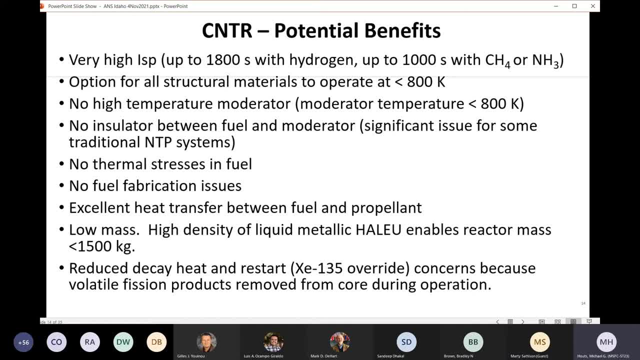 generate some significant thermal stresses in the fuel, but it's very hard to test. There aren't- yeah, it's just very hard to get in a test reactor that we can generate five megawatts per liter in our fuel, especially you have some of the higher temperature. 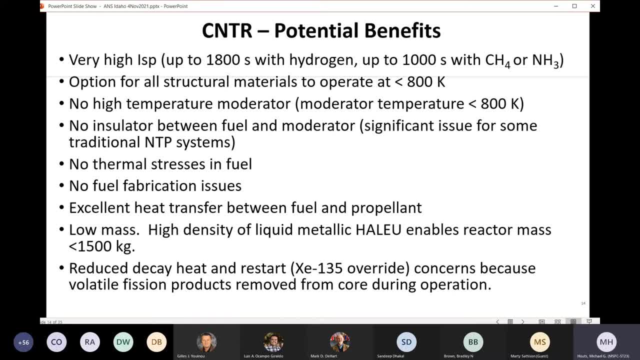 fuel, and so that's one issue. So I think that's one issue. fuel forms where your uranium loading might be down a little bit, and then also the fact that we're trying to go to high-asset, low-enriched uranium. I should mention that all these numbers 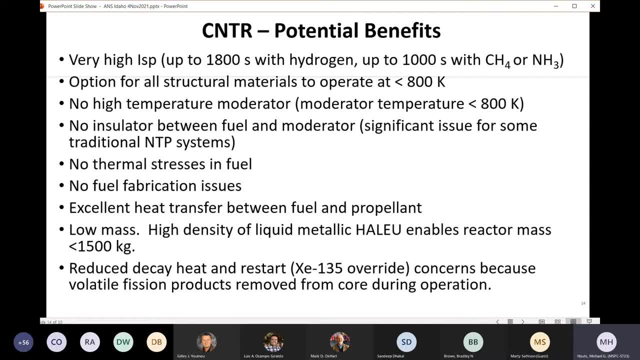 were also run using 19.75% enriched uranium. And then this one's even more tongue-in-cheek: no fuel fabrication issues, because basically we're just loading a metal into these cylinders. You do have really good heat transfer between fuel and propellant, and that's. 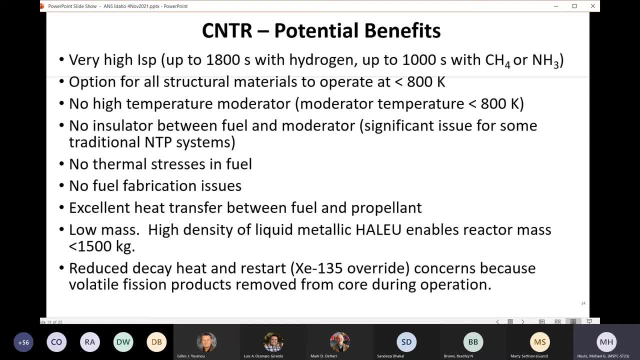 been verified primarily by UAH, but other universities have verified that Low mass, the high density of the liquid metallic helium. It looks like Michigan did a lot of these numbers- University of Michigan, and they were coming in, I think, like 1,300 kilograms. 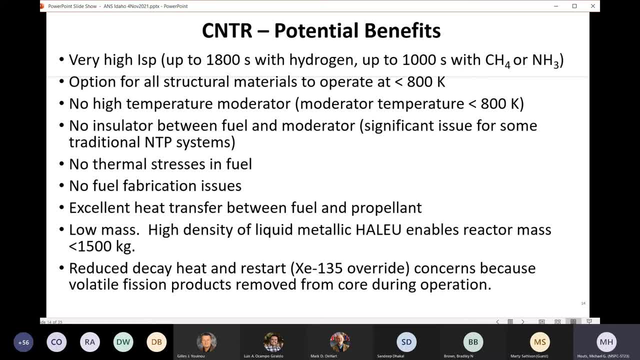 but that's just for the reactor. You also have a lot of other things on the engine, but that's a good, reasonable number. And then reduced decay heat and restart. Okay. so now this. to me this is the classic turn a bug into a feature. But you know we will. 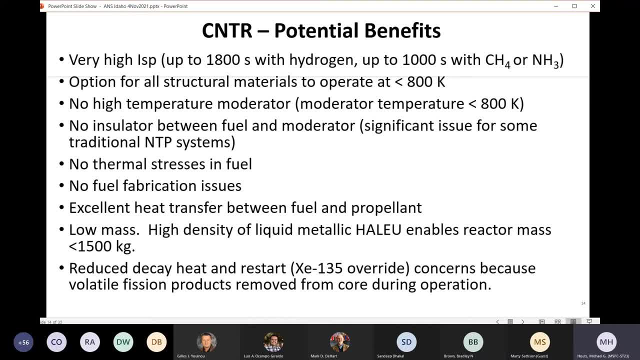 be losing volatile fission products, you know, through the nozzle And so the. but the potential advantage of that is by having all the a lot of the iodine basically leaving the system during operation. then we don't have the xenon-135 override if we did shut down and want to restart. 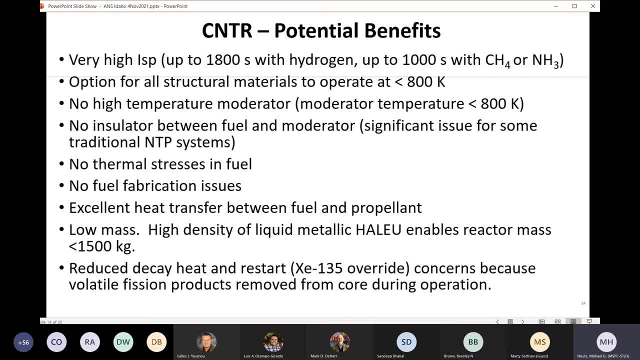 And that's usually. that's if you want to do, say, multiple perigee burns or some of the you know types of missions that people talk about And so, so that's an advantage And you actually do, depending on how we set it up. that should also reduce our decay heat removal issues. 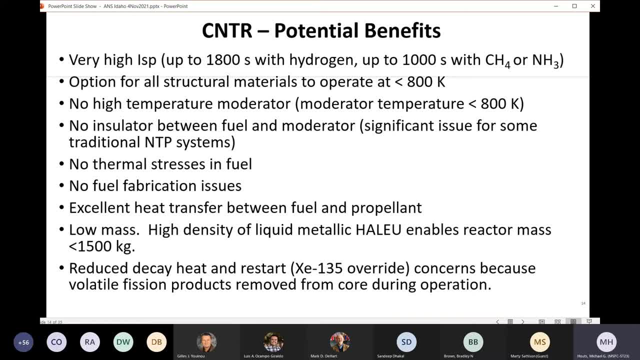 in the system And the, and then just the kind of the dose to the astronauts. Right now we plan on having the hydrogen in the propellant tanks or whatever the propellant is. if we go with methane or ammonia, That's provides a lot of shielding And then, but we're still planning. 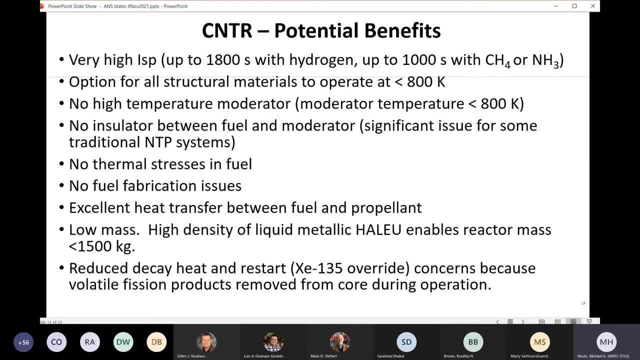 to have the astronauts in there, Basically in their solar flare storm shelters, so basically in their radiation shelter during the burn and then for a while after the burn, And so so, basically, if we any of the fission products that 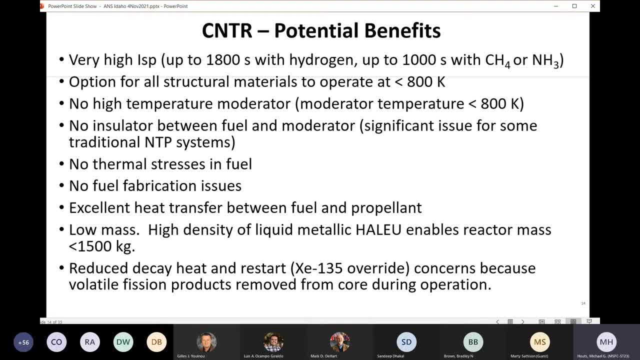 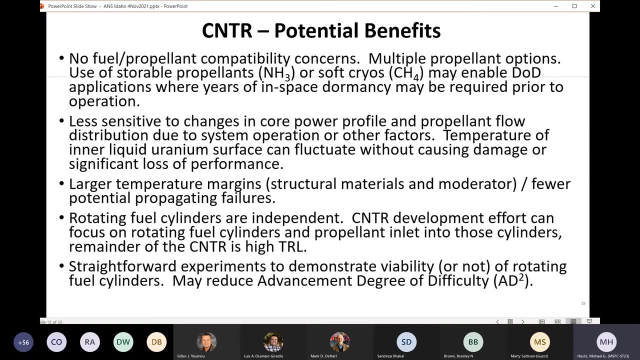 are removed from the engine during operation actually does it does help us from that standpoint. also, Other potential benefits. this is one. this really goes back to the, the storability. So you know your classic DOD application. you basically you how to phrase it. a lot of times people say it's if you never have to use them. 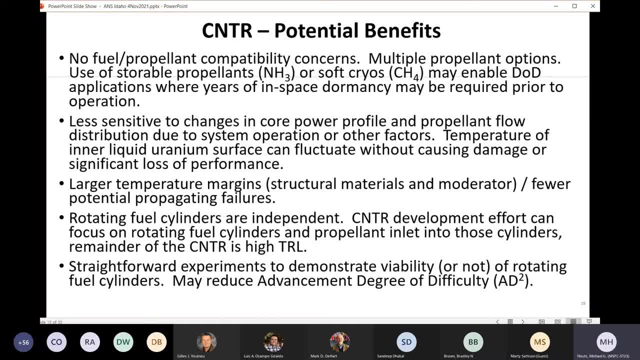 that's, that's the best you know, best thing that you know, best outcome you could hope for, But if, but, you also need to. if you do need to use it, you need to make sure it'll work. 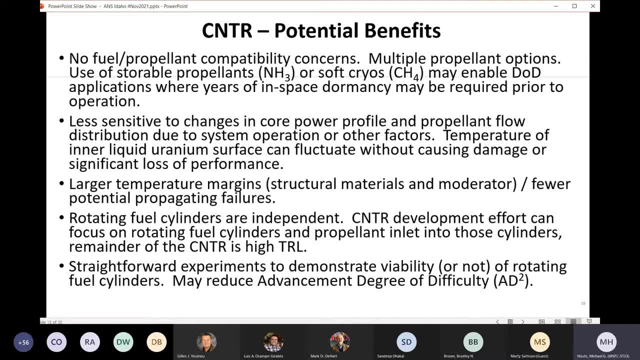 And so say there was a DOD application where you had years of in-space dormancy but you still wanted to make sure that you could go someplace quickly if you needed to, Then if we did use ammonia or methane propellant, that's just a lot easier to hold onto, and especially 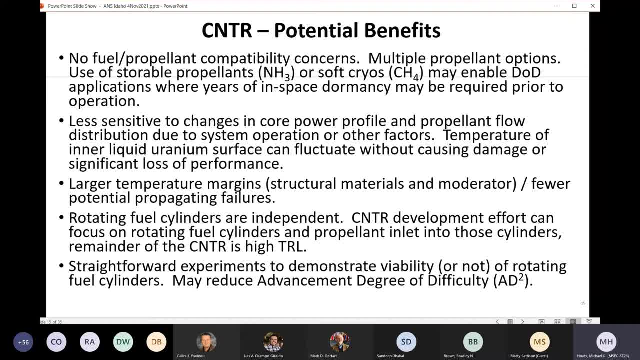 ammonia. I mean it's just, you don't need cryo coolers. I mean you just sit there, you know, totally, totally quiet for years, you know and it, it, it just doesn't go anywhere, which is good. 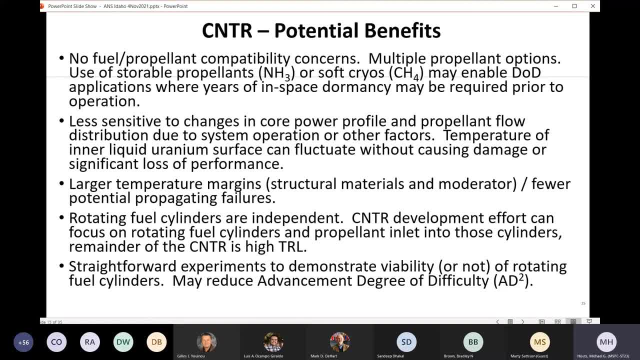 And so that's a potential application. It's also- I mean it's- a benefit for NASA missions, because when we're, if we're, assembling close to Earth, you do get enough Earth shine, that'll. that'll start to heat up your propellant tanks, But it's. 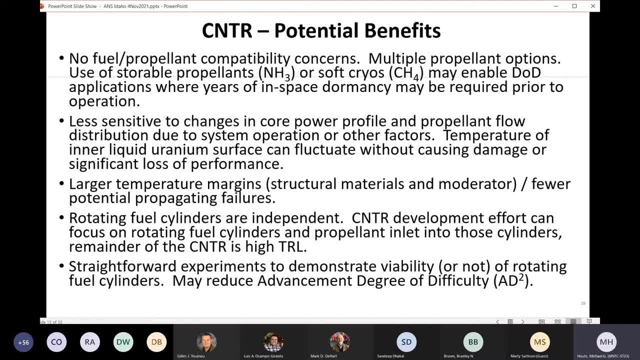 it's possibly a you know larger, or you know just whenever the system needs to be dormant in space for a long period of time that you could almost envision. you know even down the road. you know propellants pre-deployed around Mars. 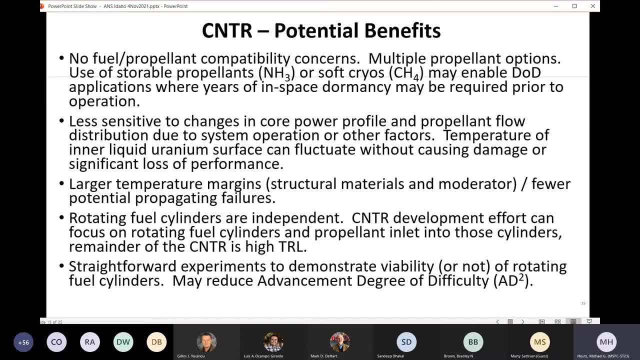 that's just available for use. if needed, Then again that's probably way down the road, but it's just a potential benefit. The less sensitive changes in core power profile and propellant flow distribution. So this is a- this is kind of relative to a solid fuel system. 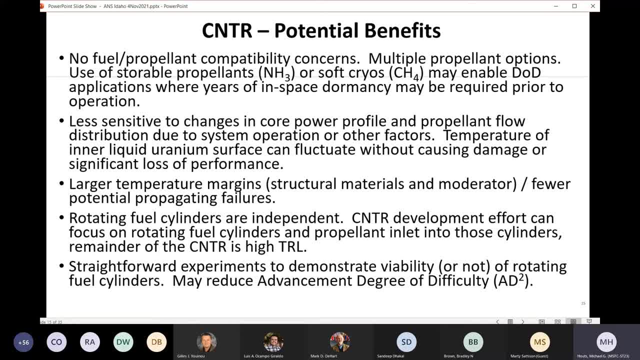 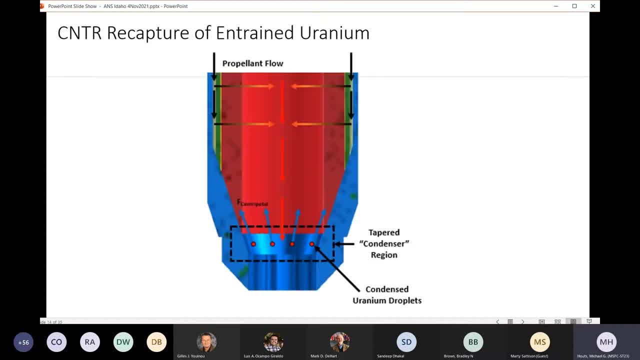 You know, for example, you mentioned, you know, a lot of times the designs. I can't remember if we have a, I might not have put a good schematic in here. Okay, so you know, this is kind of your standard. 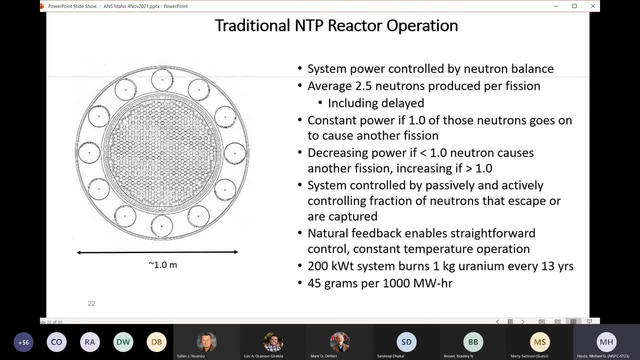 NTP core. You see the control drums around the the sides of the core and that's, of course, how the system's controlled. We try to keep you know, minimize the in-core control, And so you're controlling with these controls, you're controlling. with these controls, you're controlling. 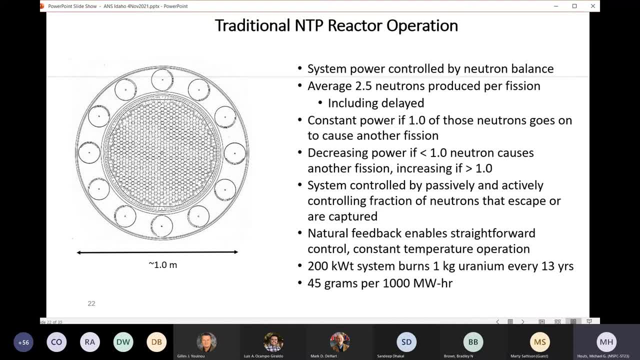 with these control drums. But you know, say we have a control drum get stuck, then you'll end up having a little bit of power tilt in the core. And so you'll say you'll say this one got stuck with its absorber in. well, the power's going to be depressed a little bit here and then we might. 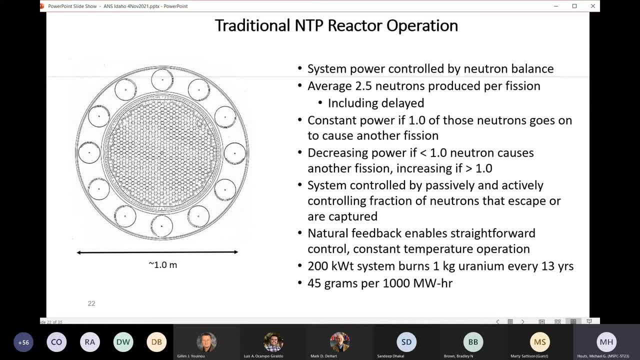 have to compensate by adding a little more reactivity over on this side, So you actually end up with a little bit of a power tilt, And so, to keep the same specific impulse, this fuel would end up having to run hotter on this side, or you because you'd be at a higher. 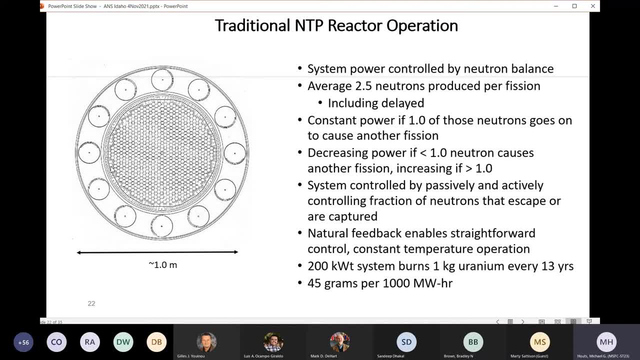 power on this side than you would on this side and it's hard to control. you know flow to each channel, So you start getting into complexities like that. or you can have- you have, say, your flow distribution system. you can start to. you know just changes in the flow distribution about. 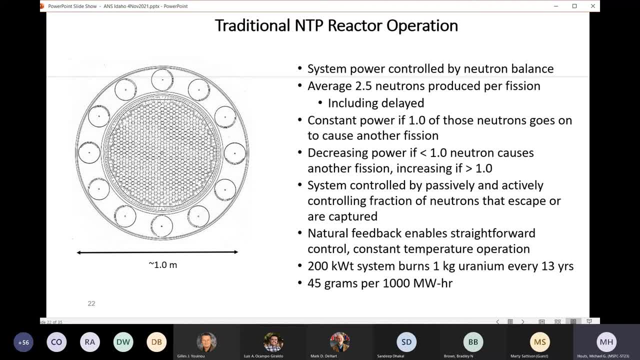 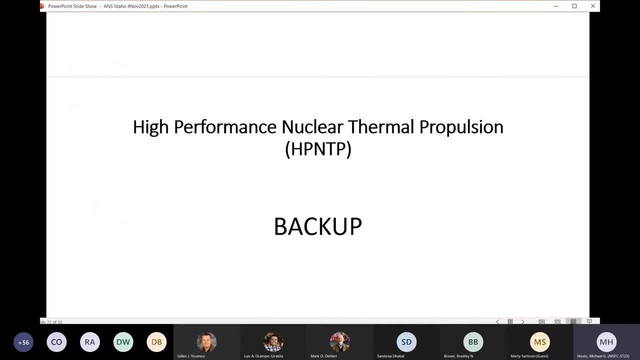 the core. So those are, those are things we're dealing with and we're, you know, working with on the solid core systems. But you, you end up you know you don't have that as much as the liquid. If, say, on that inner liquid surface, say, parts of it are at 55,. 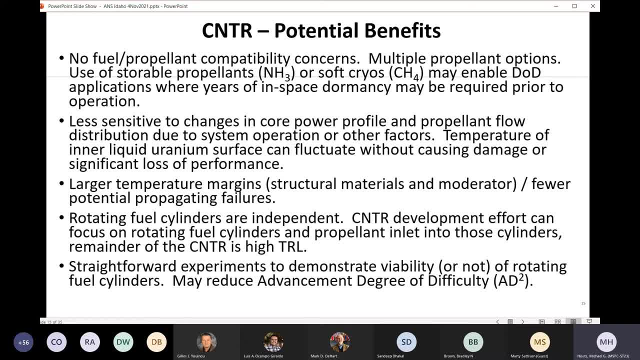 500 Kelvin and parts of it at 5,000 Kelvin. just based on these changes, it's really: yeah, you're not generating thermal stresses. Yeah, there's going to be some second order issues, but that's a again a potential benefit. I do have much larger temperature margins in the 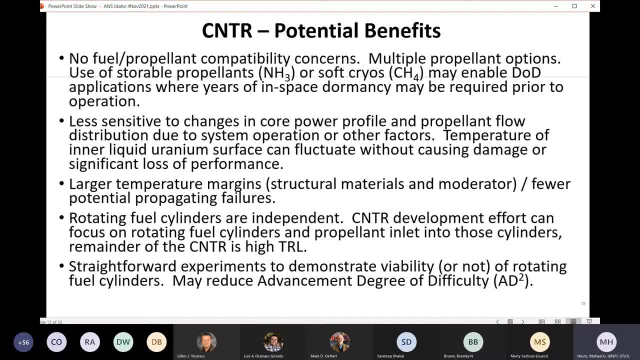 liquid fuel system, and that's just because the structural material is a moderator. We should be able to run very cold. So there's no high temperature structural materials, no high temperature moderator, and there seem to be fewer propagating failures. And then the rotating fuel cylinders are independent, And so ideally, if we can get one, 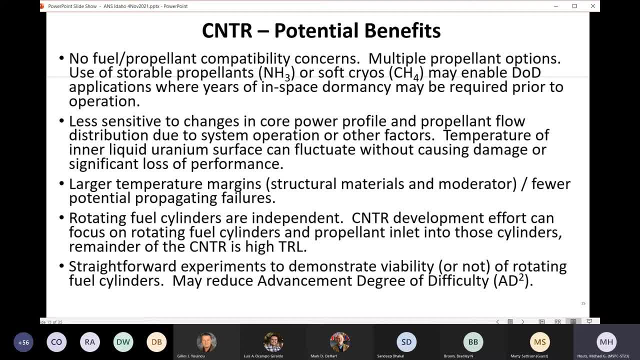 fuel cylinder working and that could be a test, one of the concepts we're thinking about for the. I think I saw Katie online, but you know there's talk about a smart reactor, you know, just a reactor that would basically be testing fuel elements, And so this would be, you know. 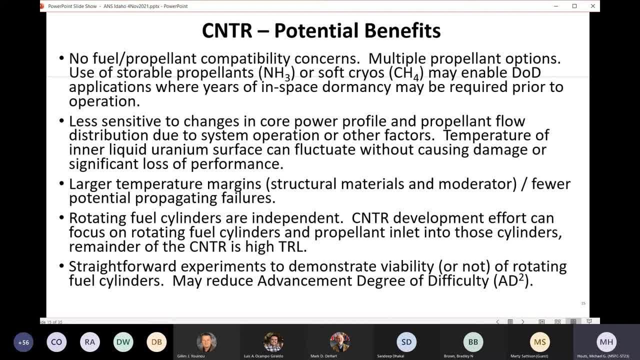 we would basically, in this case we would test the fuel cylinder. If we could somehow work out all the bugs on these rotating fuel cylinders, then they would, you know, they would, you know, typically be independent and nearly identical. And so that bottom bullet, you know that would be. 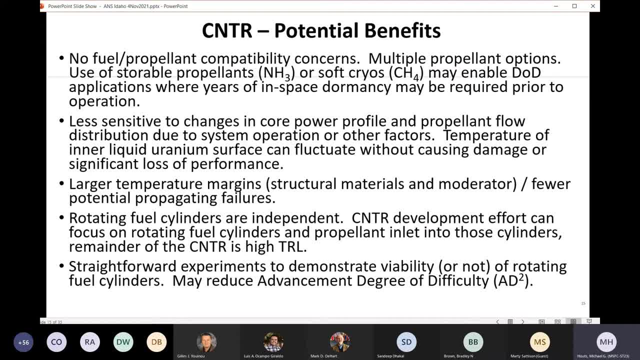 one way to try to reduce this advancement degree of difficulty, because we could really focus on: okay, how do you make this fuel cylinder work- And you know the idea- like a smart reactor or some other reactor that's really set up for, you know, doing tests related to space nuclear. 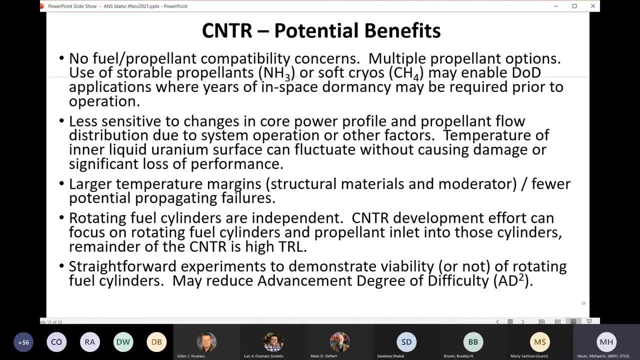 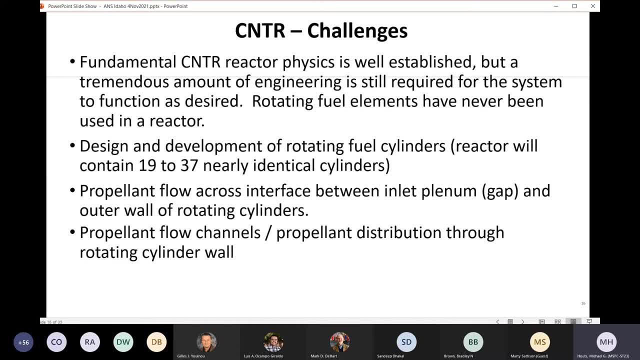 propulsion could be, you know again, hopefully directly applied here. Now the challenge is- and there's a lot of them, you know. so the physics is well understood, but we- I mean just in a nutshell, you know- we've never used rotating, to my knowledge. and boy, if someone. 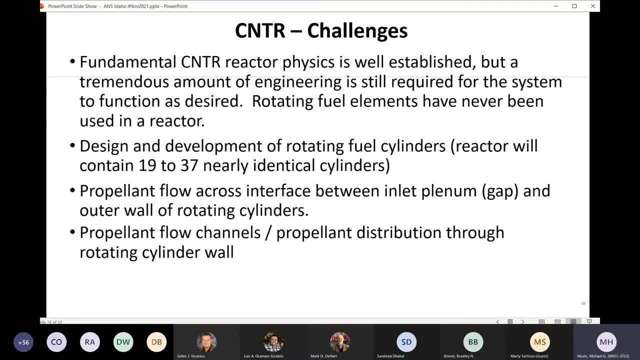 online knows different, because we did all kinds of you know fun things in the past, but to my knowledge, we've never used rotating fuel elements in a reactor, And so usually when we've never done something, that's when it looks the best And so we really need to. you know, okay, what are. 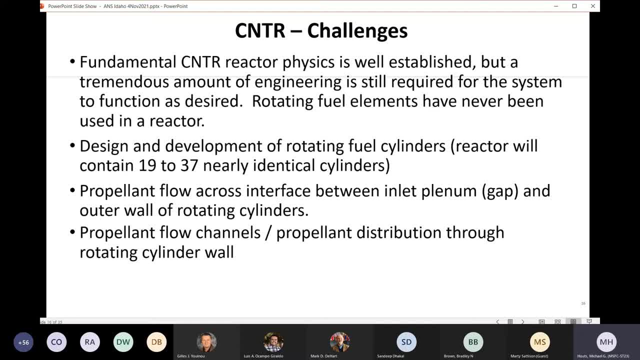 all the. you know, I don't know, we've never done something. that's when it looks the best And so I don't want to say nuances, but you know what exactly does that, you know basically. 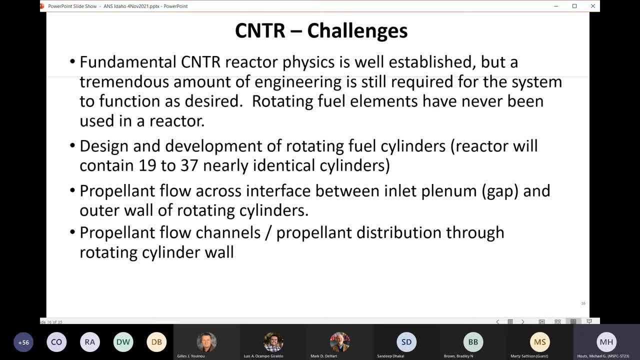 what effects could that have? And so really the challenge is really just the design, development of those rotating fuel cylinders So you can see, you know, for example, the fuel, you know with the propellant going through the fuel you know there's going to be, you know it's not just going. 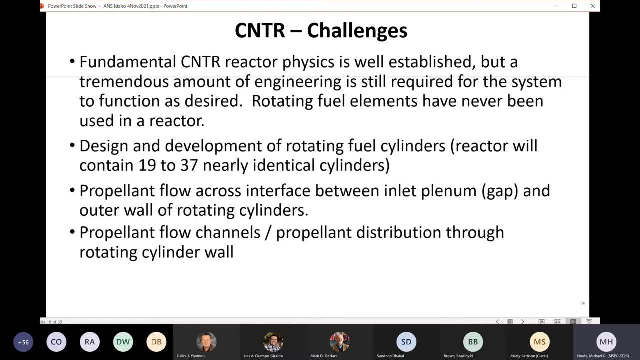 to be this constant. you don't want to call it benign, but you know, just you know you're going to have a lot more dynamics going on, So you'd have, you know, bubbling through this fuel. the fuel is going to be moving around some within those cylinders, And so the question is: 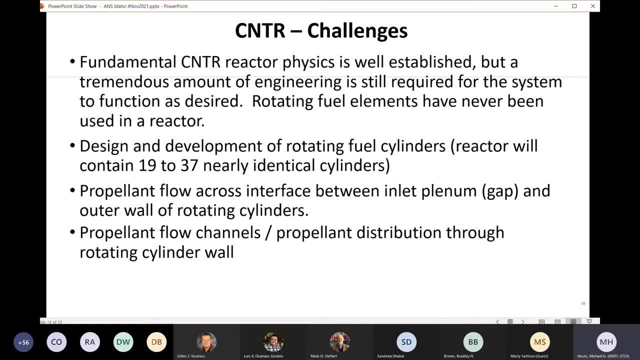 how do we make sure that that's stable? Do we need to just to make things you know, statistically, I'll almost say wash out? do we need, you know, more than 19,? do we need, like 37 cylinders, Some? 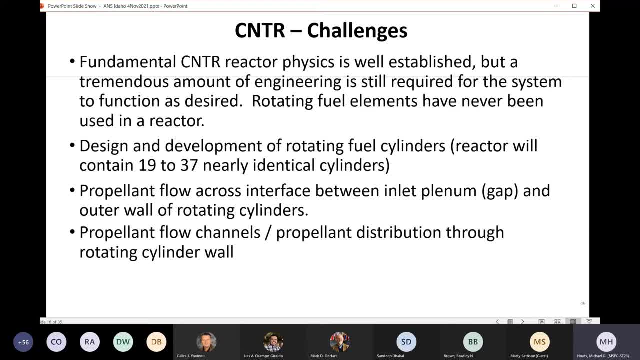 of the concepts in the 60s, they were, I think, over 40 cylinders, And so that's something that needs to be analyzed. But the you know, just to, you know, like, and that goes back to like, 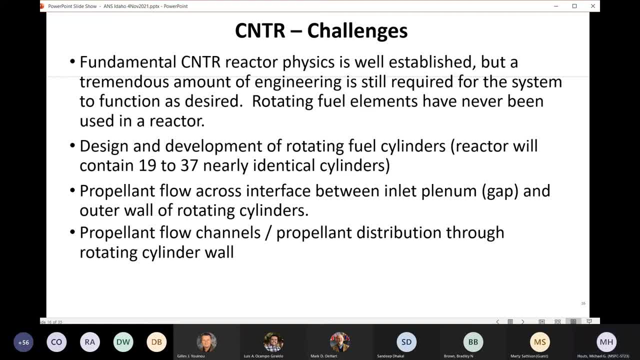 how much you know depleted or low enriched uranium do we need to add to our moderator to help stabilize the dynamics of the system? So those are all things that's going to be mostly calculational, of course. to start with, The propellant flow across the interface between 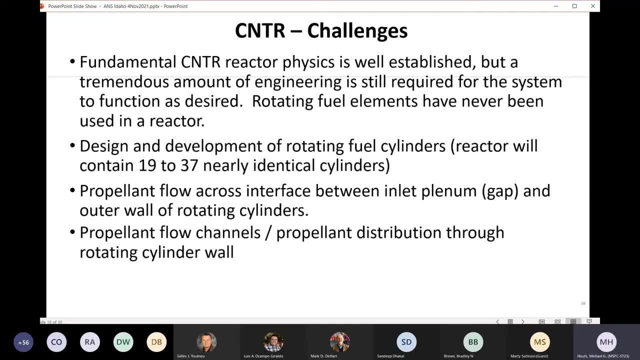 the inlet plenum and the outer wall of the rotating cylinders. This is one the university professors are just loving, because you know I've got this hydrogen and I'm trying to bleed it in. you know, probably you know millimeter or fraction of a millimeter diameter holes that 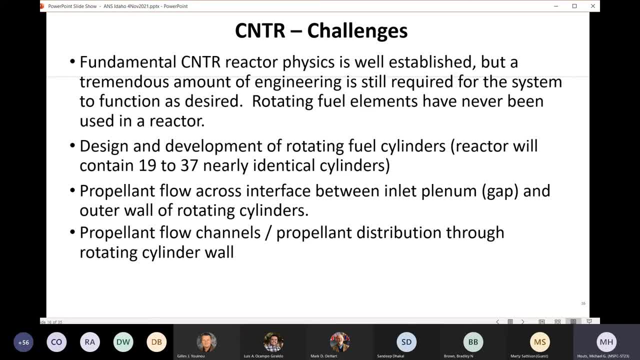 are kind of perforating this whole cylinder, you know. and how do you model that? What equations do you use? And so I'm joking, I say they love it because they see a lot of students being able to get PhDs out of that. Then the you know again, just flow channels, propellant distribution. 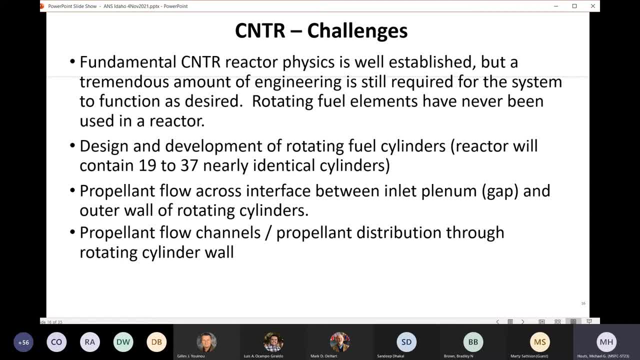 through the rotating cylinder wall. how do we manufacture those? How do we make sure they can handle? you know one thing is what if you accidentally freeze the engine? So what if you have some liquid uranium metal starts to get pulled back into one? 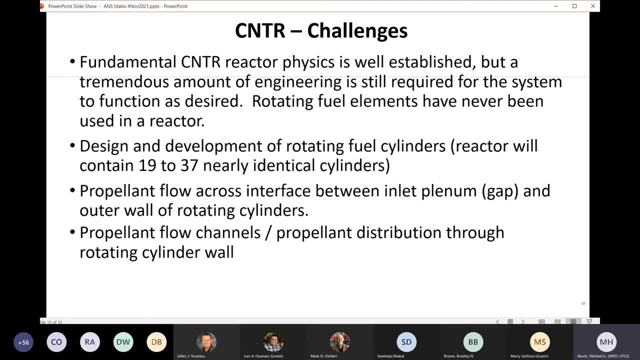 of those flow channels and it freezes. Well, it should melt fairly quickly because you would have blocked your coolant and it's going to be fissioning. But you know how many times can you do that before you start to really road that? you know the wall of that cylinder. So I mean. 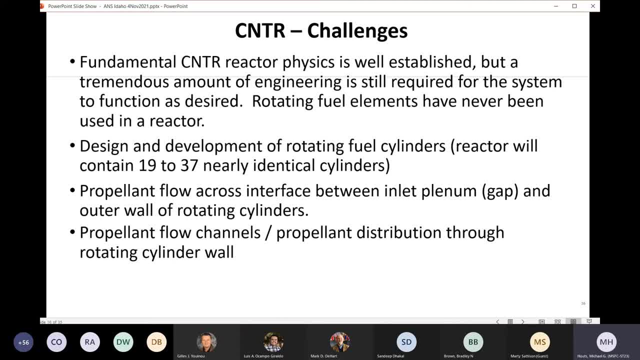 just all kinds of things we're going to need tested and calculated. The drives, like Gilles mentioned, you know how do you. you know what's the, you know drive turbine design, you know the design and what you can do with the drives. So what's the cost and how do you use them? 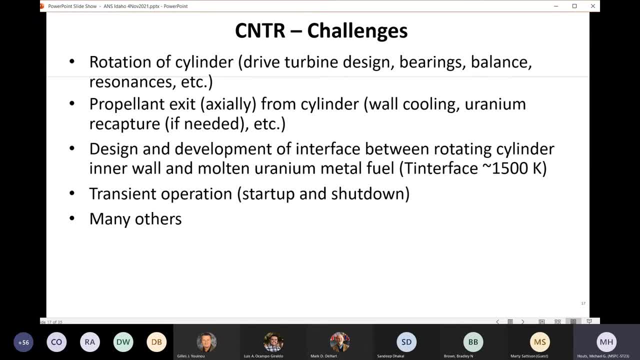 Do you have any recommendations to the next slide? To start with the concrete: the parts do you, you know? do you start with the parts? you know? the uh, uh, you know? drive turbine design in more detail, the bearings, balances, uh, resonances, one of. 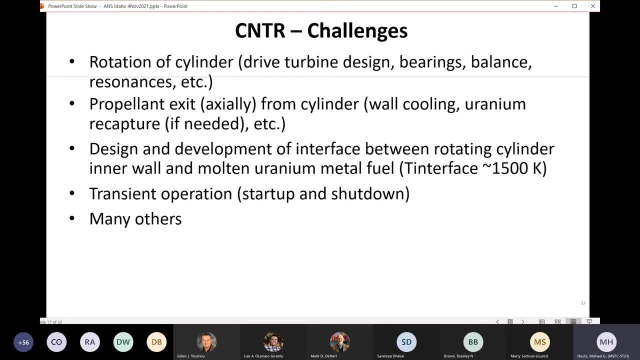 the reasons the chemical rocket engine guys don't like us. taking 30 seconds to start is uh if, depending on how we're running our turbo pumps, you can actually get resonances that can be really hard on the turbo pump. so how do we design the cylinder so you can go from zero to, you know, 5000? 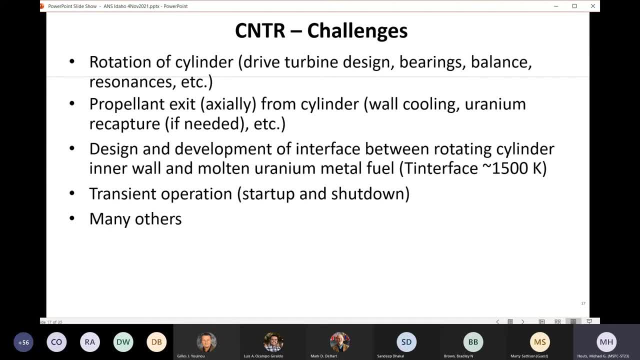 rpm, you know, or whatever. we end up needing uh, but avoid resonances and you'll make sure that's um, uh, yeah, holds together well. the uh propellant exit from the cylinder. uh, everything from wall cooling to uh, you know, especially to run at the higher temperatures. you know, the uranium recapture. 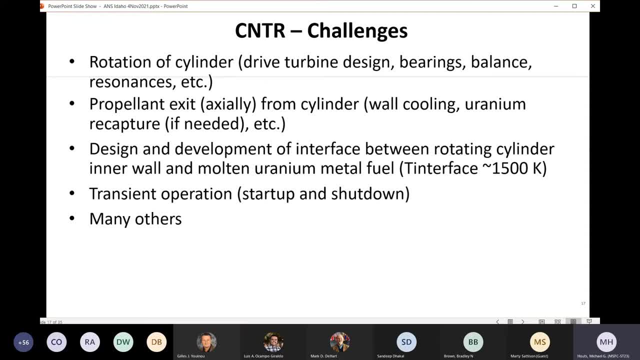 things like that. um, the uh, just the interface between the rotating cylinder inner wall, the molten uranium metal fuel. wanna again, we'll have a higher pressure driving propellant through that wall, but we don't want to. um, uh, yeah, but there's just. there's going to be some other effects if we 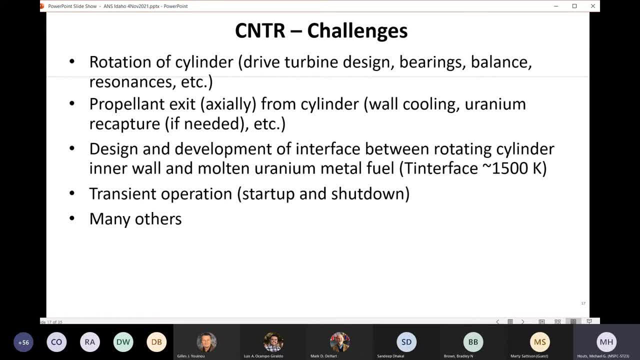 if we do, you say, a silicon carbide cylinder with a zirconium carbide layer on the inner surface for compatibility, you know what's the best way to manufacture that? i think it's one of the ohio state guys is- is looking at additive manufacturing. uh, yeah, trying to do that with additive, but uh. 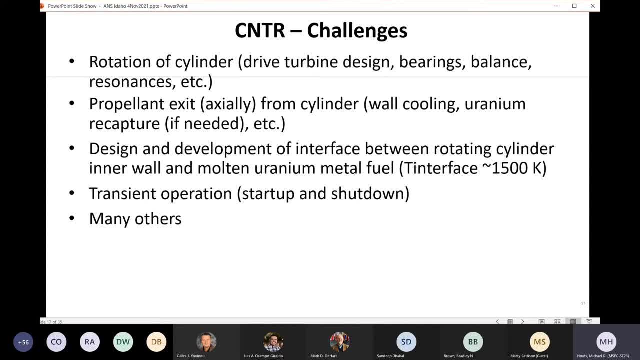 you know. again, that's something we would need to prove. uh, transient operation: start up and shut down the? uh, yeah, of course, the general idea is: you, just you, you know you start, you melt the fuel, you know, at a very low propellant and you spin up while the 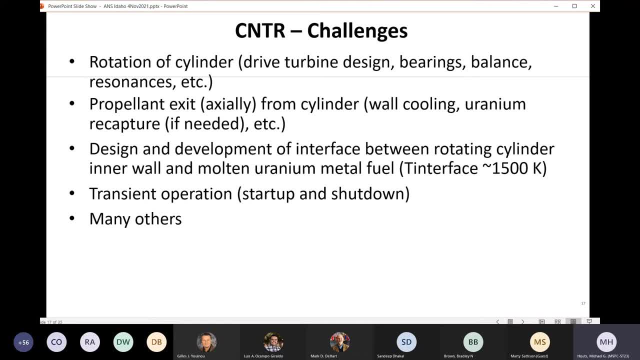 uh propellants being increased and shut down, you uh essentially turn the engine off and you keep spinning until the fuel solidifies and, uh you know, depending what your decay heat removal requirements are, that could get more complicated. so a lot of uh transient operations and and then 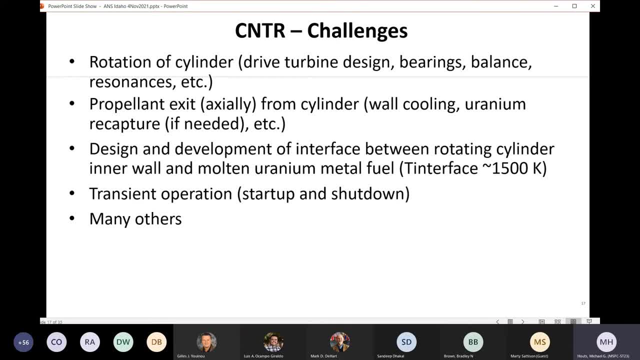 you know, many others uh, beyond that. so again, lots of uh potential challenges to making it work. um, and so again, i'll just- i'll leave this up on the screen again. just going back to the goals, the other thing i should mention is no one is at all- uh, you know- wed to this particular. 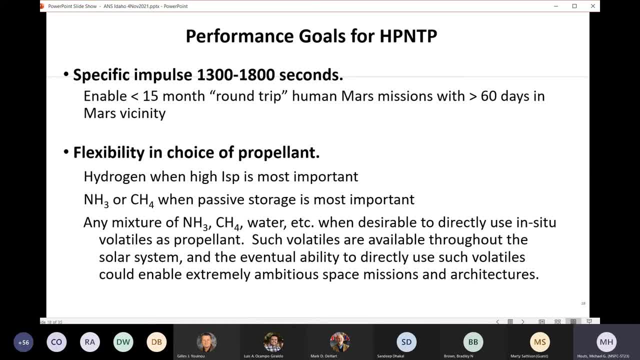 concept, it's just one that seemed like it was good work done in the 60s and a few people working on it now, and. but it just gets us into this range where if, um, if we were able to develop this type of system, then, uh, it's just like everybody's all of a sudden excited about space nuclear. 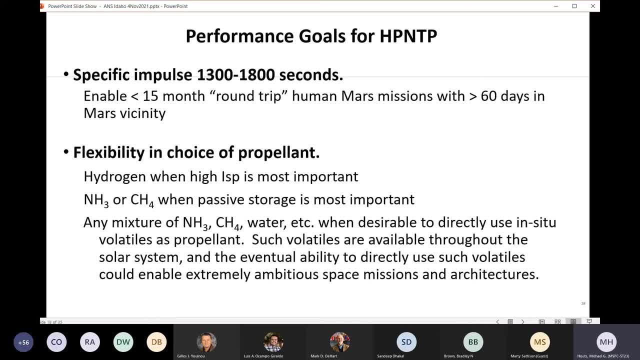 propulsion, just because of what it would enable and so uh. so you know that's kind of the carrot. and then it also has just some other advantages for, uh, both nasa and dod missions, as far as being able to use more storable propellants and then going far future. 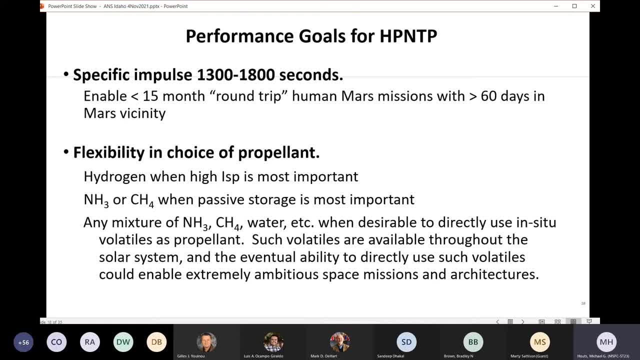 it's amazing what you can do with a system that can use um, basically use volatiles that are um found in space. now, oh boy, i really bet i might have the name wrong. they might did anybody know. uh, i think it was tony zapero at, i know. 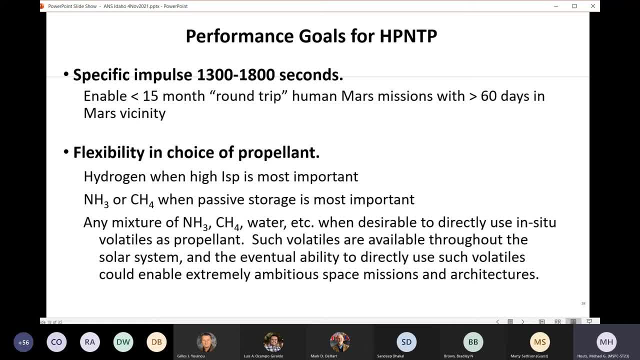 it was a long time ago. he was there probably 20 years ago, but i might have the name wrong, but anyway, he was showing uh everything from. uh, you could even uh move kuiper belt objects around you, could, uh, you could basically position any object in the 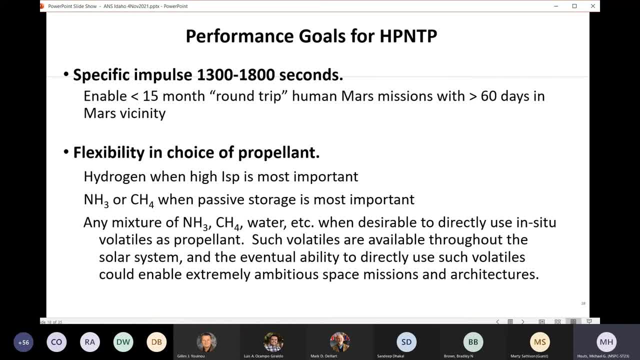 solar system, um, anywhere you wanted it, using, uh, just a small amount of thrust and a, and then gravity assists, and then also you're having propellant depots so you could do very ambitious missions uh, around, uh, yeah, around- the solar system. so anyway, so that's kind of the long term, that's. 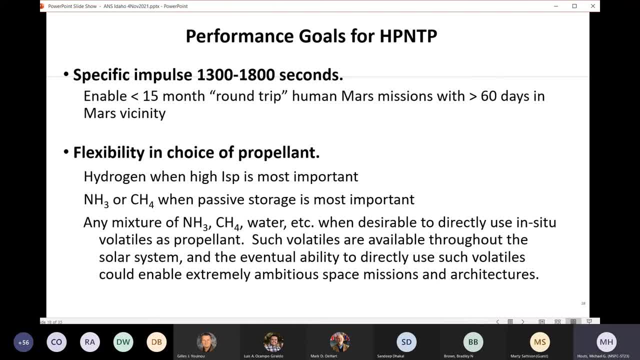 that last bullet. so any uh just, yep, wait, just open it up to discussion, or or definitely go backs, because i know i i sometimes talk a little fast and uh just uh, anything that wasn't any well, any suggestions or any, uh you know, any uh uh, additional concerns or anything at all. okay, i see uh. 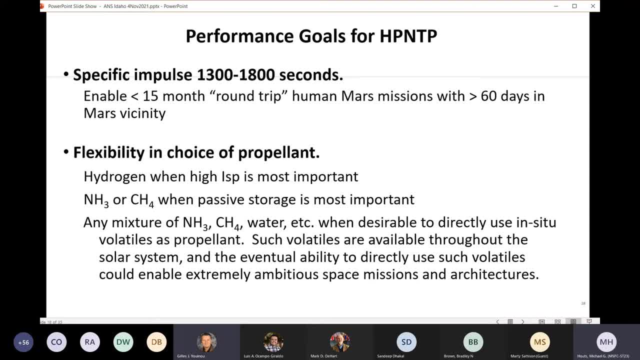 steve reese has got a hand up. go ahead, steve. we're not hearing you. you may be muted. well, steve, it looks like you're muted if you uh have a question. well, steve, it looks like you're muted if you uh have a question. 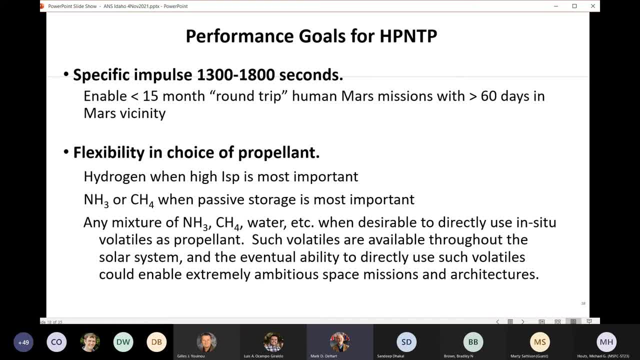 okay, you know, you get your hand up. yep, hey, mike, there's something i haven't seen in the presentation is uh, maybe i missed it, it's the uh. what's the target for the thrust? oh, okay, uh, yeah. so the uh. so right now, that's, we're really going for isp. 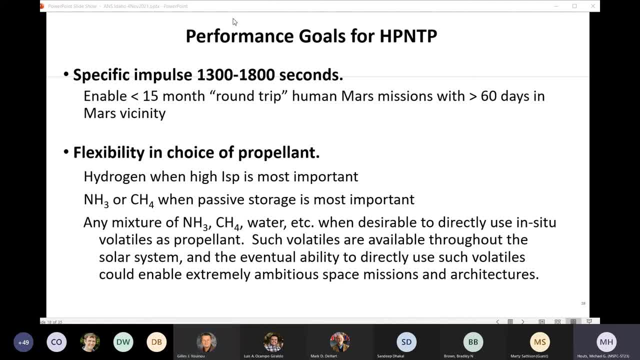 but we're trying to make sure that we can do a few thousand pounds thrust and so, um. so i think where we're setting it, um, i want to say it's 100 grams per second hydra or propellant flow, and i guess the propellant we're using was hydrogen for 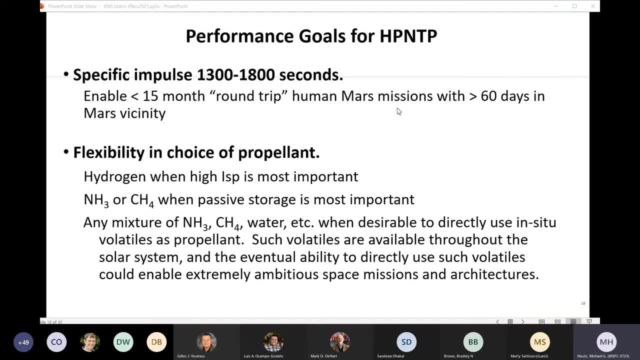 that. so it's 100 grams per second hydrogen flow per cylinder, and so that's kind of the yeah, that's kind of when. when that comes into play, that's what people are looking at. so. So that ends up with a 19-cylinder system. 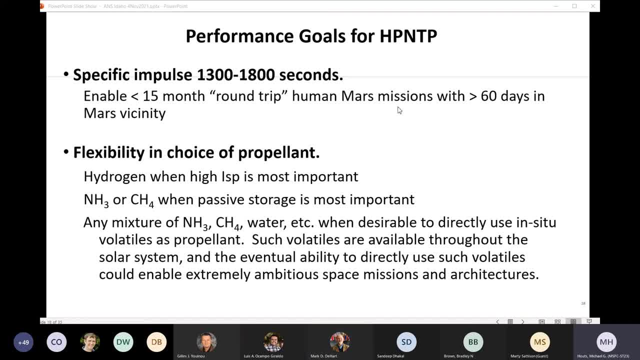 Of course we're trying for double the ISP, so I should be able to do that off the top of my head, But it ends up being a few thousand pounds for us. If we need to go lower, we could and maybe still have some benefit from going higher. 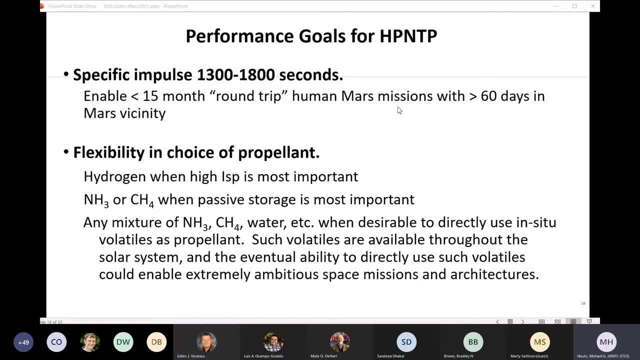 But it's really the high ISP is really what gives us the good performance, or what's most important for the good performance. Okay, so in terms of performance, then it should be compared more with nuclear electric propulsion than standard nuclear thermal propulsion, right? 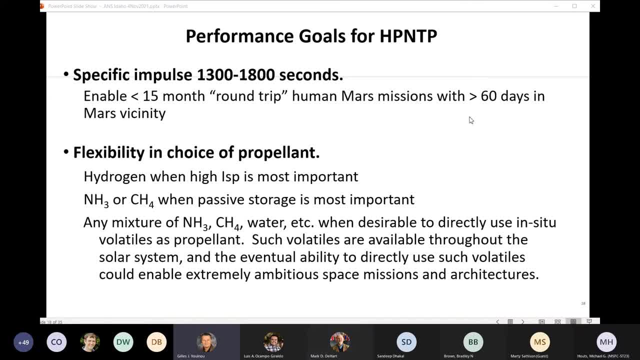 Well, no, it's up in the nuclear thermal propulsion range, The nuclear electric propulsion. well, you're looking at like pounds of thrust And so when you get into that few thousand pound thrust range you can do impulsive maneuvers And you'll maneuver very quickly. 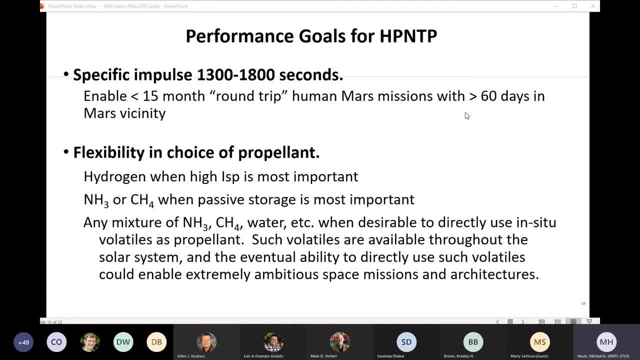 So you're in the but yeah, we would definitely we'd need to start looking at the gravity losses And so, right at Earth, departure, burn, you know, and this again would get into details- We might want to run in a you know like, run extra propellant through. 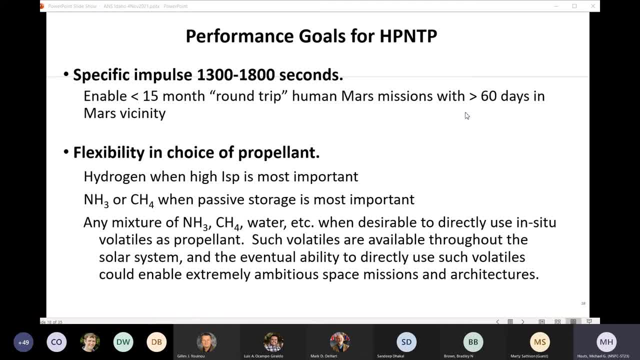 But if we're- yeah, just around, if we're like 5,000 pounds thrust per engine at Earth departure, you know, right now our baseline is we're looking at 25,000 pounds. You know, a three engine cluster. 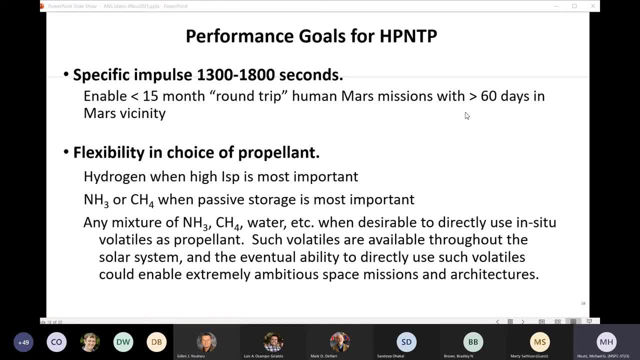 But we don't have. just looking at you know what Aerojet Rocketdyne has been doing. we don't have a huge penalty going down to 12,500 pounds thrust per engine and three engine cluster. So this one, if you know, say we did configure for five but we have the higher specific impulse. we'd have to look at how that traded. 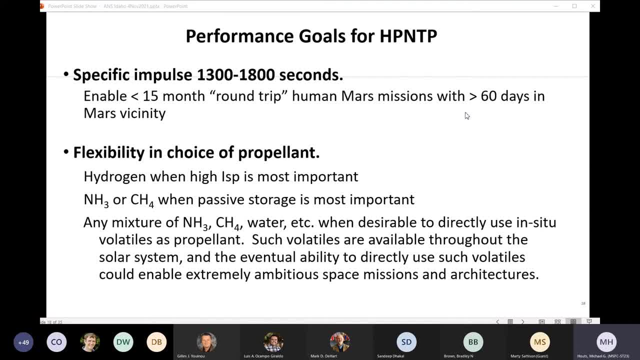 We could go, yeah, we could use more engines or go up in thrust too, But no, we're, but we're. we're definitely wanting to make sure we're high thrust and impulsive maneuvers, not because electric propulsion you can get. 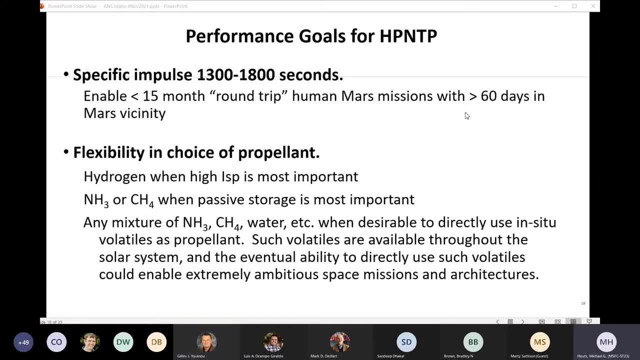 you know 10,000 seconds specific impulse, but you're again just a few pounds of thrust. you know for most of the even a couple megawatt, But in terms of performance? but in terms of performance it looks like it's in between the nuclear electric propulsion and the standard nuclear thermal propulsion. 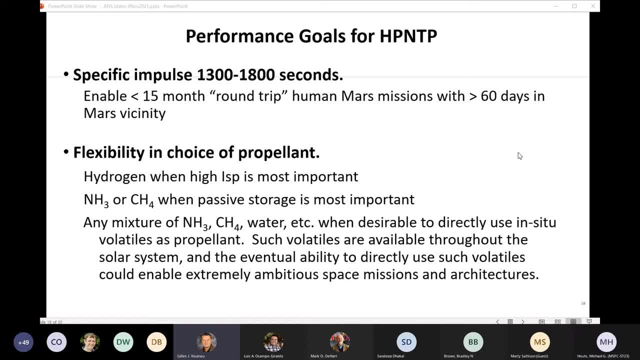 Because if you wanted to increase the thrust of this concept to the same thrust levels, or let's say up to 100,000 pounds, the thrust to weight ratio would not be favorable, would it Right? yeah, the so it's. yeah, essentially it's the specific impulse. you're right, that's down, that's you have almost between like an arc jet and a hall thruster. 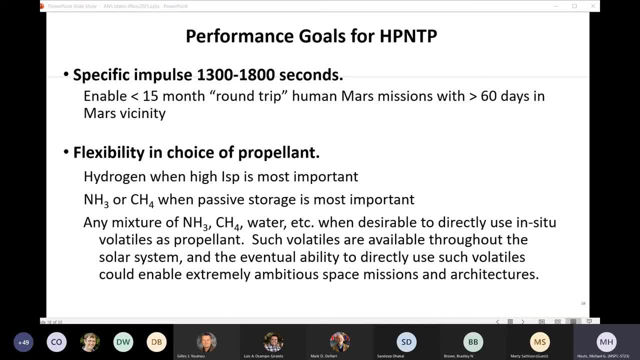 But the idea is is just getting the getting the high thrust you know. so you can do the impulsive maneuvers, And so that's what. so you're in the range where you could still do so it's it's. I'm sorry, but when I, when I say between an arc jet and a hall thruster, you're, that means you're on the low end of what specific impulse you get with nuclear electric propulsion. 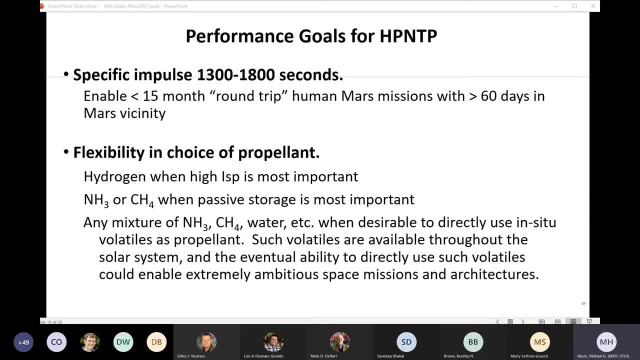 So that's why. but when you're doing the, the fast human Mars missions, then you want to be, you want to be able to basically have impulsive burns, And so that's where we have to make sure the thrust stays up in this. you know, you know safe space. 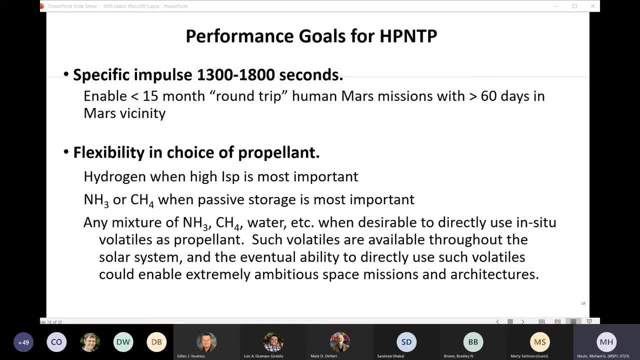 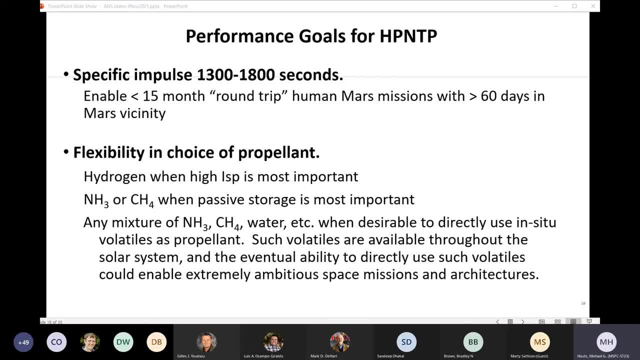 one paper- i think it was ragsdale back in like 1970- um said he could get to mars in 30 days one way. but i want to say he had like a you know like millions of pounds of propellant, you know. i mean it was like he had to really want to get to mars in 30 days, so but yeah, so it's just the but. 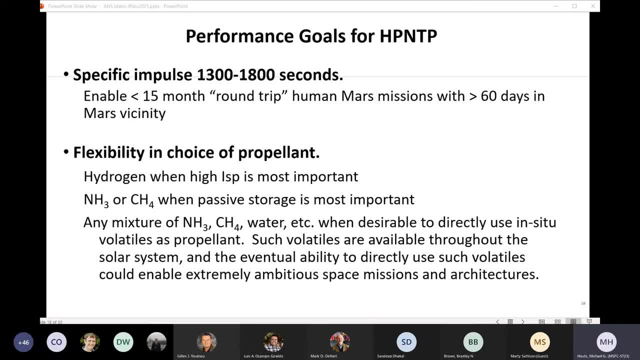 but you know again we're, the specific impulse isn't as high as you can go with an ion thruster or a vasomir or even an mpd, but the uh, but it's just the high thrust is what enables the, the fast trip times. i see travis lang has a question. travis, yeah, thanks, uh, this is really fascinating. i. 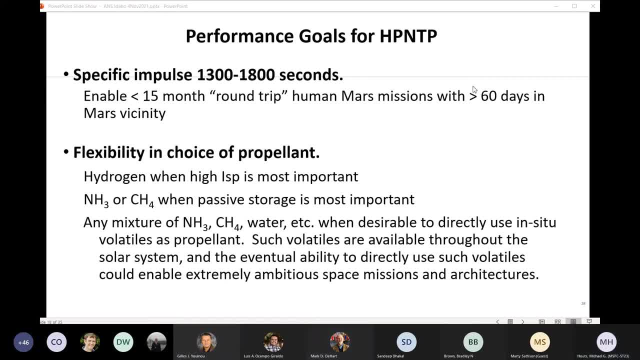 appreciate you putting it on. uh, you, you had spoken briefly about if one of the control drones got stuck in maybe a solid um fueled reactor. what if um one of the rotating, you know, cylinders that has this liquid metal fuel slows down or gets stuck? i mean, if it's the 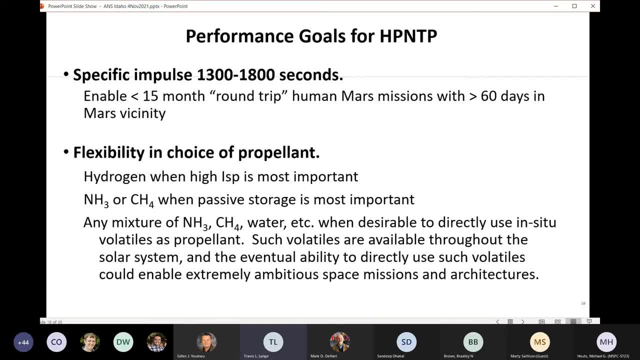 the reactor or the spaceship's being forced away from it, would it all just leak out the back and you just lose that all that fuel entirely, or can you talk to that right? so that's probably exactly what what you said would likely happen, like, say, the uh. 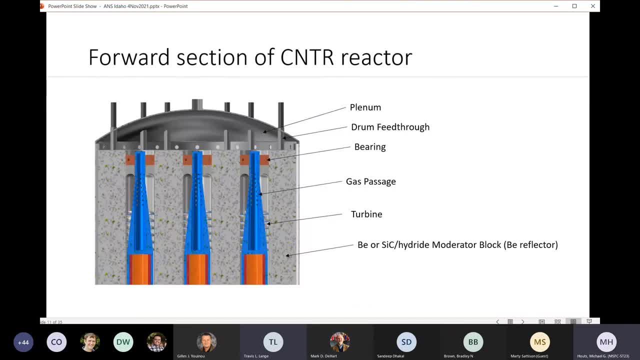 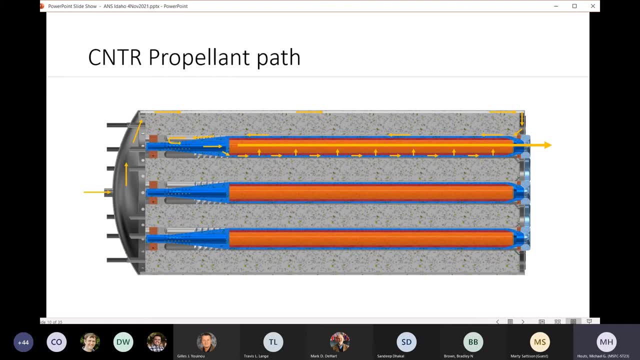 you basically say a cylinder was to just seize up, then, uh, exactly, the um, um, you'd have enough even without the propellant flow. but you'd probably have enough propellant flow still coming through. that that would just exactly. that would just go into the fuel. now you don't have any centrifugal force. 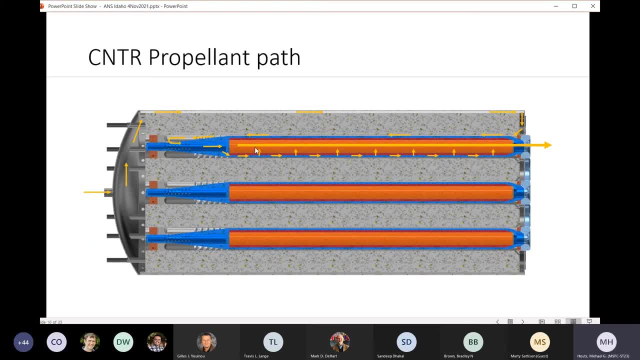 you know nothing holding the uh, metallic uh, uranium- in, and so that fuel is just going to go out the back and so the um, lots of things there, you know. so that would mean we'd probably want to keep our nozzle temperature up high enough that it didn't solidify on the nozzle wall. 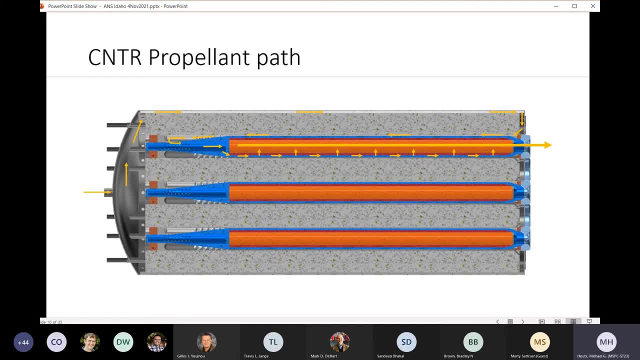 you know you may keep it liquid, so that would eventually, you know, go ahead and leave the system. but the bigger one is, and that goes back to this trade of you know, how many fuel cylinders do we need? uh, can you have a enough control swing on this system that i can lose a whole cylinder worth? 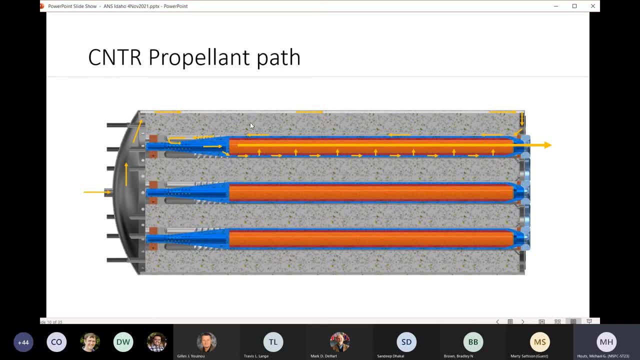 of fuel and still, um, keep, operate, you know, still stay critical, and so that would that would likely drive us to having, you know more, smaller cylinders. so maybe have a- you know 37, you know cylinder smaller diameter. so if you, if one, if one of the rotating cylinders did seize up and you lost, 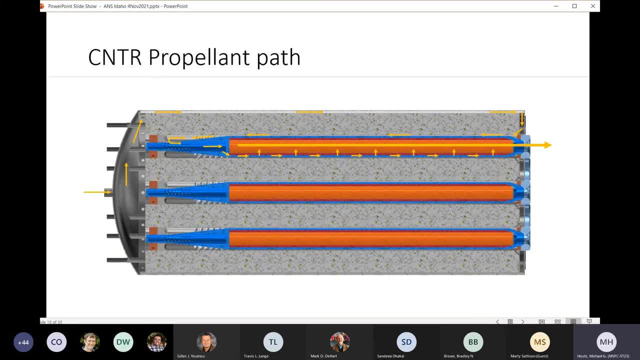 a 37th of your fuel. uh, you could possibly compensate with your control system. so those are all the trades that we need uh need to be done. there's a chance: the uh the naval academy students are gonna be looking at that some. but again, the- i mean students are fantastic to work with, but then 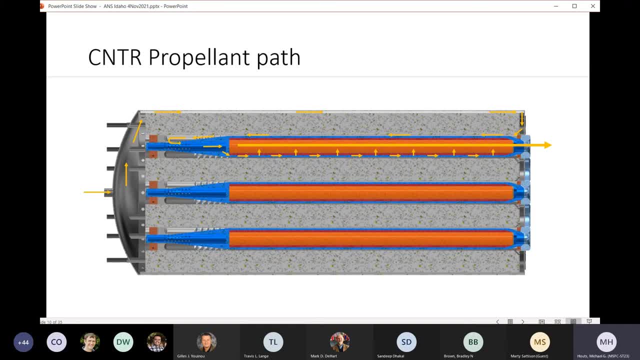 they. then they leave and, as hard as they try to to tell you absolutely everything they did, you know it's a kind of yeah, it does, but anyway, that's why i think one of the things they might be looking at too is the control system. so that's one of the things that we're going to be looking at too is the. 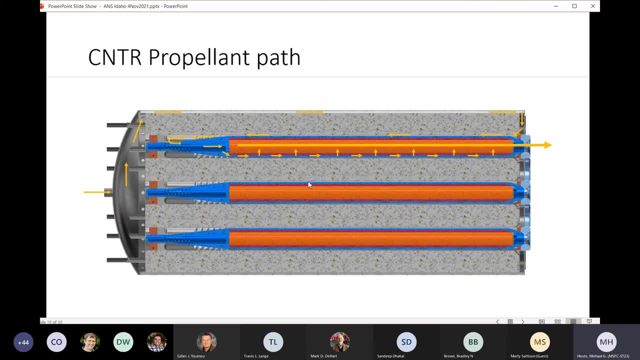 control system. so that's one of the things that we're going to be looking at too- is the control system. um, you know basically how much control we would need on the system. but yeah, that's uh. but yeah, exactly like you said, the uh, basically if that cylinder seizes. 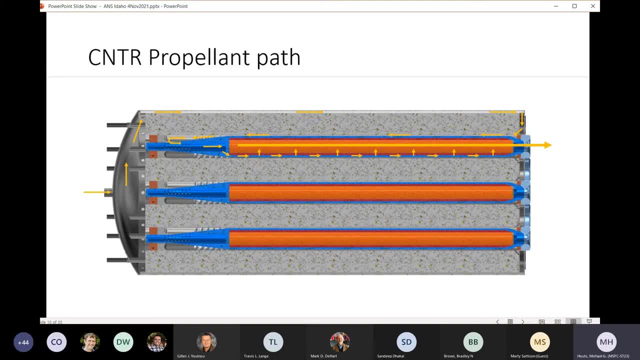 uh, the uranium is going to stay, uh, molten um, and we have to make sure that it doesn't damage, you know, pretty much, the nozzle on the way out. so we, you know, we want to keep that nozzle at 1500k or hotter, just you know, because if it did solidify and then there was more, yeah, i mean so a lot of a. 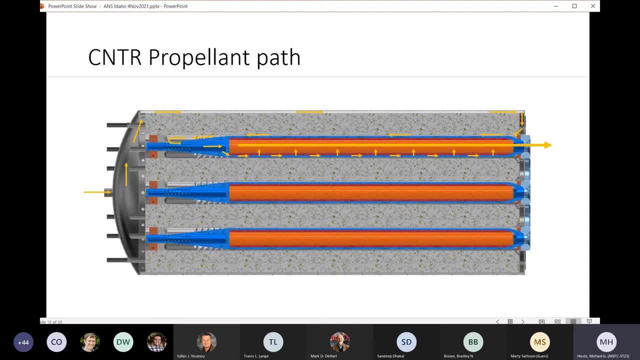 lot, of, a lot of things would come into play. and then, from a nuclear standpoint, yes, how do you, how do you, how do you keep the engine running? uh, how many cylinders can you have lock up before that engine has to shut down? and then at that point, you're relying on just 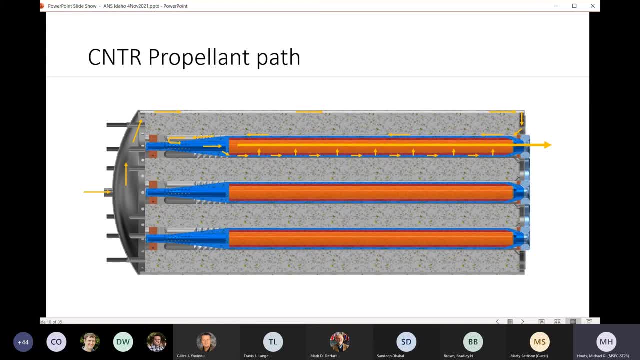 if you had a three engine cluster, you're relying on that. the other two are still running and so, uh, so yeah, huge amount of analysis that have to go into that. so from a kind of a regulatory or, you know, a proof of risk standpoint, you know, how would this compare? obviously you're not. 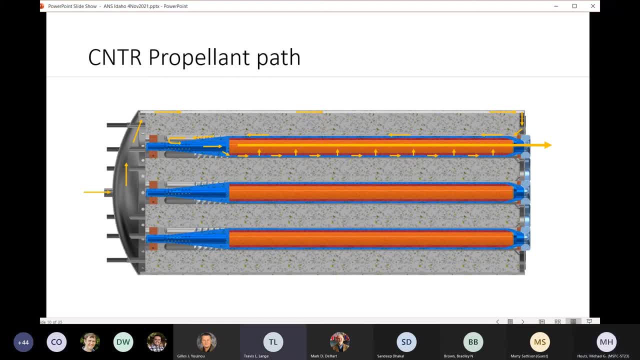 you're not worried about release to the environment, but you know, if you lose enough liquid fuel to the in your, your, your astronauts are stuck in space. so i guess from a- yeah, kind of a risk regulatory, you know, showing that it's going to work, you know, for the next one million years or whatever it is, 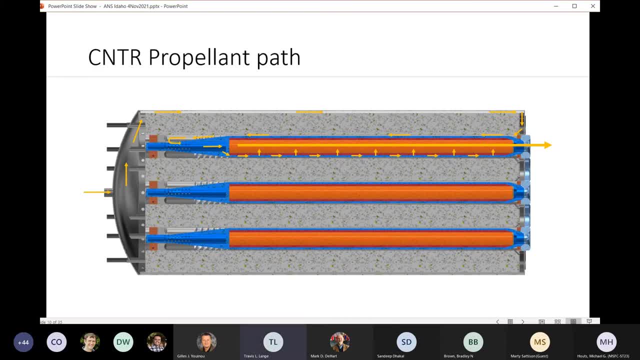 you know, what do you think that's going to look like? yeah, so we'd have to, uh, essentially come down to just the reliability analysis. so, ideally, uh, uh, one of the things people look at is: okay, if you can, you know, say the solid core nuclear rocket, if you can, if you could get home on one. 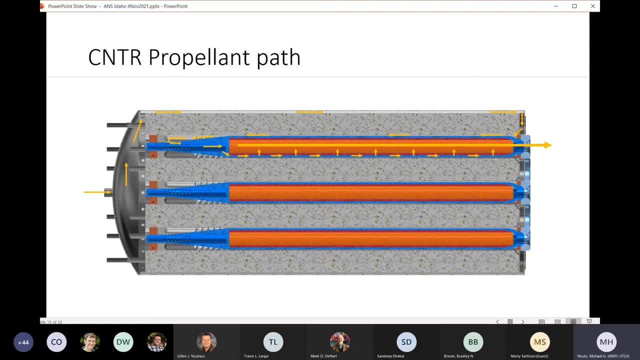 engine and then each engine is 90. i think, okay, i'll probably get these wrong, but you know, correct me if i- but you know- say each engine is 90 percent reliable and you can get the astronauts home on a single engine and you have a three engine cluster and they're truly independent. you know, then i 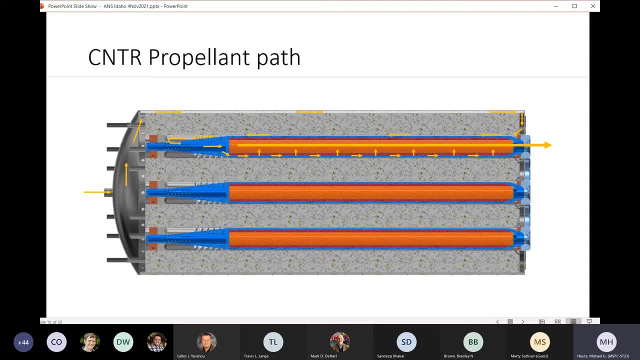 think that's, uh, maybe a one in a thousand chance that, yeah, you won't be able to get the astronauts back home, so that's uh, um, so that would probably be the way they look at. so we would have to show that these engines are. i'm going to go ahead, and i'm going to go ahead, and i'm going to go ahead, and 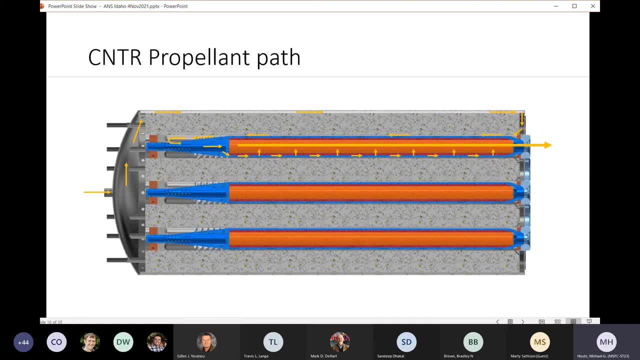 guessing at least each engine we'd have to show that they were going to be at least 90 percent reliable. for the uh it's going to be um. even at the few thousand pound thrust range we should be less than 10 hours total operating time. so that's at least reasonable to try to show. but i think 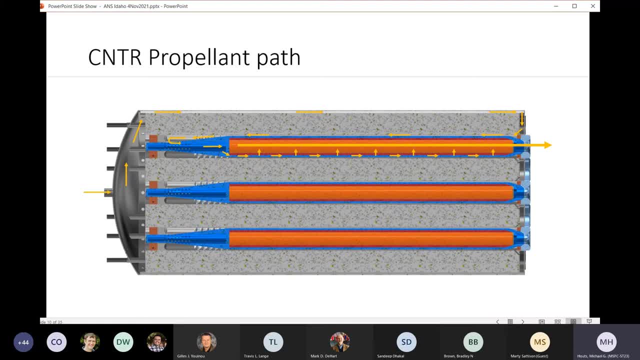 i think each engine- and that's again that's also assuming that that the engines are truly independent on the vehicle and we can get the astronauts home on one engine, uh, three engine cluster i think will need to be at least 90 percent reliable engine. okay, thanks, no, thank you thanks. 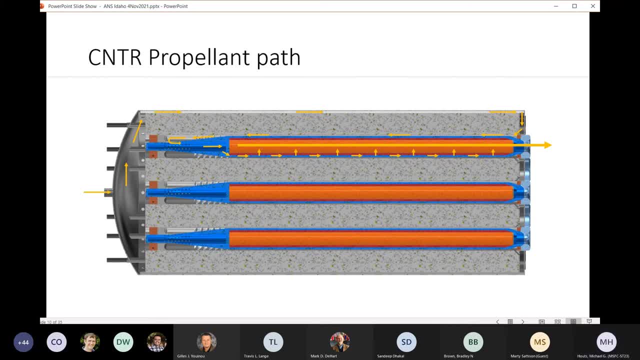 do we have any other questions? you had up to? uh. i apologize for the clock in the background here. you had up to uh. dan thomas has a question. i just disappeared. um, what is the conceptual? let me step back one, because brad brown asked propellant feed pressure, the driving force for getting it to diffuse into the cylinders. 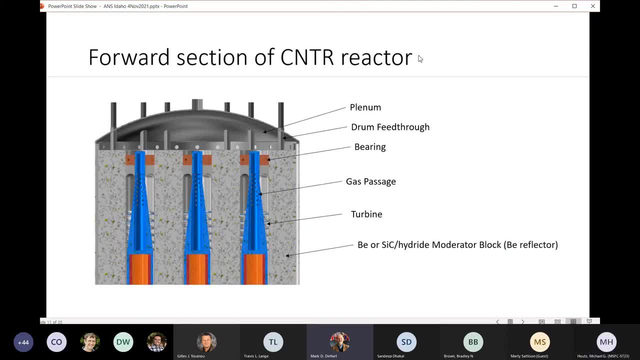 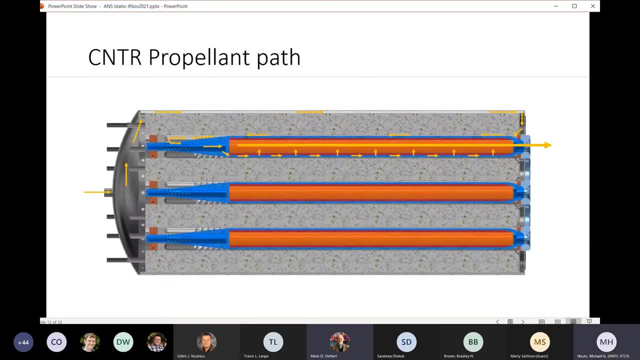 or are there other mechanics at play? so yeah, usually we were, uh, we were just using the pressure, uh, so, um, yeah, so i guess it would be, um, you know, whatever pressure we needed coming out of our turbo pump, and i think we're assuming when it hits the liquid it's at 500 psi, and so if we 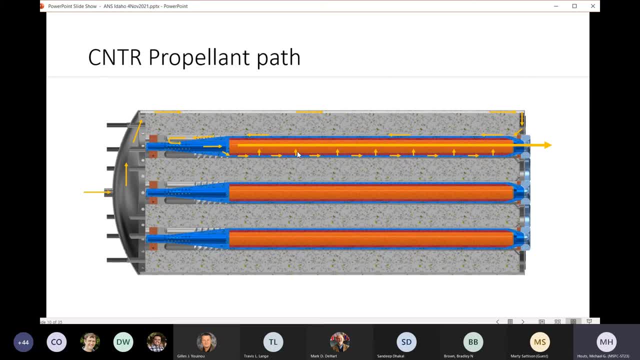 needed. you know, say, if we had a lot of pressure drop in the engine- and that's uh, yeah, that's again, learn a lot from the traditional ntp, the um- if we had a lot of pressure in the um, yeah, a lot of pressure drop, then we, you know, it might be like a thousand psi coming out of the turbo pump. you know. 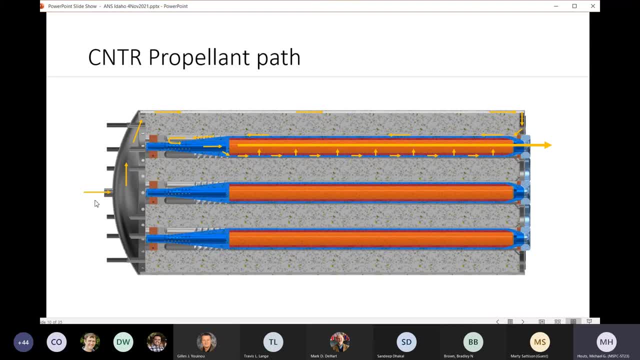 you know, depending on the pressure losses through the engine or more, uh, but yeah, exactly this. when we get to this point here, it's just all. it's just all the propellant pressure. it's the current concept i need to. that's the current notional design and that's one of the reasons i love. 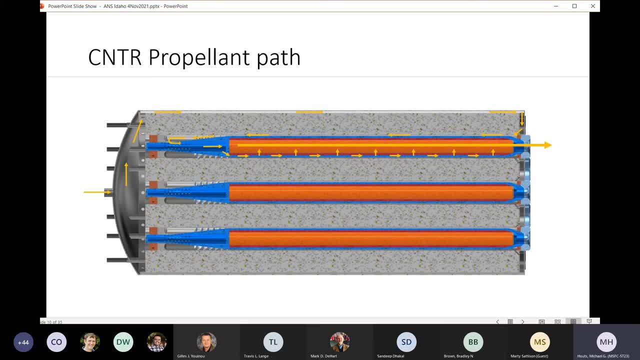 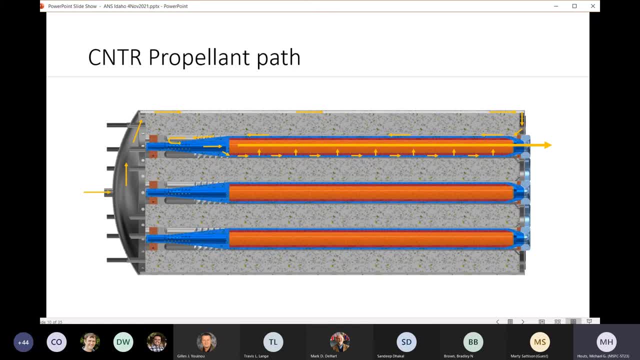 and so that's going to be a very big challenge. but, uh, yeah, um, i think it's a very big challenge too for us to get to that point. yeah, so, um, you know i think we talked about, uh, the more of a, you know, making those suggestions or how to make this more reliable or, you know, easier to. 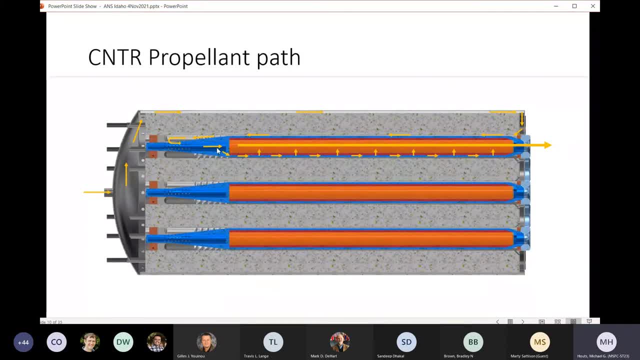 develop, then that way we're 100 open to that, okay, um, dan thomas has a number of questions. what is the? some kind of valving so you can really control your your propellant flow out of the tank? so if we went with that route or if we could passively do it, you know, just off of the turbo pump, then 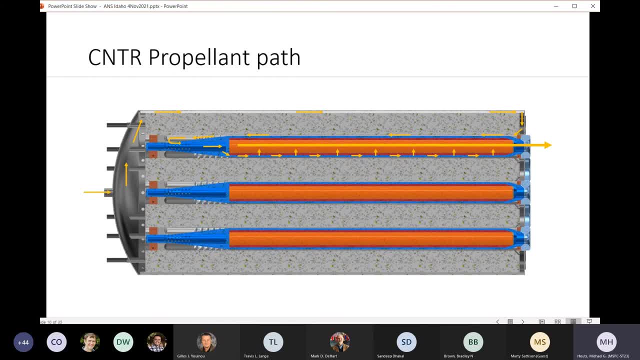 the idea would be: uh, keep the flow going through the fuel, uh, as long as needed. you know, this would just be the decay, heat removal. and then at some point, when that uranium started to solidify, then you'd: uh, you know, then that would be um, uh, at that point you could, either the wall should be. 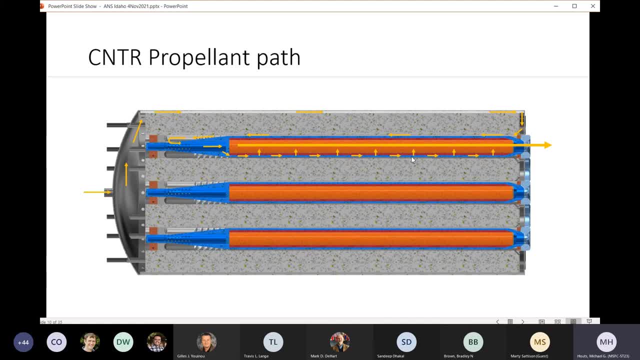 okay, at the 1400 kelvin or less, but if you still needed, uh, some cooling, there's talk about having again going back to the traditional ntp uh loops within the moderator that you could maybe be used for power production or assist in decay heat removal, but that's uh. but yeah, the bottom line. 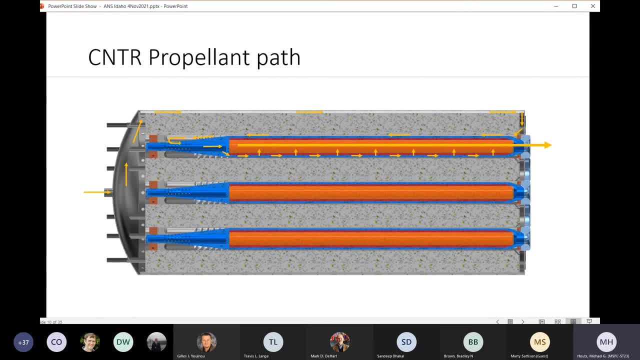 would be: just keep the cylinder spinning, uh, until that uranium metal fuel solidifies. okay, related to that, he asks how much coolant is gonna is it gonna take to come down from the operational temperature to a temperature for your non-fuel components can take? right, so that would be, uh, so. 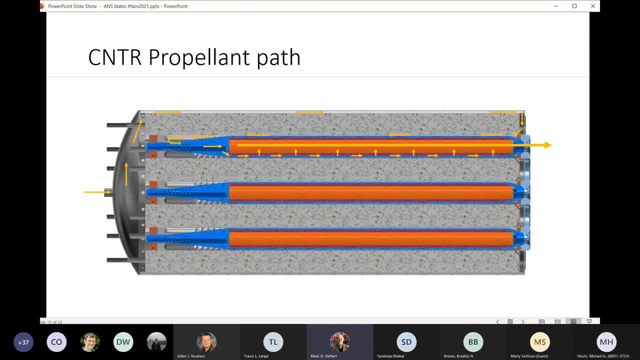 we'd probably go ahead and, um, uh, you know, come you know, as part of the shutdown sequence, we would uh likely uh start shutting down. um, or you know, take, take advantage of the initial cool down. so go ahead and have uh your propellant flowing through that uranium until it got down. 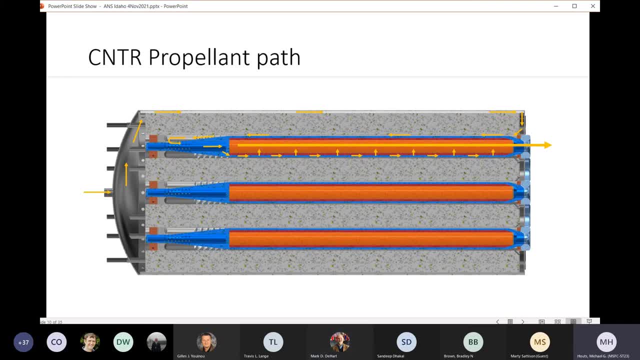 um, you know close to it where it's going to solidify, and then it would just come down to decay, heat removal and so, looking at it from that standpoint, there's actually an incentive to uh, to have the um fission products. you know some, at least you know well. frankly, there's incentive to have all of the 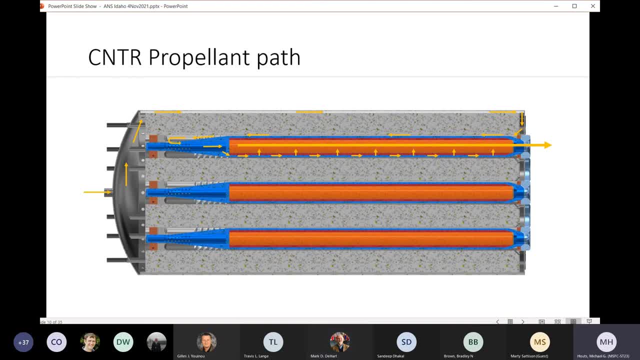 fission products. leave the engine, uh, before, uh, you know, during operation. now we won't get all of them, because there's gonna be some that are, you know, just as high temperatures, uranium, they all. obviously, by definition, they're all lighter than you know they're going to be. you know they're going to be. 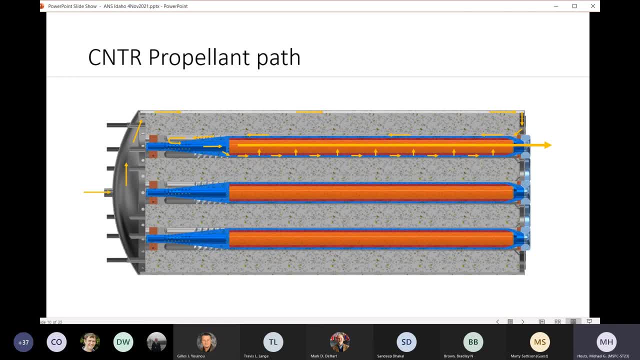 more solid than uranium, but there's still going to be some solidified there. so that's going to be um, uh, yeah, so we're hoping it's less than the amount for a solid core engine. uh, you know, looking at, say, three to five percent of the propellant is used for a cool down. that's where all the fission. 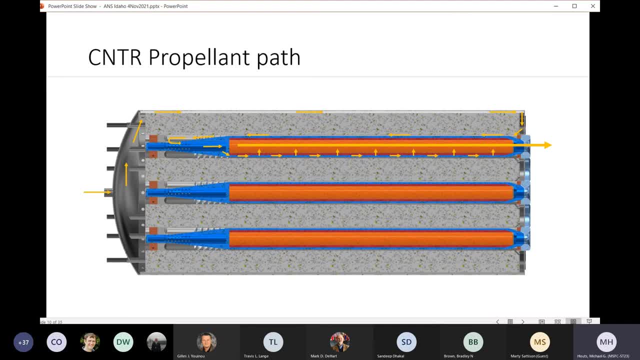 products, you know, basically are still in the fuel and so, and that depends on the plumbing. you know, like, if you, uh, if you want to try to take maximum advantage of your hydrogen propellant or something you know, if we could, you know, ideally we'd like to get that down to, yeah, lower than that, you know. 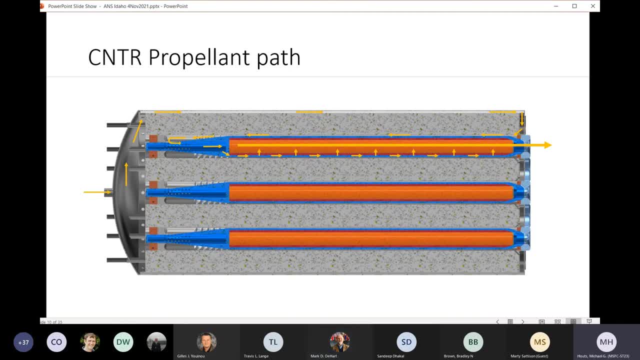 and that's just something we'd have to run some tests and do some calculations on, but there'll be uh, probably at least your rule of thumb. even you know, if a lot of the fission products do exit the system during operation, we're still probably gonna have one percent of our propellant flow uh used up. 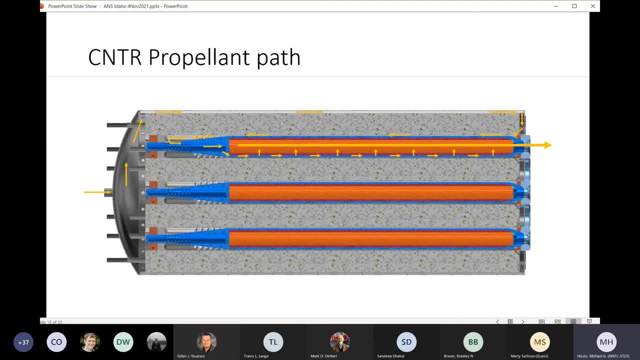 just keep you know, and in that case we would probably have to have some way of bypassing, you know, coolant flowing around this wall. this is solid so it can't, you know, get into the. you know it can't go through the fuel, so it would have to basically just be keeping the wall cool and then maybe bypassing into our exhaust or um. 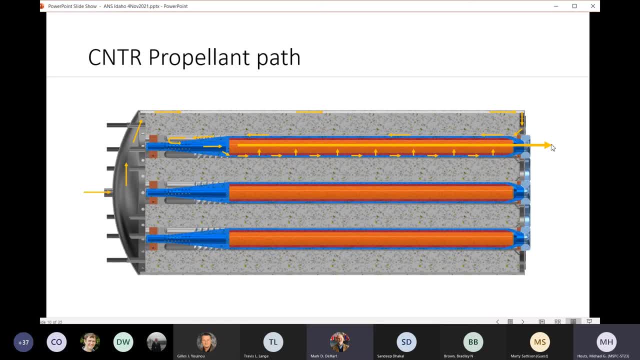 so that's. that's definitely something we haven't optimized or designed yet. okay, um, so with traditional NTP- what traditional? there's no tradition here, but solid fuel NTP. right, they talk burn times of of tens of minutes to an hour. is that about what you'd expect here? 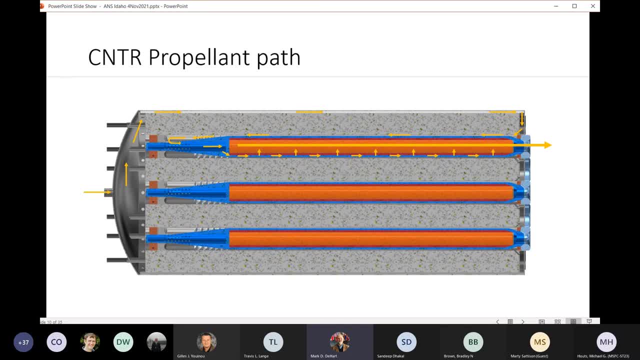 yeah, yeah, we're trying to make sure there's nothing that would keep us from going to 10 hours, uh and then. but that goes back to, uh, you know, jill's question about just what's our thrust per engine. yeah, so if, um, yeah, so if we were, you know, half the thrust of the solid core, then we would um. 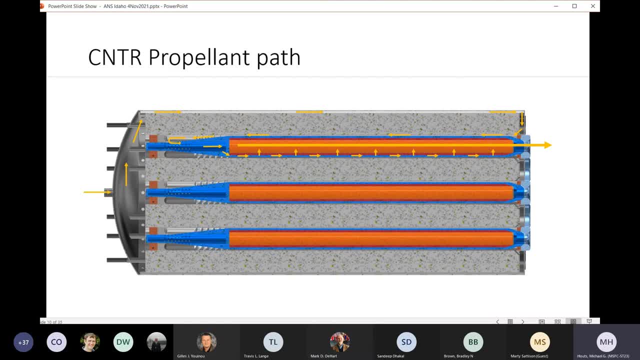 um, yeah, we'd end up needing twice the, you know, twice the burn time. so we're, uh, so, just notionally, we're, making sure there's nothing that would, um, you know, fundamentally keep it from running for, uh, at least 10 hours, or 10 hours. 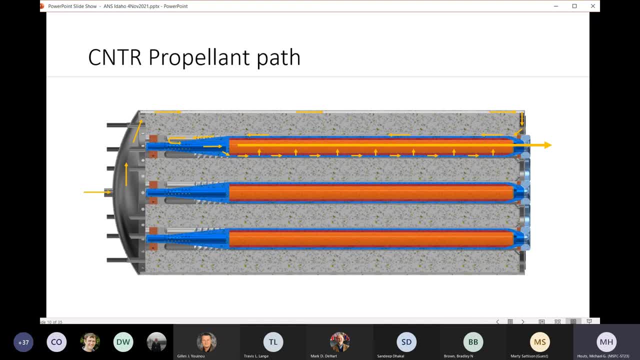 okay, do we have any other questions? i of course, have a ton of questions, but i'm not gonna not applies here. okay, dan asks any benefit for hou or weapons grade plutonium. um, so there, um, you always get, uh, some benefit from either of those. it's um, yeah, but we, we are really getting um, 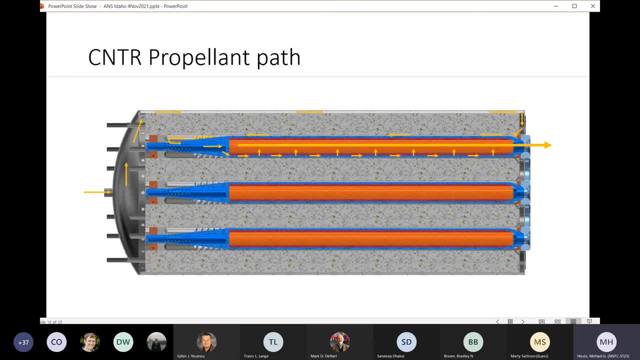 really encouraged to use high assay, low enriched uranium right now, and so that's why so we've designed this around the high assay, low enriched uranium. i think the uh, if we did go to heu, then you could have less, um, you know you, you'd essentially just need less uranium per cylinder. 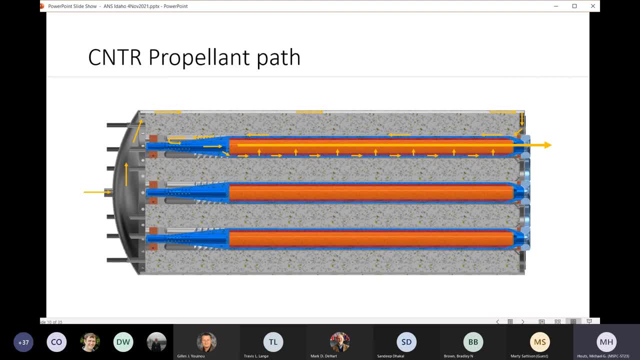 might be one way to think about it, and so you know that that would likely be an advantage. you know, making a the system a little, uh, you know, maybe, uh, you know, the dynamics of the cylinder could get easier. yeah, you wouldn't have as much mass that you were spinning uh, the, uh, yeah, the. 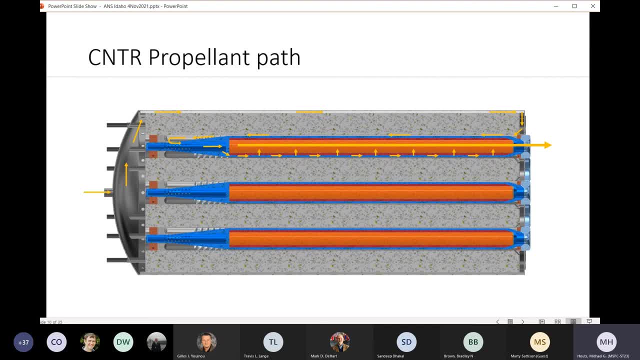 mass isn't, it's not too bad right now. even the- i mean the, the 1500 kilograms is, yeah, that's heavy, but it's, it's not unreasonable and you know we could probably get that again. a lot of the calculations are coming in like 1300 kilograms, but it's uh, but you, so you, but you would save. 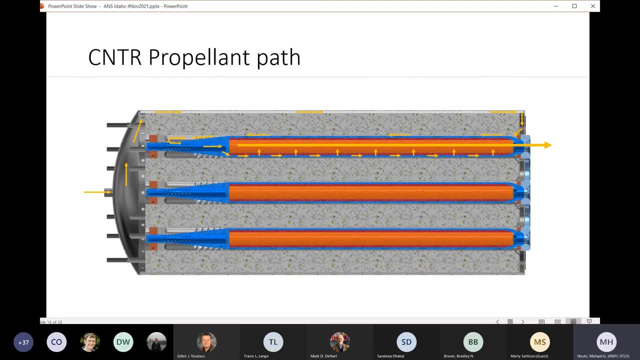 some of the mass, but i think a lot of it. we haven't really looked at it just because we're we're being so encouraged to use the high assay, low enriched uranium, but i guess one of the ones i could see if i- um, yeah, just picture, say i had the same number of cylinders. 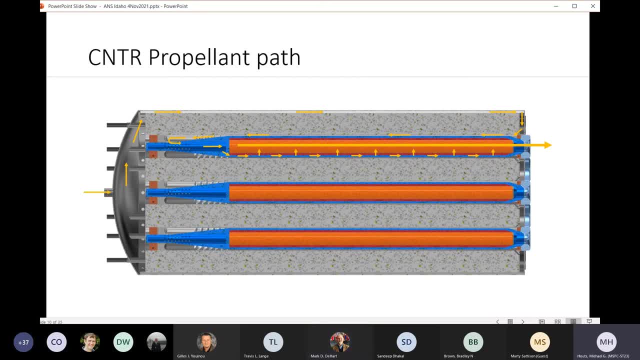 but i only needed a fourth as much uranium metal or fifth as much, whatever that number would end up being in each cylinder. then that that could be a um, just the dynamics of the rotating cylinder. i could see how that could be potentially be an advantage. and then plutonium- yeah, that's an. 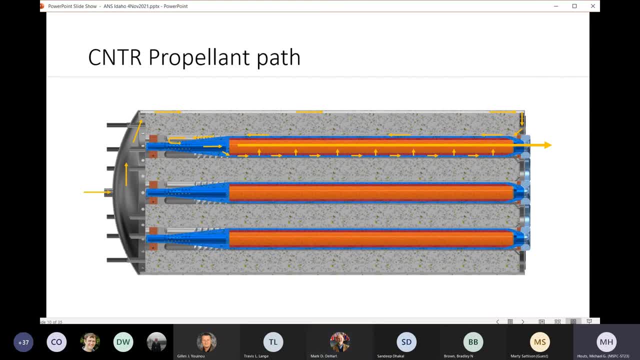 interesting one it's. it's probably really hard to launch. uh, because a big advantage of the uranium-based systems are they're essentially non-radioactive at launch and and the like. the nspm-20- yeah, that came out, um, in 2019. i think it was like august 20th of 2019. 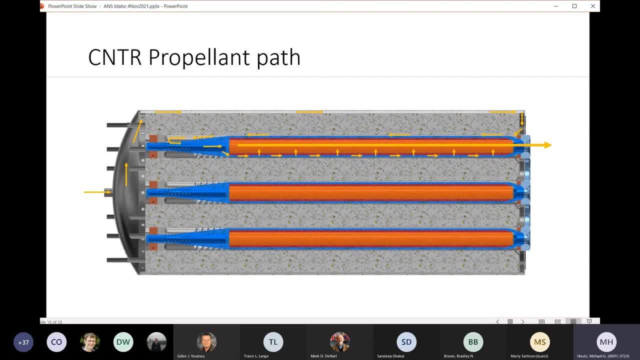 it's just nspm-20. it's a very straightforward for any of the engines we're looking at to meet those criteria. a lot of that comes down to because we have a. i typically have a three mile standoff during a launch, you know, between the members of the public. but even with a half mile standoff, 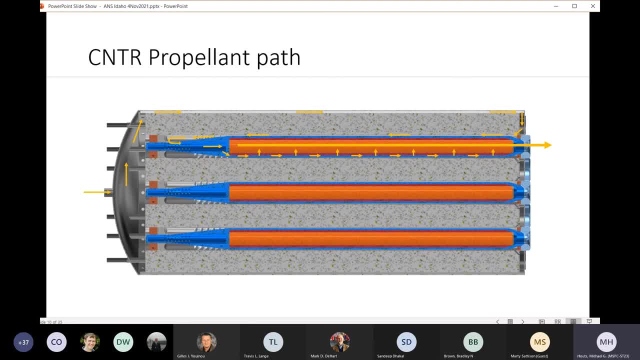